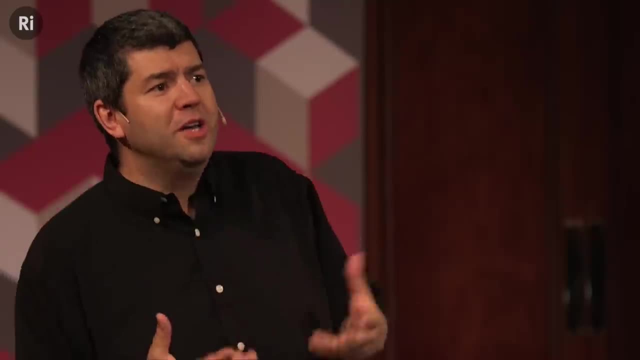 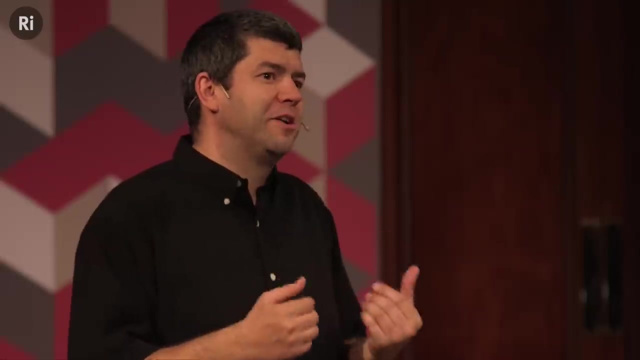 than any other dinosaur and therefore you actually tend to get this kind of weird positive feedback, because it is something that we know an awful lot about As a paleontologist. starting a new study or a new project, you're going to pick an animal that you 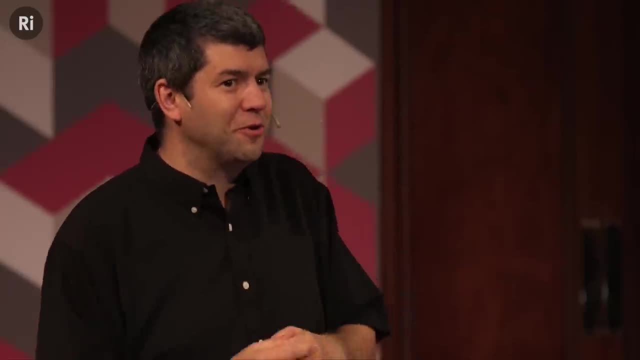 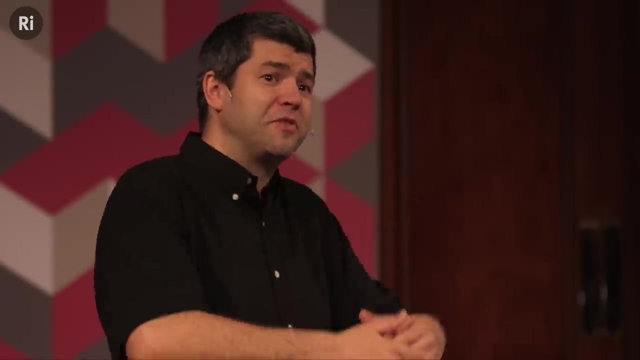 already know a lot about. so people tend to focus on Tyrannosaurus, so they do more work on it. so we learn more about it, so we do more work on it, And so our knowledge about Tyrannosaurus in particular has kind of accelerated away from the other dinosaurs and it's become extraordinarily. 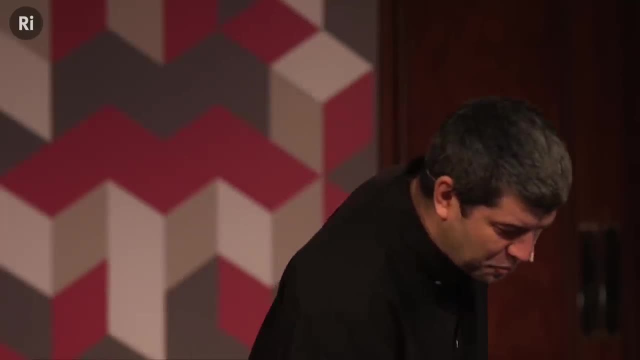 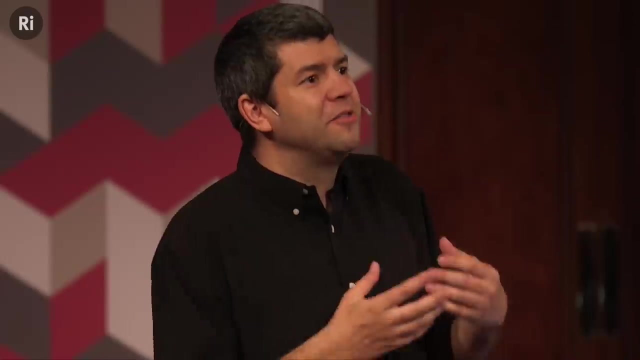 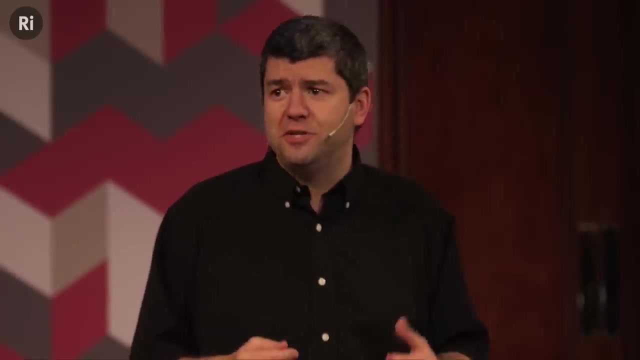 well known and therefore very, very important for us. But what people often don't realise is just how much we have. There's this kind of idea that all our dinosaurs are very fragmentary and things are only known from a few little bones here and there, and that is true for many species of dinosaur. We often have only 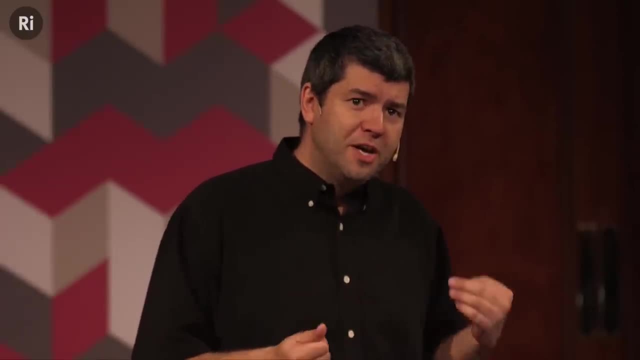 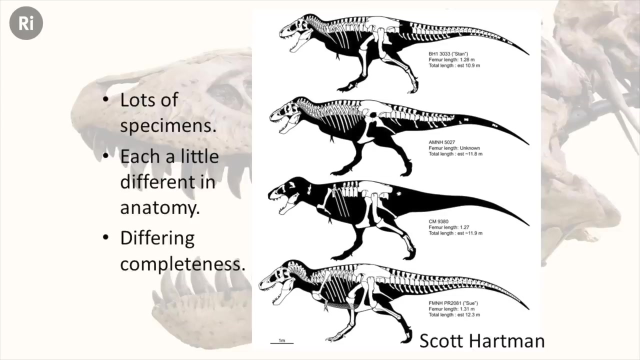 a single specimen. it's very fragmentary. we only have a few bits. But Tyrannosaurus, that's really not true at all. Here are just four that are known, and you can see here that each of them is varying degrees of completeness. some of them have quite a lot missing, some 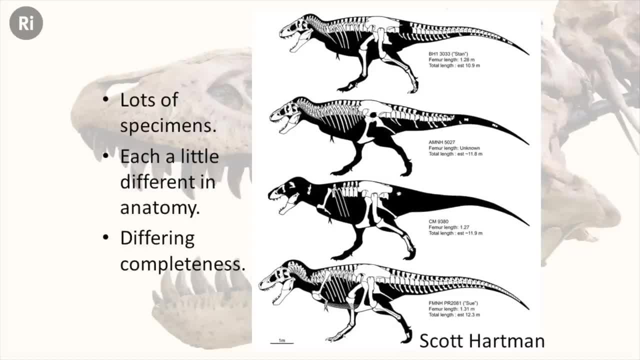 of them are basically complete. The one down at the bottom there is known as Sue, and the other is Sue, which is in Chicago, and Sue is basically complete, As you can see. a bit of the foot's missing, a few other little bits here and there, but we basically have. 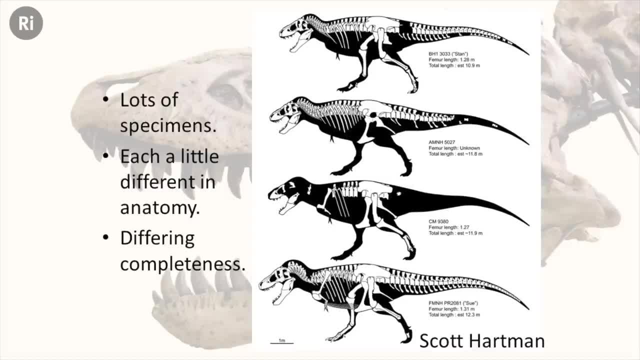 almost every single bone of Sue, And it's also worth noting that they're not all quite the same, Just as not all of us are quite the same. every individual is slightly different. there are subtle differences in the anatomy, the number of teeth, the slight shape of the 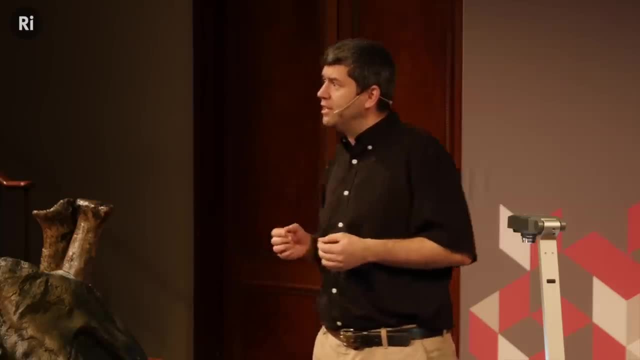 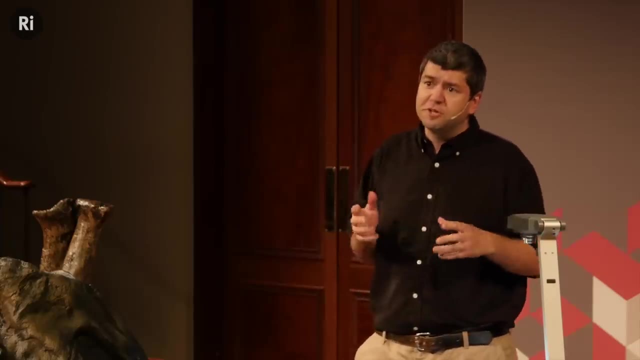 head, the shape of the hands or the pelvis and things like this. So there's really quite a few Tyrannosaurus specimens. There are specimens out there and that helps us learn more about Tyrannosaurus. You can see what the range of variation is. you can see what big ones and little ones are like. 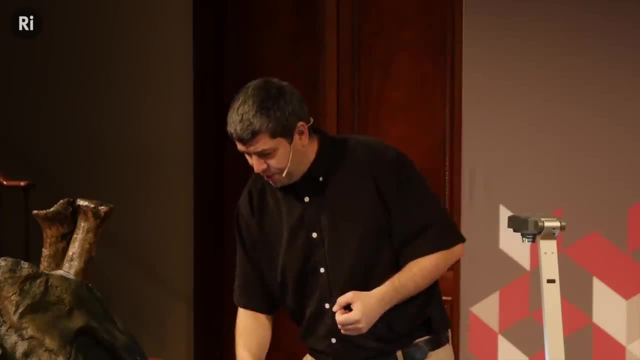 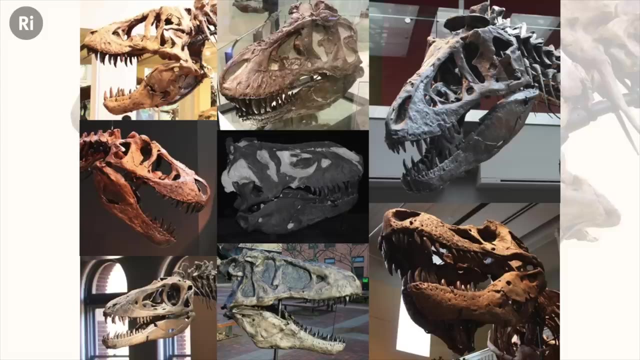 and things like this, But you may be surprised to know just how many we have. So here is just a collection of the skulls that we have of Tyrannosaurus. So here are eight different skulls. Queenie is actually in there in the middle down at the bottom, and these are a. whole bunch of Tyrannosaurus skulls from various different museums, and even this really doesn't cover the diversity we actually have. These are just ones I happen to have photos of. There is about 20 good specimens of Tyrannosaurus, give or take, Ones that are like the previous. 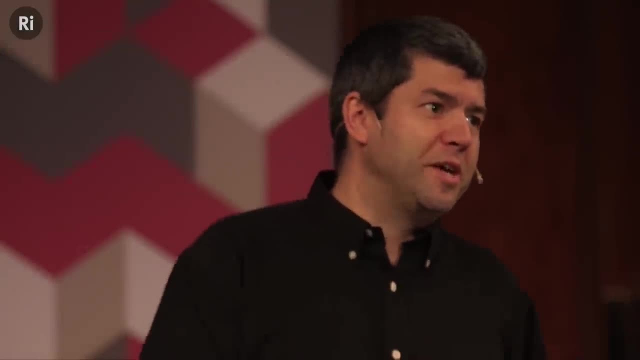 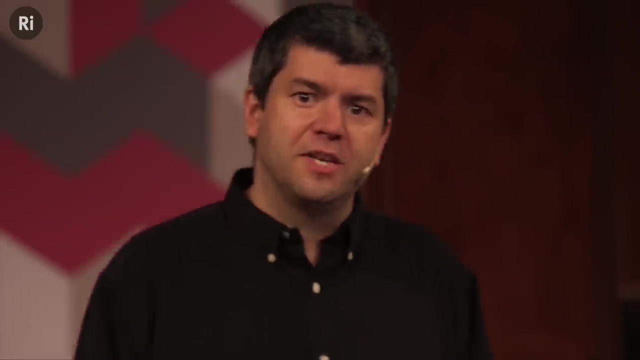 slide I showed. And then, when you start adding up all the other little bits, we've got very fragmentary and incomplete skulls, bits of backbone, single arm, single feet, odd bits of rib and things like this. We have dozens of specimens of Tyrannosaurus. So, while it, 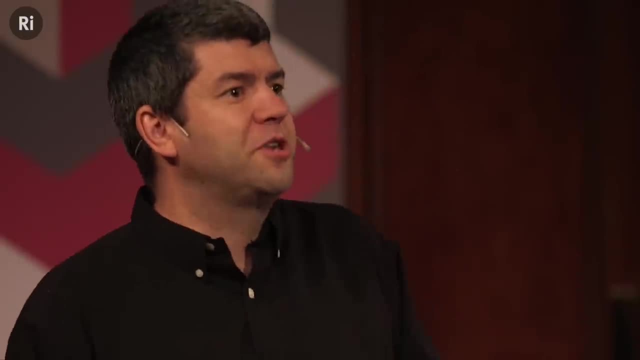 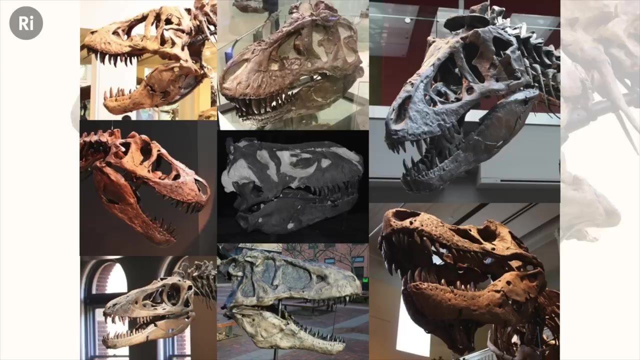 is true that odd dinosaurs are known from very little information. we have to be very careful not to extrapolate a lot. This is one where we have very large numbers of specimens, often preserved in exquisite detail, Though there are some things we need to take care. 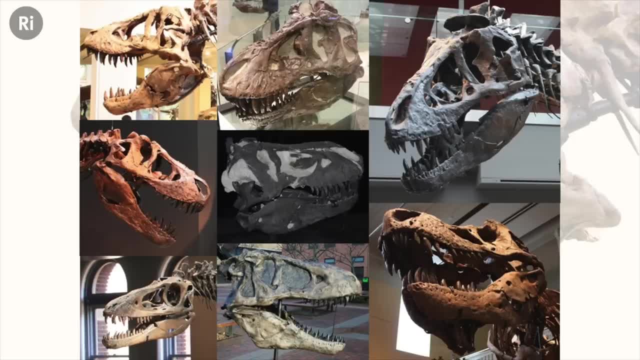 of. One thing that's quite clear, even from this photo, is they're often all different colours. The one in the middle is a specimen in Canada which is called Black Beauty, because the bone is almost black. It's actually a beautiful specimen, but we've got others that 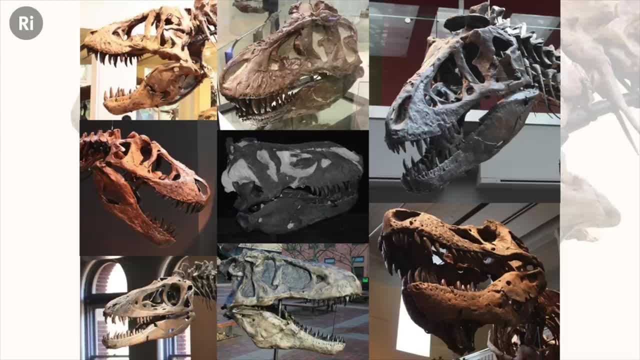 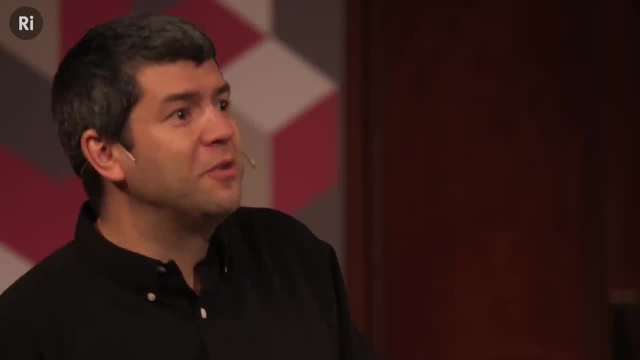 are brown, very, very pale colours, and that's because they're all preserved in slightly different rocks. they all have slightly different histories. They've all been squidged and squished in various different ways at different times. Being underground for 65 million years often does quite a lot of damage to you and you. 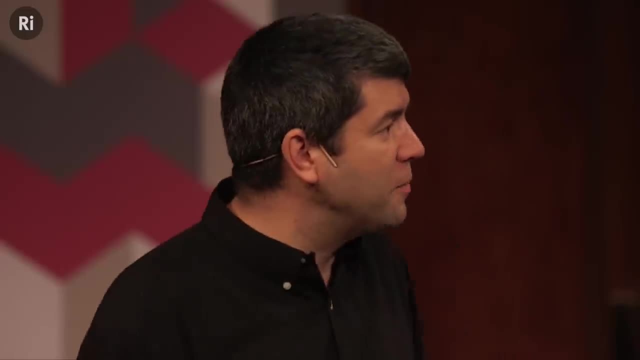 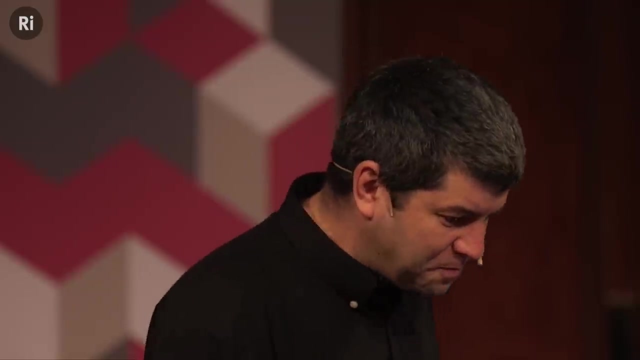 can actually see this in various skeletons and skulls that are up there, And so they're not all quite the same, and we do need to be careful in how we piece together our evidence and build them up. The other thing is: so far, everything I've shown you is basically: 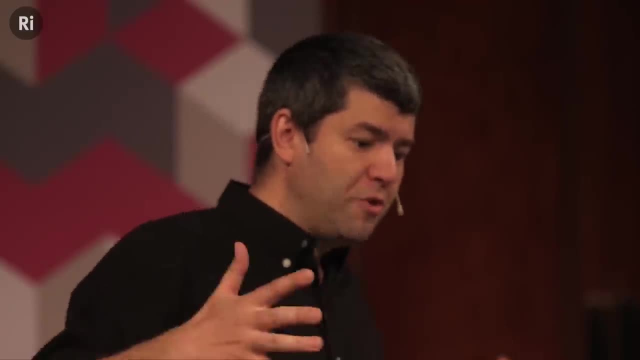 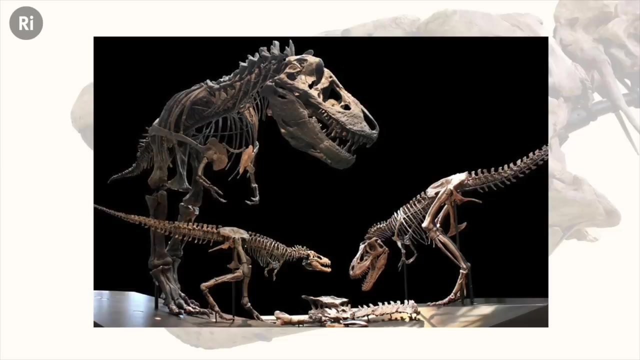 an adult, or at least near enough, But we actually have a range of different sizes of Tyrannosaurus. So these are three specimens that are in Los Angeles, and at the top, at the back, we have basically a full-sized animal, so it would be about the same size as Queenie. 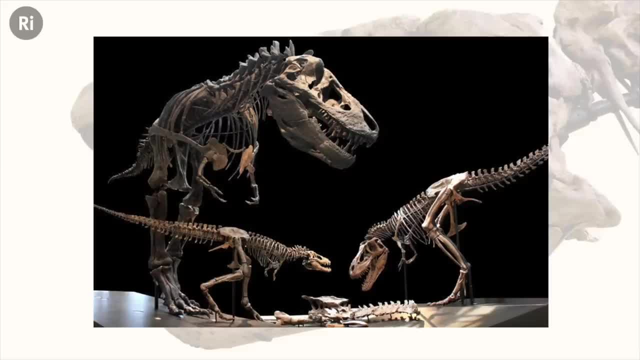 down here so you can see just how big that would be, And then off on the right is a kind of about half-sized animal, at least in terms of length. in terms of weight it would be considerably smaller. And then, down the front again, is a tiny little one known as Chomper. 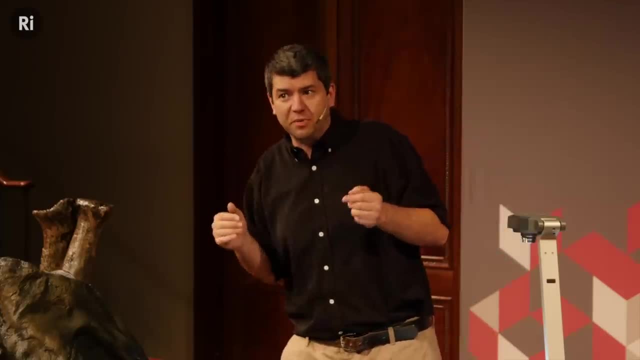 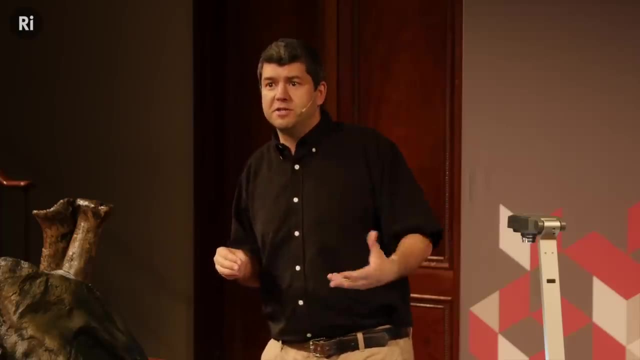 and their head is about this big, 30cm, long, 30cm. maybe It's a very young animal, maybe only a couple of years old, So we have a real range of sizes as well. So it's not just that we have this whole big pool of giant bone-crushing. 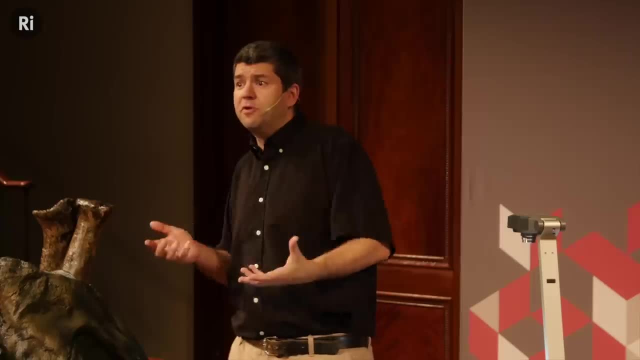 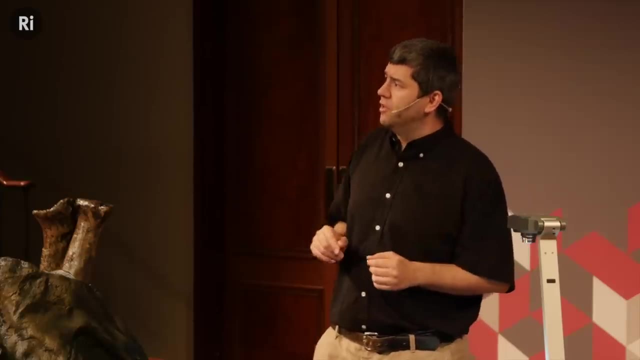 monsters. although we have plenty of them, we do actually have the equivalent of teenagers and even very young children, though sadly, to date, we have no eggs and no embryos. We do have lots of eggs for dinosaurs and even a few unborn embryos of various ones, but 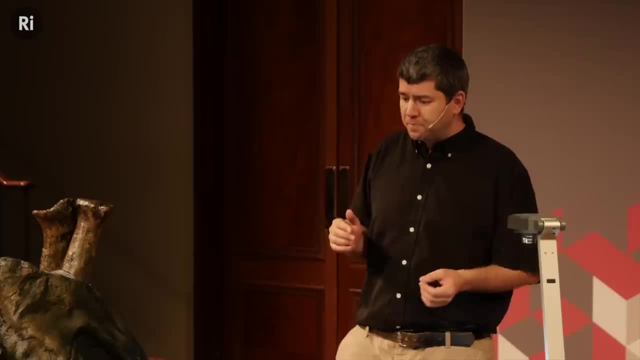 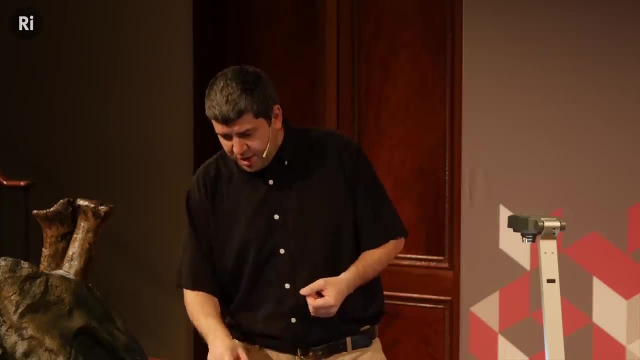 not one for Tyrannosaurus, or indeed any of the Tyrannosaurus, And any of the Tyrannosaurus is a really key point because, again, everyone has heard of Tyrannosaurus, Everyone knows that name. It is one of about 30 species of Tyrannosaur. 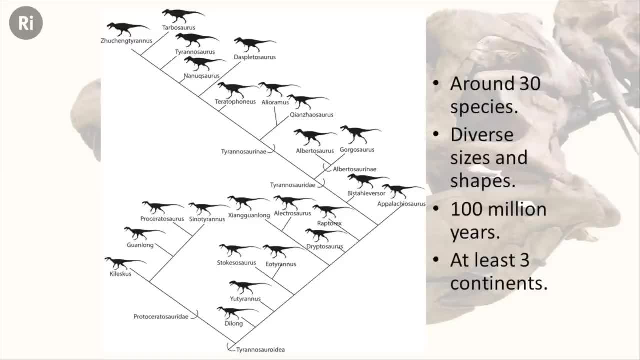 This is a big, diverse group of animals. It is not just one species- T rex- it is in fact a whole group, or what we'd call a clade, so an evolutionary group of animals And, as we can see from here- hopefully you can see quite a diverse sense of size and shape. These 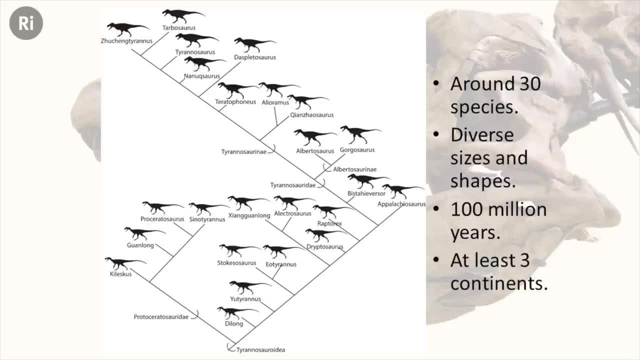 little silhouettes are not done to scale And this is the complete family tree of them. so far, I say there's about 30 species, because we don't actually know quite how many there are. And there's a couple of reasons for this. First of all, paleontologists actually disagree. 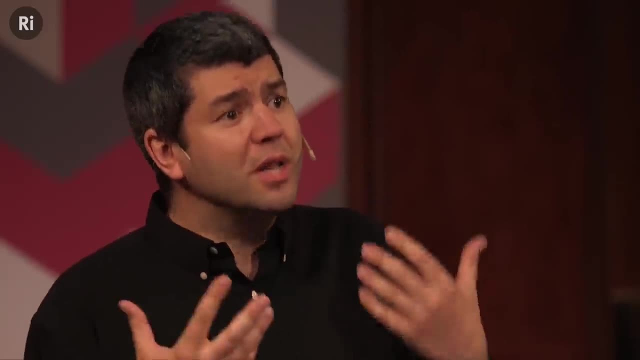 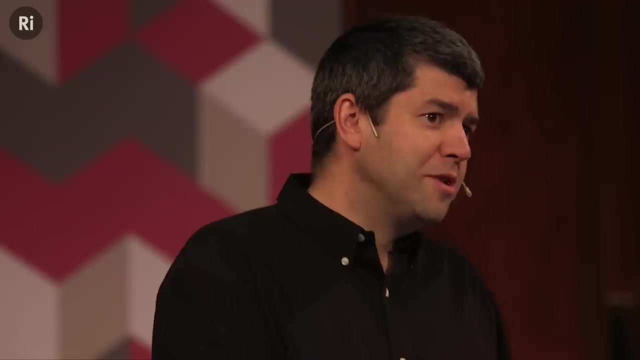 on quite how you tell species apart. This is a problem that plagues modern biologists: Two things that look very, very similar to each other. it can be very hard to say if they're one species or not. They might have very similar genetics but quite different. 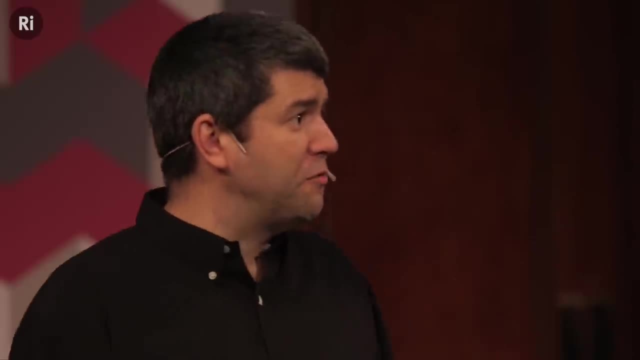 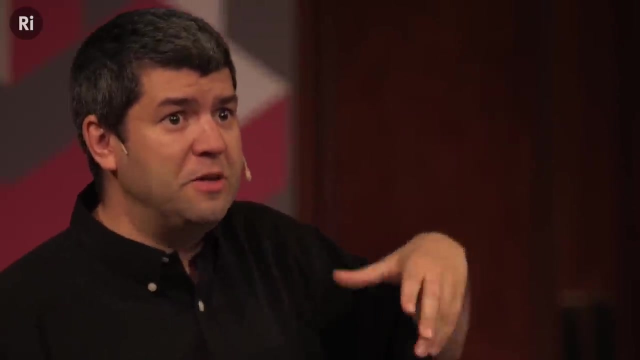 DNA or very different appearances and live in different countries, but then their genes are almost the same. We are looking back to at least 65 million years, with most of the bits missing. It's therefore inevitably very, very hard to say sometimes when you have two. 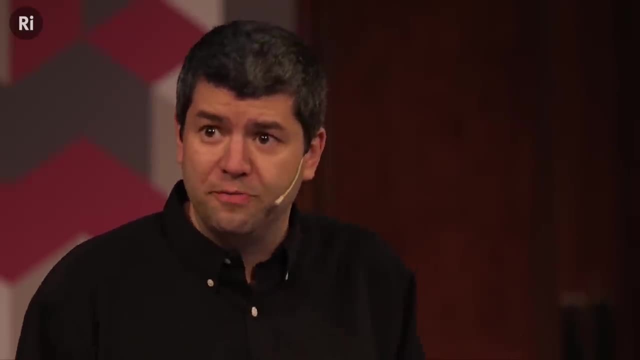 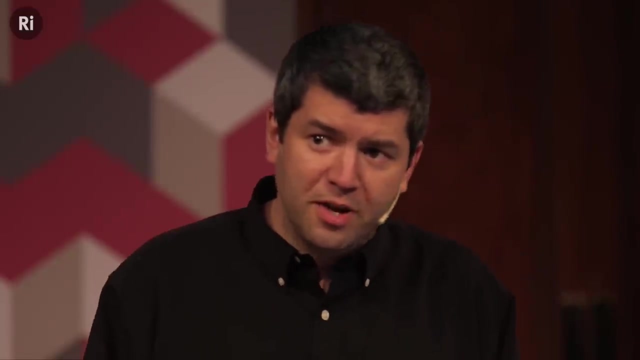 very incomplete skeletons. if this is one species or two, Or if you have only a small group of very nice specimens, maybe there's two species in there, but we're not quite sure. So I say about 30, because that's a number that 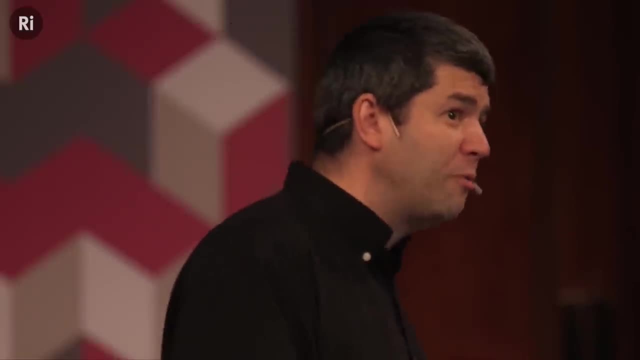 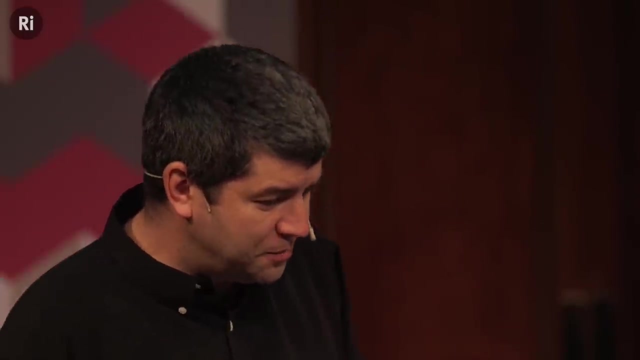 probably everyone agrees on, But there could easily be one or two more and we don't realise yet, or one or two fewer and we need to revise some of our estimates, But it's certainly really quite a diverse group. Not only that, but Tyrannosaurs really got around, Tyrannosaurus. 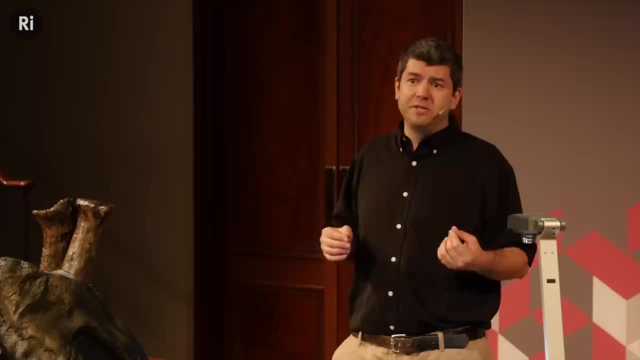 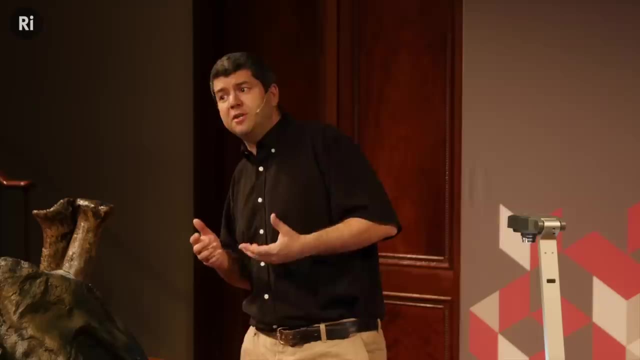 itself lived in North America. We have lots of specimens from Canada, particularly in Alberta, and the US, particularly in Montana. But it was wider ranging than this. There's a whole bunch of bits down in central Mexico which may or may not. 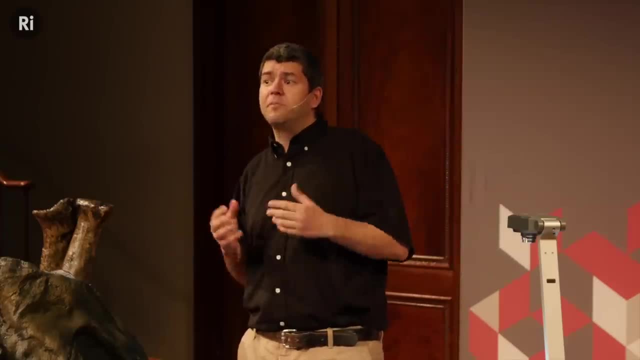 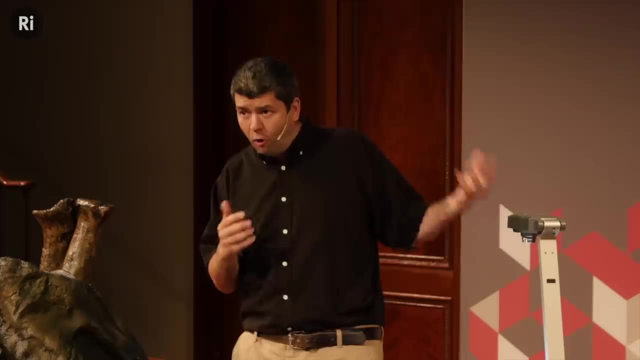 be Tyrannosaurus. They're very fragmentary, but certainly about the right time, and it would not be a big surprise if T rex had a really big range across the whole of North America. There's a whole bunch of Tyrannosaurs that lived in North America. It's not just. 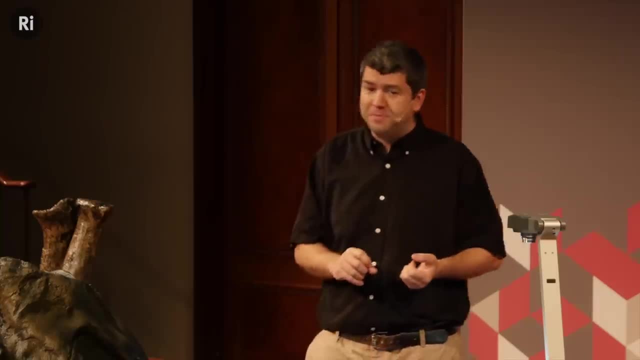 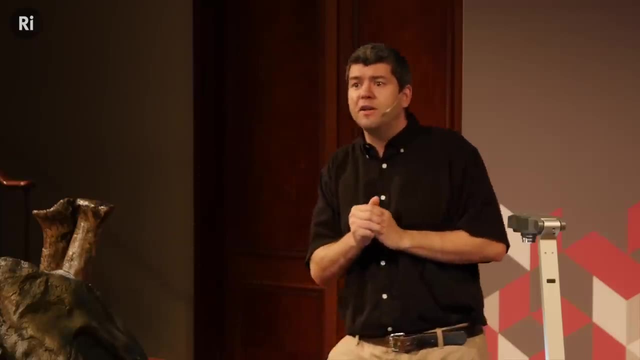 this guy. We have things like Albertosaurus from Alberta and Gorgosaurus and Daspletosaurus and a whole bunch of others. We have a whole load from Asia. There's things like Tarbosaurus, Juchang, Tyrannosaurus, Aelioramus and many, many more. 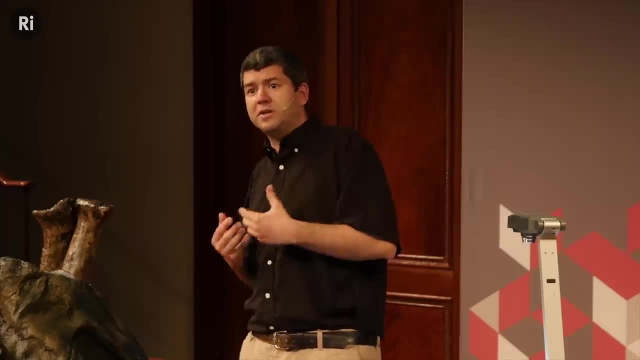 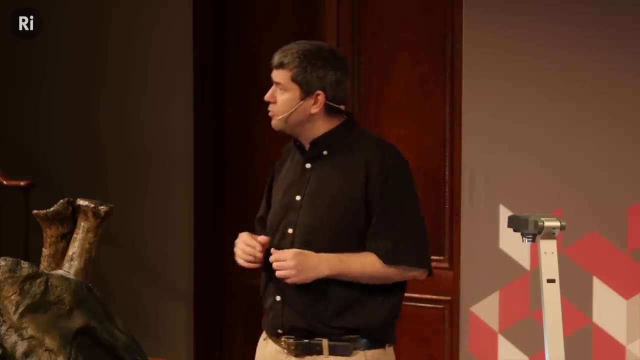 And then, going right back to the early days of Tyrannosaurs, we have things like Guanlong and Deelong. What may surprise some of you to learn is we actually have two different species which are known from the UK. They have a little thing called Proceratosaurus. 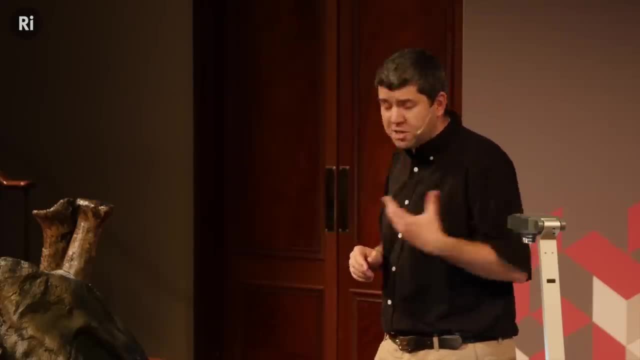 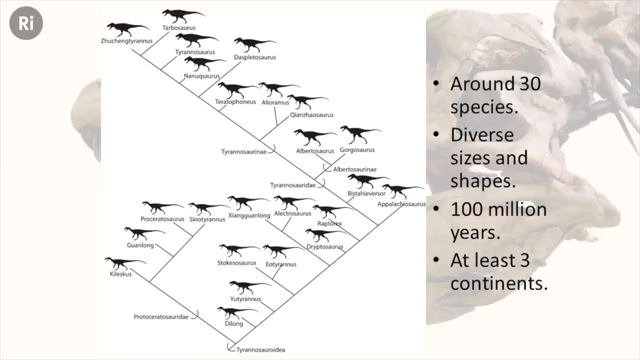 and another one from the Isle of Wight called Eotyrannus And actually Proceratosaurus, is one of the earliest of the Tyrannosaurs. So it actually sits here on this little branch which is actually called the Proceratosauridae. So it's an own little branch, a very early. 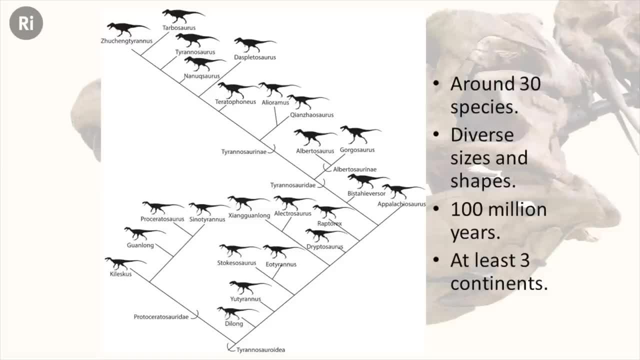 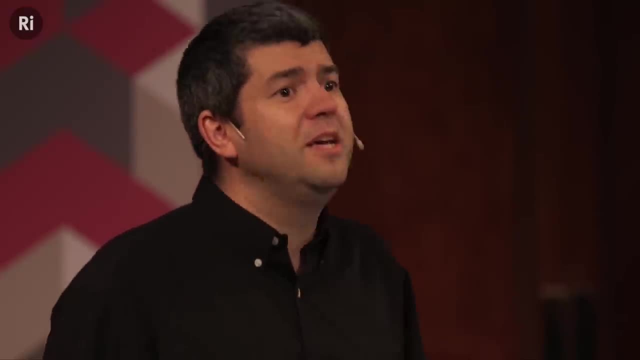 branch of Tyrannosaurs that came off the Earth And diversified into a small little group. And these are unique because they all actually have little crests on their head, which we'll see better in the next slide. But the emphasis I want to make here is just how many Tyrannosaurs there are. It's not just T rex, This is 100. million years' worth of dinosaurian evolution. The earliest Tyrannosaurs that we have lived about 165 million years ago, And the last of them, including things like T rex, died with the great mass extinction at the end of the Cretaceous period. Died around 65 million years ago. So conveniently in one way, the Tyrannosaurs were around for almost exactly 100 million years. So that's a nice easy figure And we have them on at least three continents. There are suggestions of one. in Australia There's a very fragmentary. 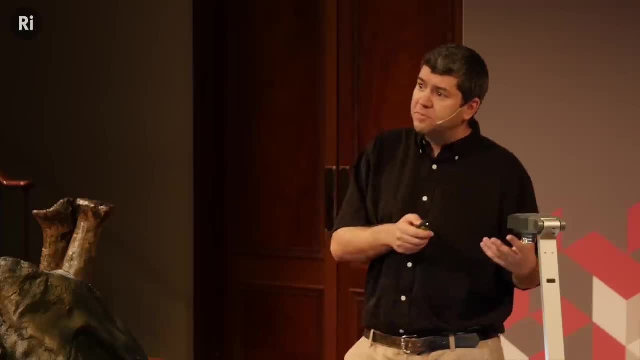 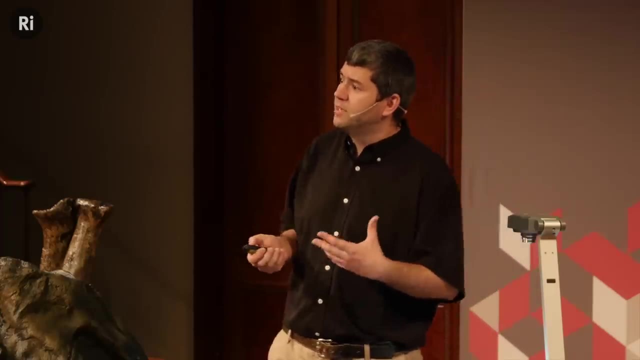 bit of a pelvic bone in Australia, And there are some animals in South America which some people think may be an odd branch of the Tyrannosaurs, And if so, in both of these cases, then we have them on at least five continents. 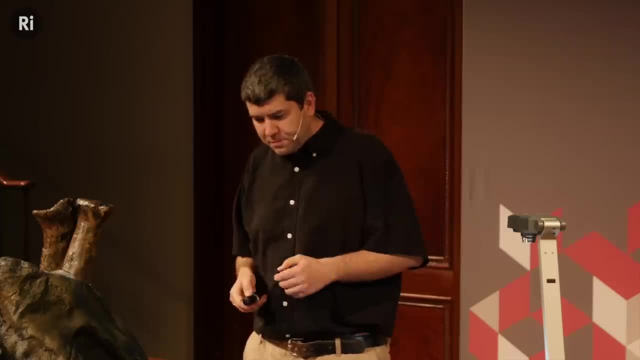 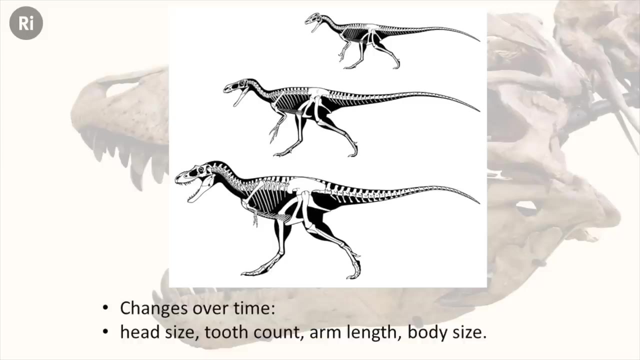 And they were basically worldwide. If we look at them in a bit more detail, we start to see some differences crop up. None of these pictures are quite to scale, but certainly the one at the bottom is much bigger than the one at the top. So the top animal here. 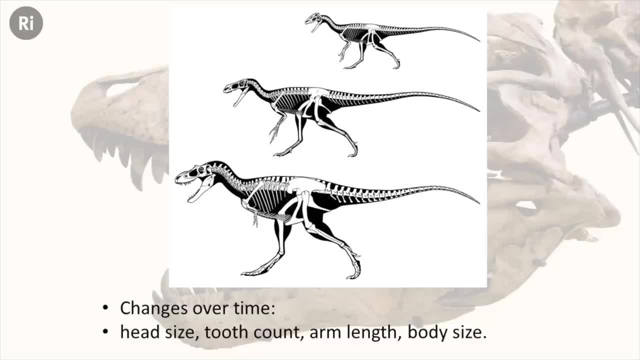 is a thing called Guanlong from China, And that name means crested dragon And, as you can see, there's actually this big expanse of bone along the top of the skull. It has this little bony crest which sticks up, And we think this was probably some kind of signalling. 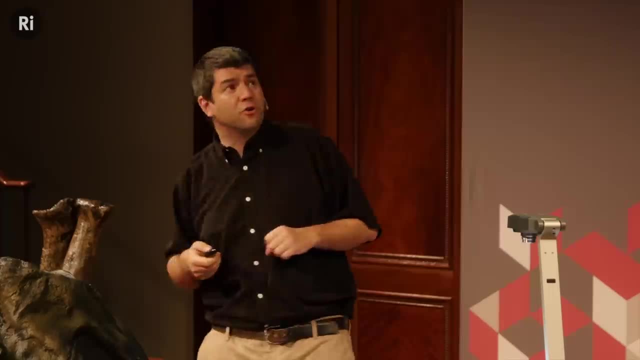 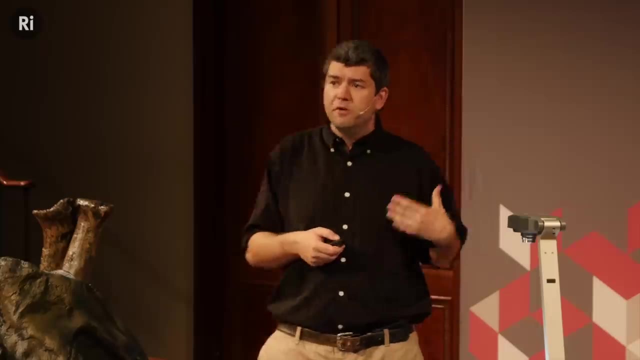 of something that was going on in the past. So something basically to show off and say how big and strong you were. And we can see there's some major transitions that happen with the Tyrannosaurs. If we look back 100 million years we see these animals are really 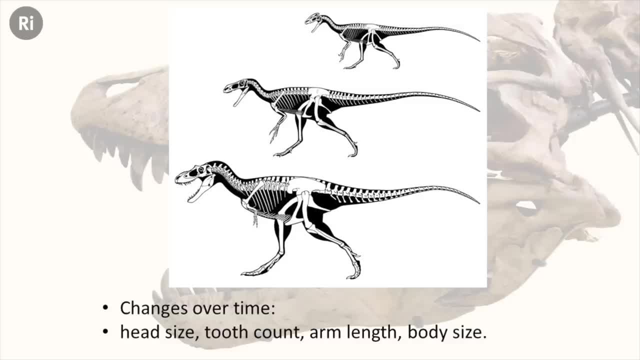 quite small. Guanlong is a very small animal, maybe about two and a half three metres in total And about half of that is tail. So you're not talking about a very large animal. If we look a bit further down, we see that there's a pattern starting to happen. The 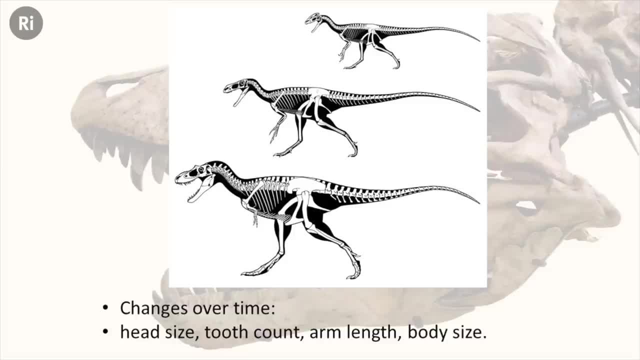 arms are getting a little bit smaller. T rex famously has these tiny, tiny arms, But if we look back to its earliest ancestors, they have great, big, long arms and tiny little heads and a little neck. This is not what we think of when we think of Tyrannosaurs. 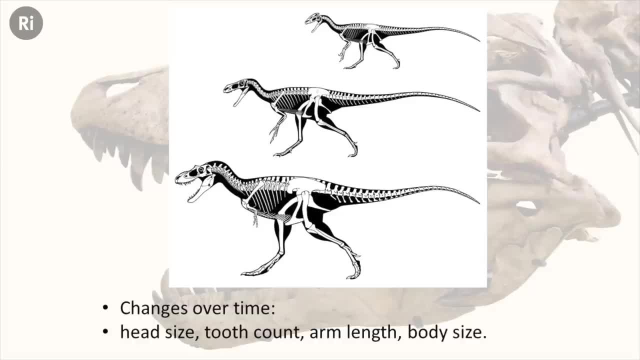 But actually, if we look over time we see there's these fairly obvious patterns of, as we go through: a small head becomes proportionally bigger and proportionally bigger. That long, thin neck becomes shorter and stronger. The body becomes generally smaller. The body becomes. 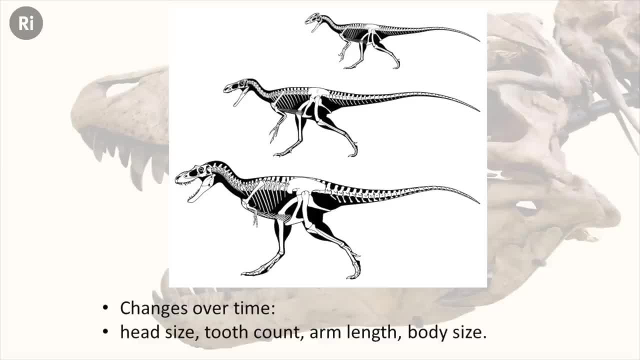 deeper and more robust. The arms change from these great big, long arms with great big long claws and the end and three fingers down to a shorter and shorter arm and then reduce finally to two fingers And at the same time the body is becoming proportionally big And 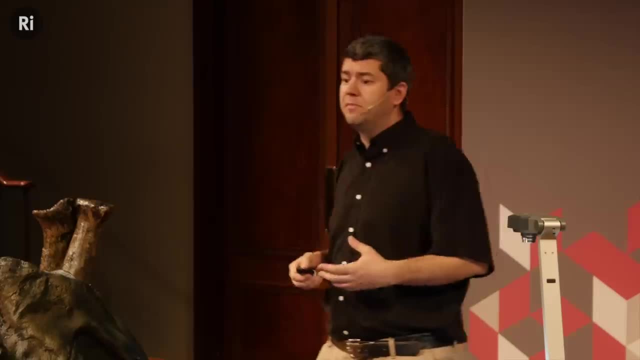 as well, though you can't see it on this figure, the teeth are reducing in number. Tyrannosaurus and its nearest relatives, things like Tarbosaurus from Asia, basically have a very large body And, as well though you can't see it on this figure, the teeth are reducing in number. 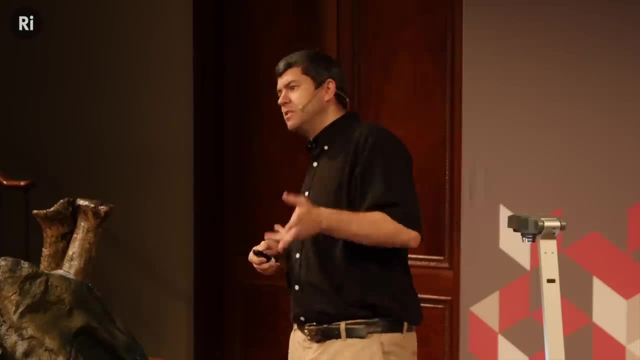 Tyrannosaurus and its nearest relatives, things like Tarbosaurus from Asia, basically have a very large body. Tyrannosaurus and its nearest relatives, things like Tarbosaurus from Asia, basically have about 60 teeth. Things like Deelong and Guanlong- some of the earliest. 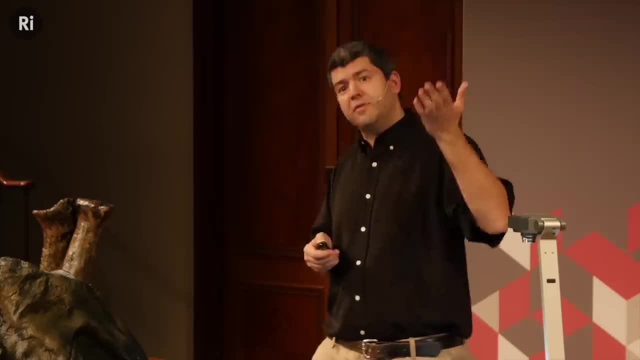 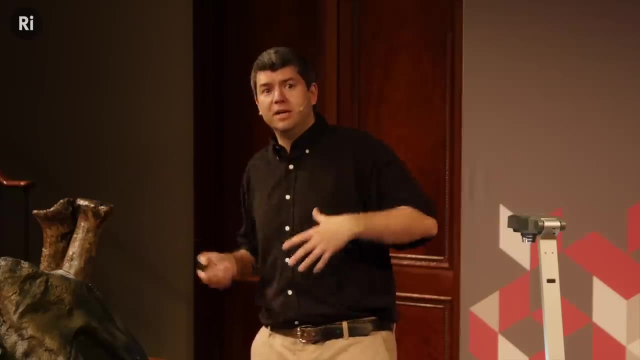 Tyrannosaurs have closer to 100. So they're slowly cutting down the number of teeth. they're getting bigger heads, shorter necks, a bigger body, shorter arms and overall they're getting bigger and bigger and bigger. And so this is what happens when you put together 100. 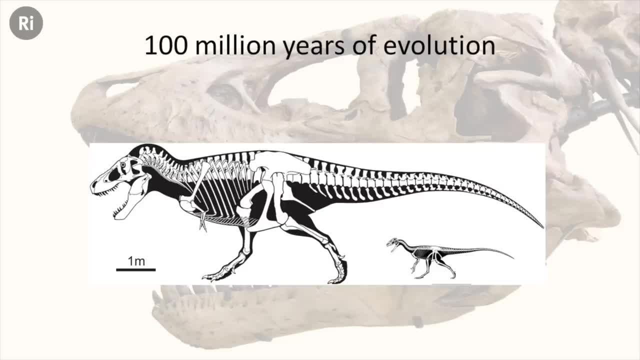 million years of evolution. So here we have Guanlong again with his little crest knocking around at about three meters long, and here we have Sue, to the same scale which is in Chicago. Sue is probably about 12,, 12.5 metres long. 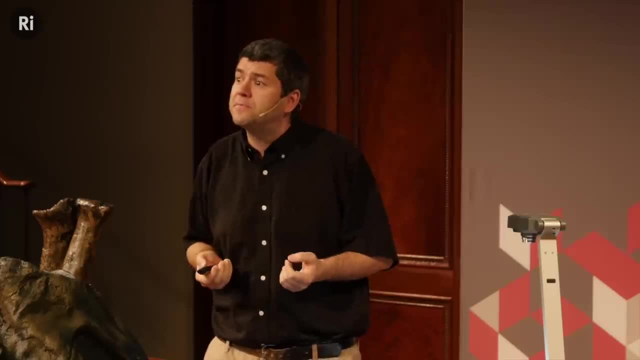 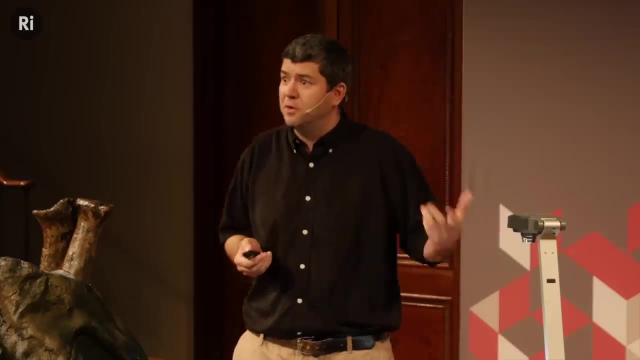 and weighed right around 7,, 8 tonnes. So that's about two big elephants put together, maybe three or four family cars in weight. and this is still a biped with a head every bit the size of Queenie here, And I can assure you because I've measured this. 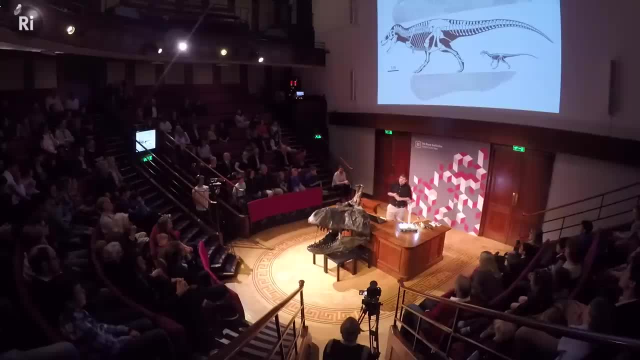 I actually fit through the mouth. So everyone who's seen Jurassic Park, if you want to know if you can eat a lawyer, yes, they can, and into a single bite too, You fit. These things are absolutely enormous, But this is the change we've seen over 100 million years. 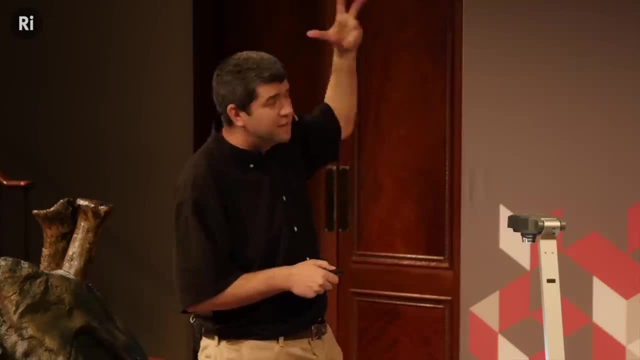 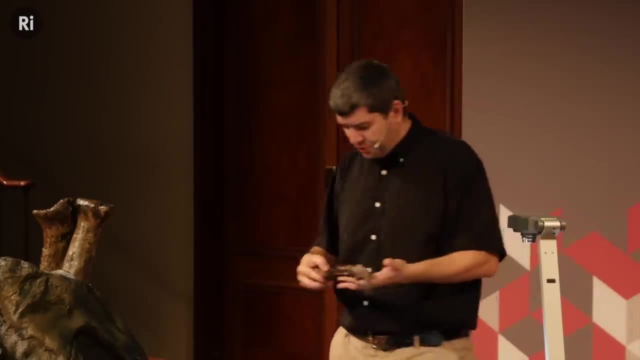 We've got massively, massively bigger in size. The head's shrunk, the neck's shrunk, the body's got bigger and the arms are absolutely tiny. Just for comparison, this is most of the forearm and hand of Albertosaurus. 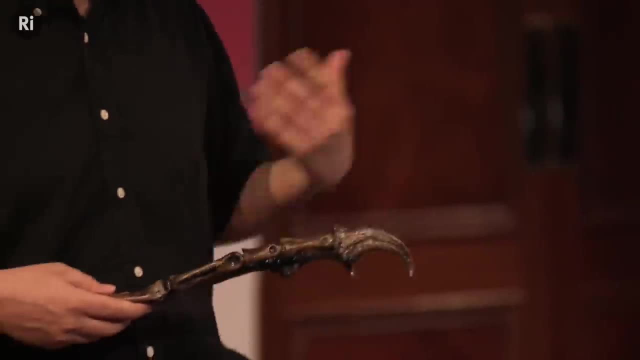 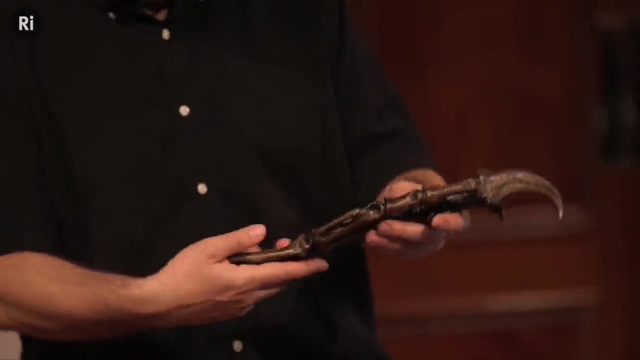 So Albertosaurus lived in Canada Around 70 million years ago, so just before Tyrannosaurus. it was a little bit smaller, maybe around 10 metres or so, And this is the forelimb bones, the radius and ulna and the hand bones. 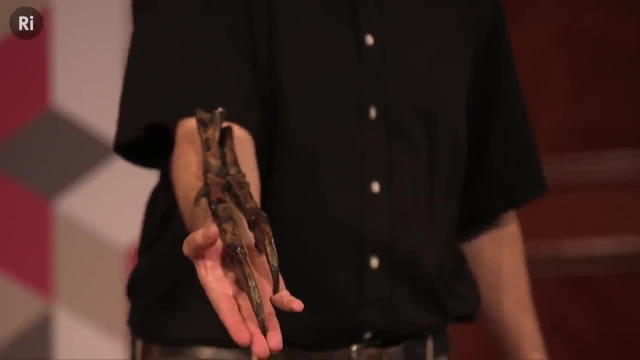 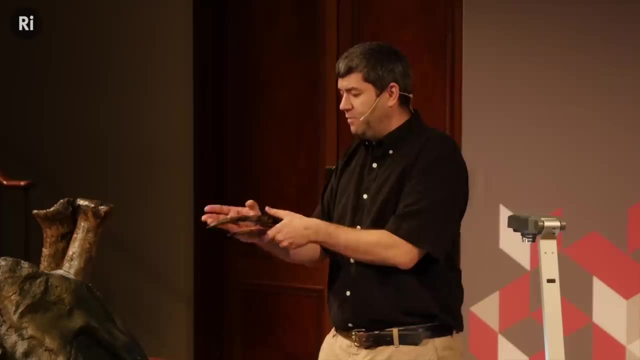 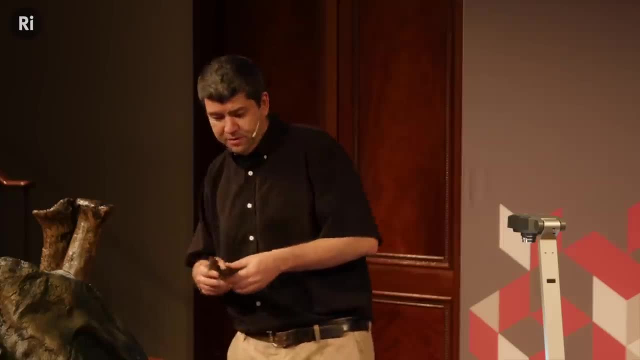 This is a very, very small arm. This is a very, very small arm. This is a very, very small arm, Which suggests they're not actually really using them in the same way. So those arms were really reducing away and becoming kind of less and less effective. 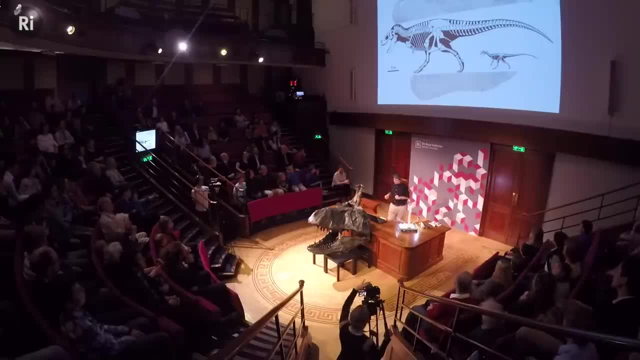 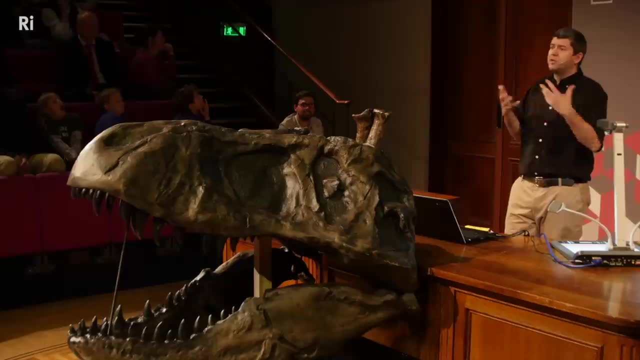 So I've introduced you to about 30 Tyrannosaurs there, if very, very briefly indeed. But how do we know they're all Tyrannosaurs? What actually unifies them together as a single group where we can confidently say: this is one evolutionary plate that we can put together? 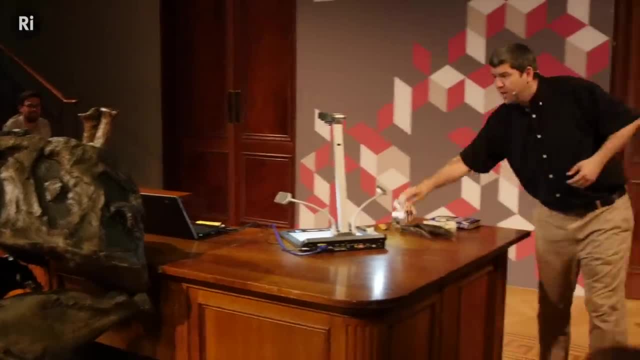 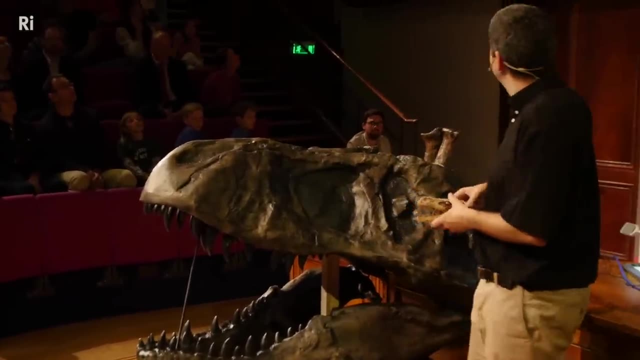 Well, there's actually a couple of features. There's a couple of features that show up quite well, And we see these on every single Tyrannosaur. One of them are the nasal bones. These are the two bones that run along the top of the snout. 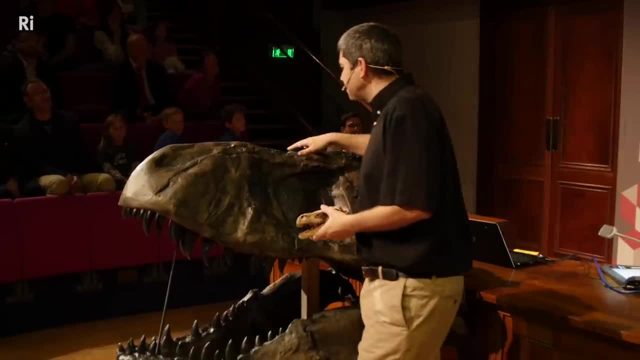 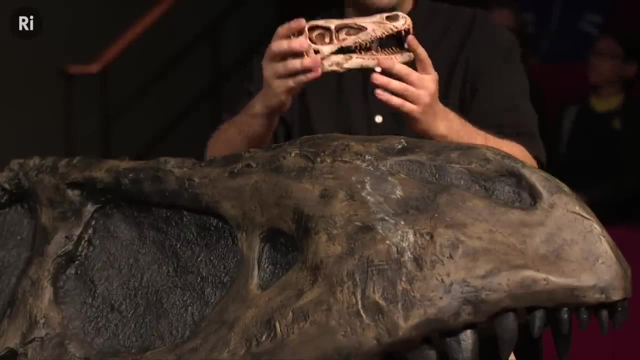 and they basically make up most of the nose. And in basically all other dinosaurs there are a pair, one on the left and one on the right, And if I hold up here my little Velociraptor. so again a nice Jurassic Park reference. 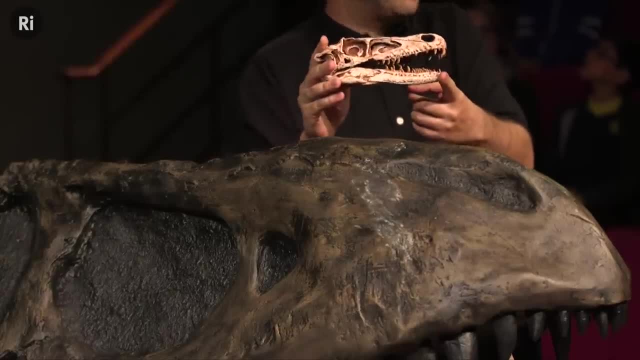 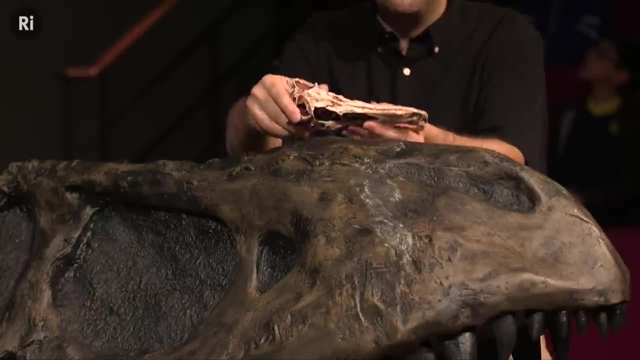 this is not going to fight this. This is how big Velociraptor actually was. I can pretty much fit this skull into just the nose. It's not really a fair fight, But actually if we look at the nasals here, 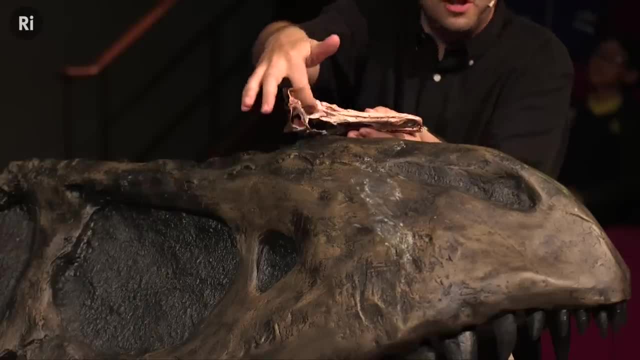 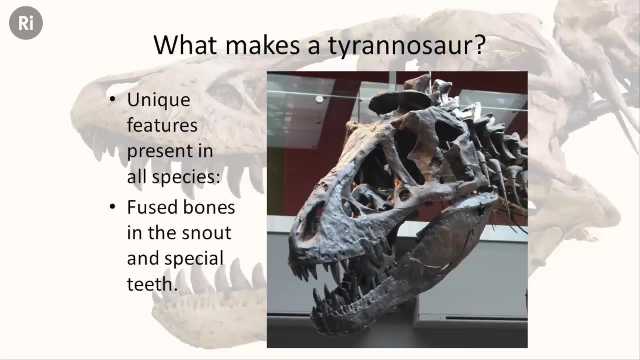 you can see there's two different bones, top and bottom, with a very obvious line separating the two. But in the Tyrannosaurs in Queenie and if we go back to the slides you can see on the skull there they're actually a solid block. 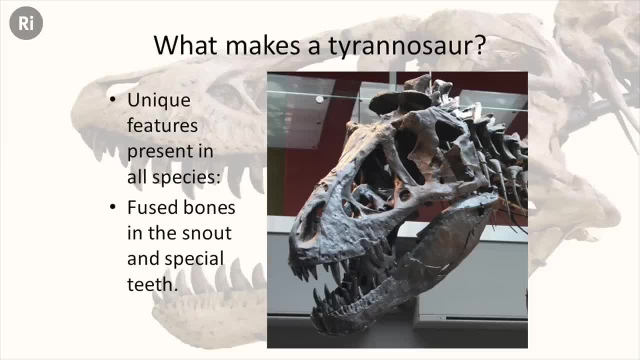 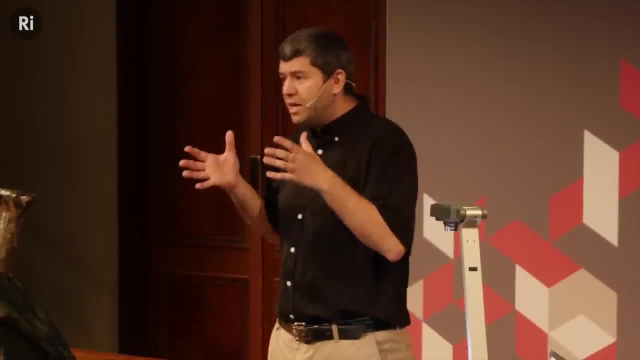 They're fused together in the middle, so they have this lovely solid pair, And that makes the skull very, very solid indeed, And this points to an animal with a very, very strong bite, even in small things like Guanlong and DeLong that were very early on. 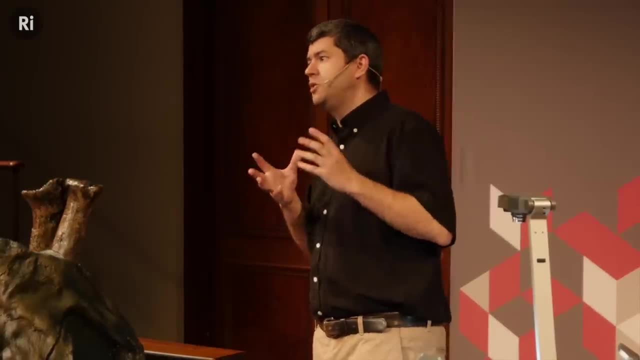 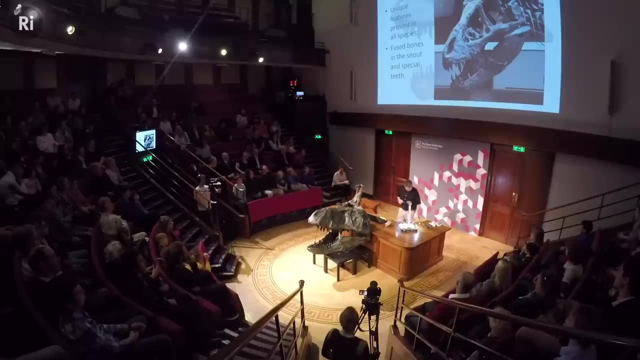 They had fused their nasal bones together and made a really solid skull, And there's no other carnivorous dinosaur that does this. We see that throughout the group. The other thing that they have is the shape of their teeth and, in particular, the teeth at the front of the mouth. 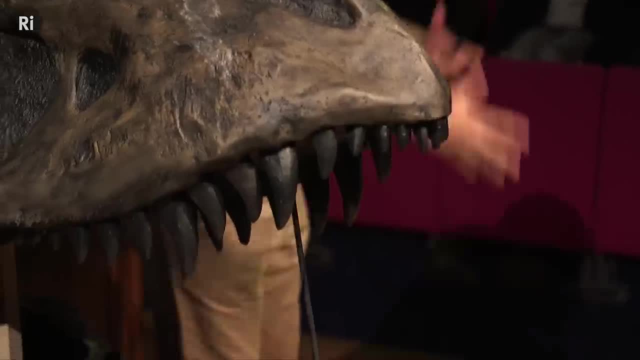 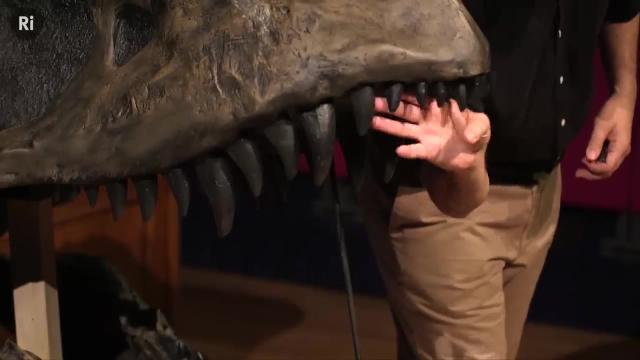 So we have these lovely big biting teeth all the way down the sides of the jaw, very, very large, very, very strong indeed. But if you look around to the front you can see that actually they're really quite small. 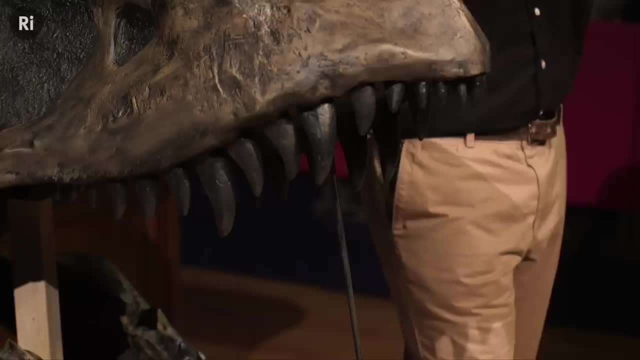 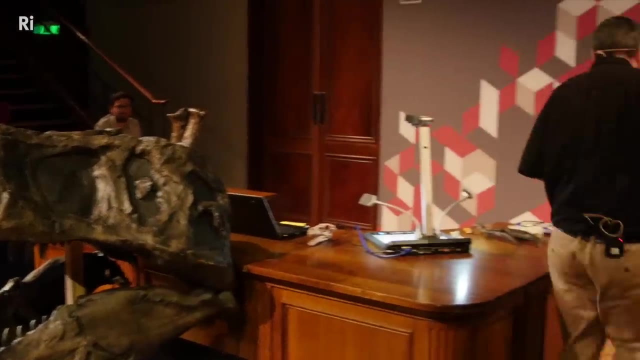 They're not very big at all compared to the side ones and they're all kind of scrunched together. They're a little group kind of all forced up, And this is unique. We see these in the tyrannosaurs and in nothing else. 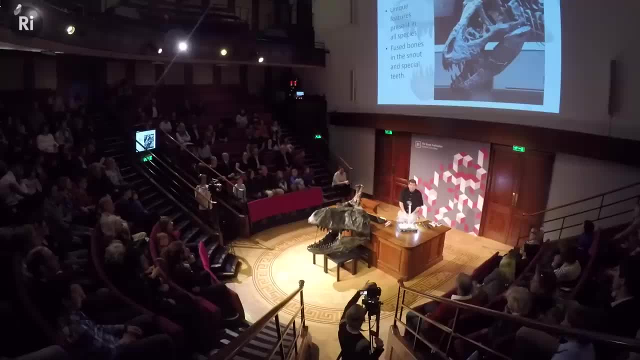 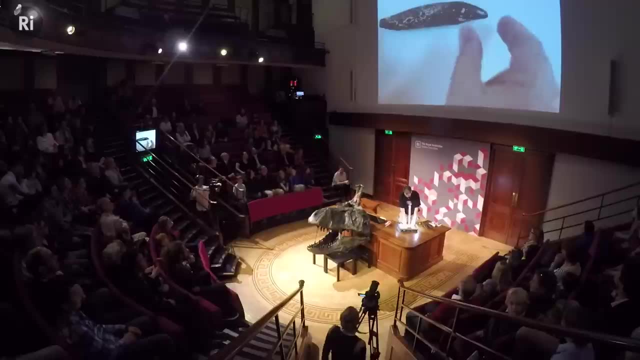 And not only that, but their shape is quite unique as well. So if we can get this up on the camera, hopefully we can see this. Here we go. So this is another cast of one. I see a very, very long root with just a little crown at the top. 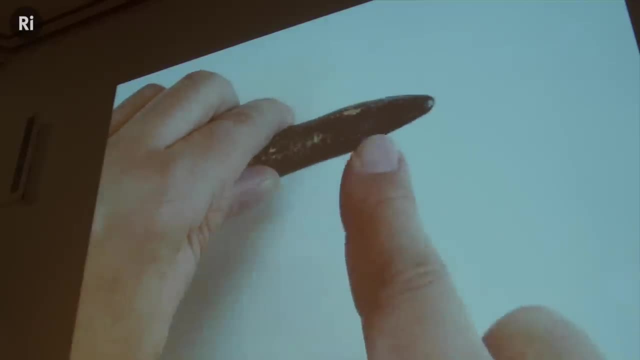 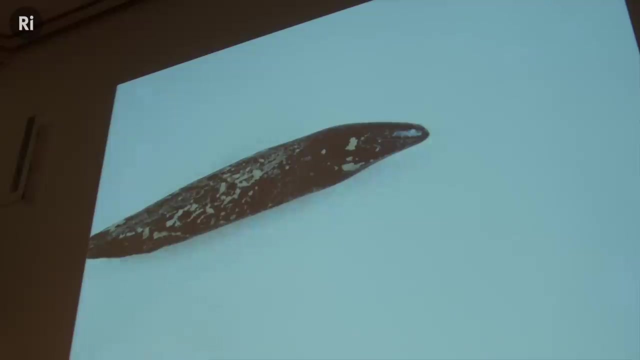 It's very, very thick. It's kind of short and fat, But you can see the rear side is almost completely flattened off, whereas the rest of it is really quite nice and rounded. So if you cut this in half and look down on top, 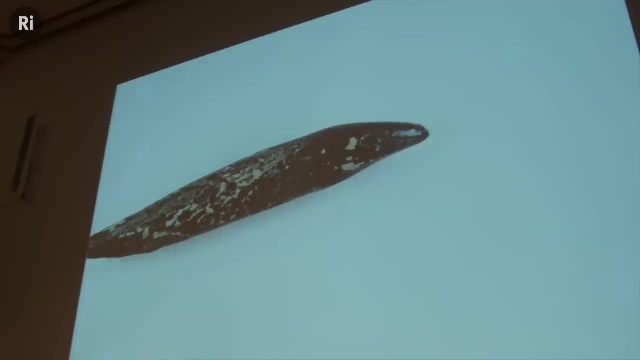 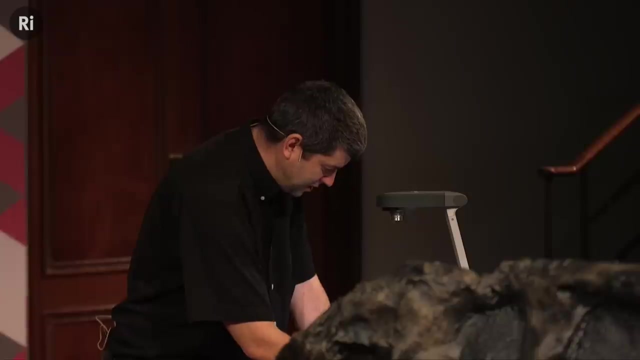 it would look like a capital D. So these are what are called the D-shaped teeth of tyrannosaurs, And if we compare that to the teeth of many other carnivores, so this is an allosaur. you can see that actually this is very, very thin and blade-like on all sides. 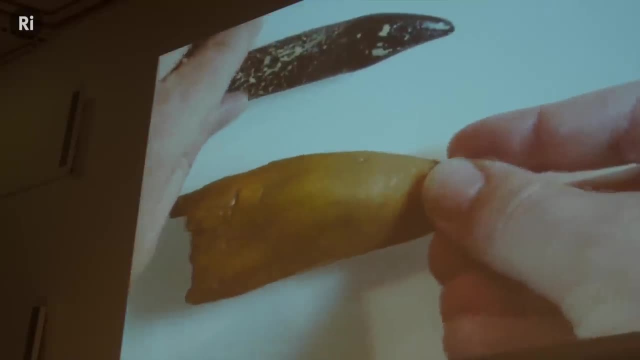 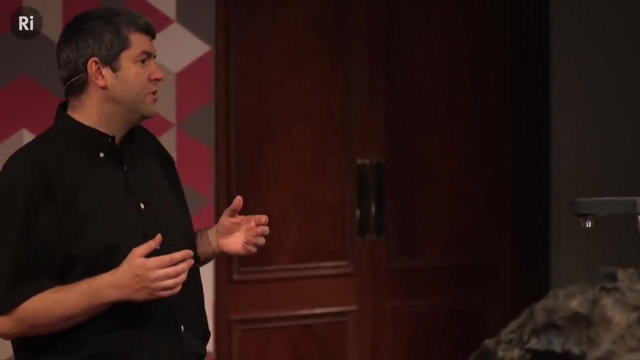 and totally different in shape to what we have with the tyrannosaur teeth. And again, this is what we see in all tyrannosaurs. We see this in the earliest forms, right the way through to Tyrannosaurus. They have these very, very small D-shaped teeth right at the front of the jaw. 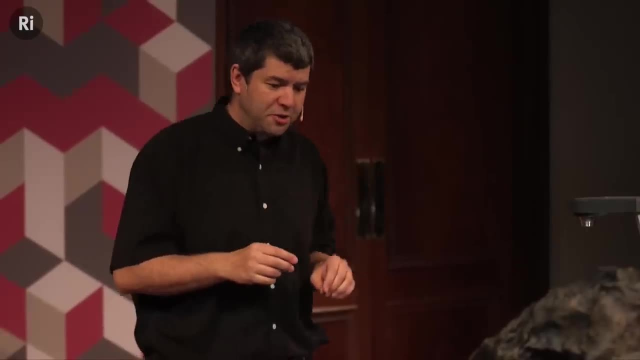 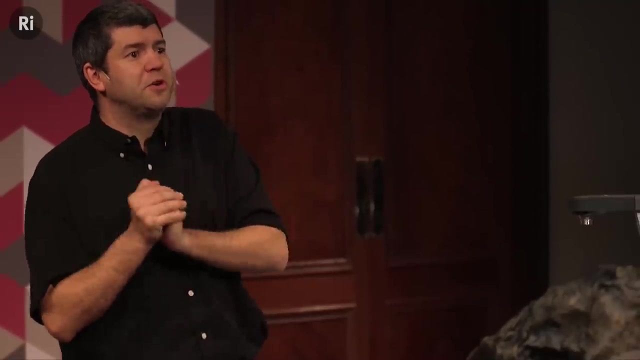 And that gives them a series of unique adaptations which we'll get on to in a little bit of just how they function. So this is one of the ways we can tell tyrannosaurs apart If you ever find yourself in a museum or lost in the desert. 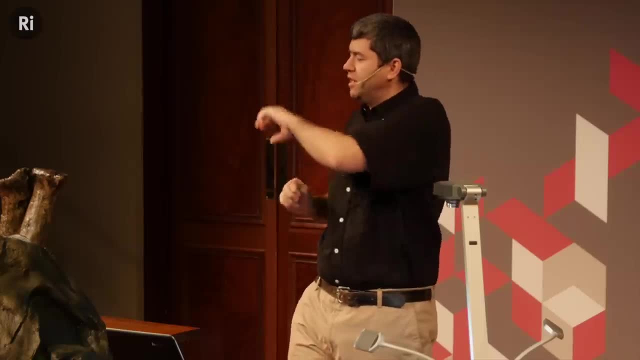 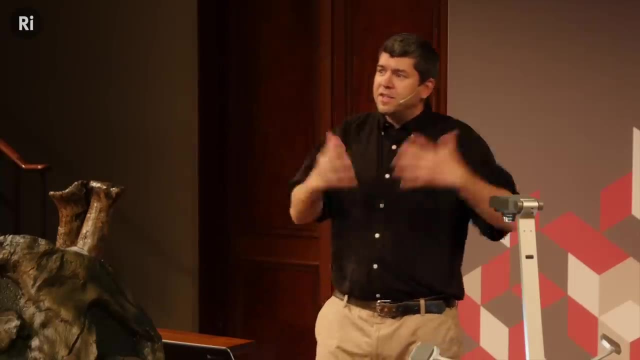 and you manage to find a new skull of a dinosaur and you see that it has fused nasals and little D-shaped teeth at the front. congratulations, you've found a tyrannosaur. So that tells us what they are, but what makes them special? 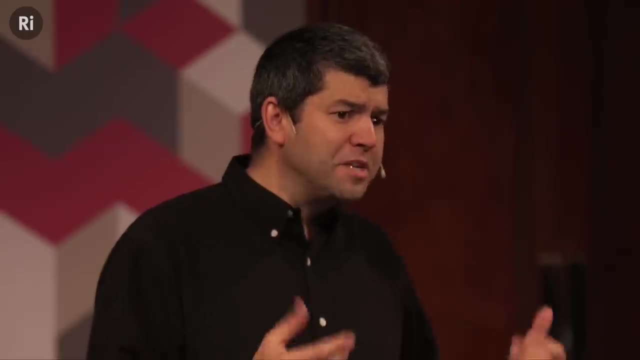 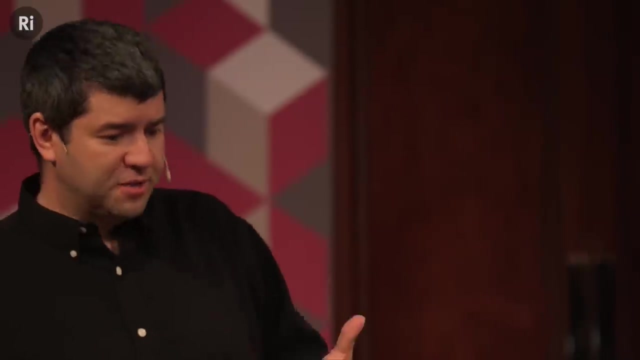 Why are they interesting and unique? Well, there's a number of features, and one of them actually is the kind of shape of the skull. Tyrannosaurus is particularly exaggerated in this sense, though it's true of the tyrannosaurs generally. 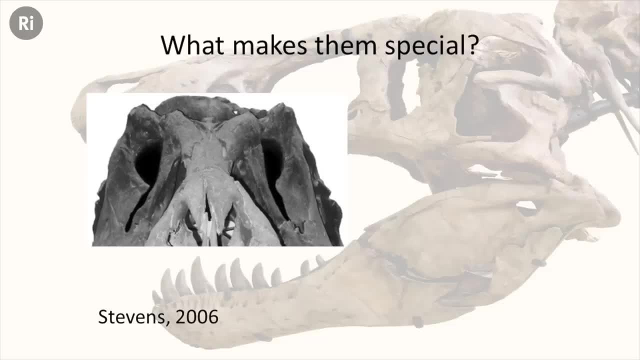 So here again, actually, you can see the beautiful fused nasals. You can see there's no line up the middle, They're absolutely solid. And here we're, looking straight up the nose, exactly the view that the audience have at the front here. 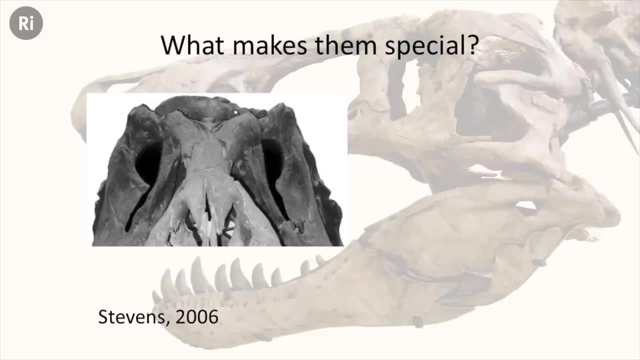 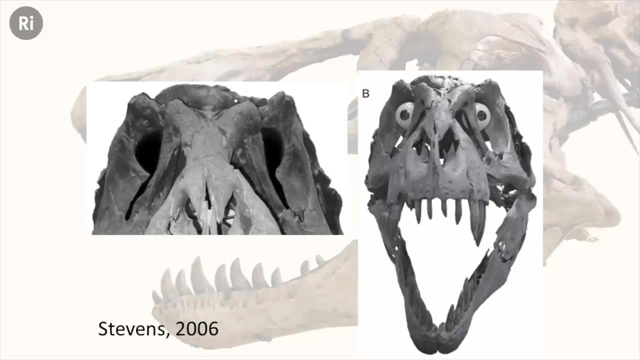 straight down are those two lovely big eye sockets. And what happens? when you fill in those eye sockets? You get this, which is always good for a laugh, but it tells you something about their shape. These are binocular animals. These are animals with big, forward-facing eyes that are looking at things. 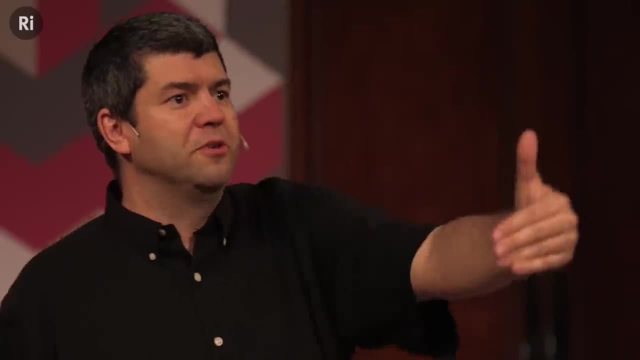 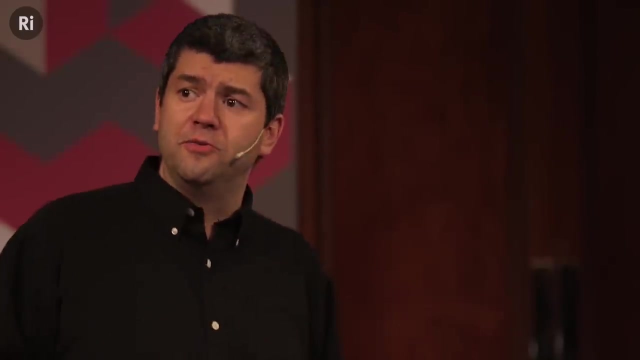 This means it's a carnivore, It is judging distances, It wants to know how far away it is from something that it is very interested in. And this is a totally different arrangement of the head to what you would see in herbivores- sheep, cows, rabbits. 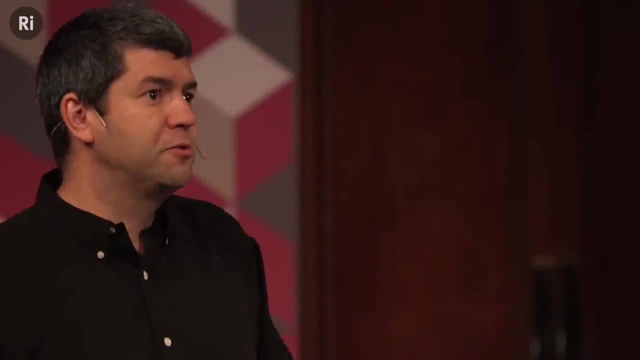 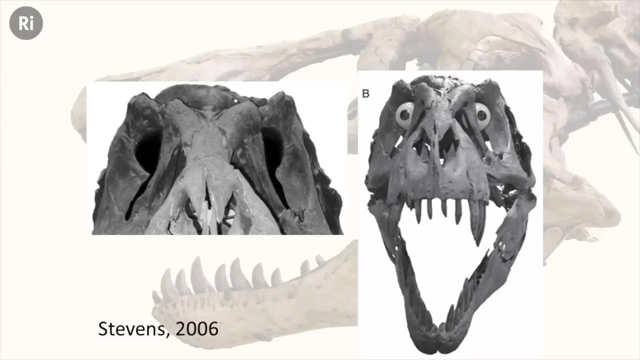 They all have eyes on the side of the head because they want to look around them and want to avoid things that are going to eat them- not something that is coming to be eaten, But what you can see here as well, though, is also the size of those eyes. 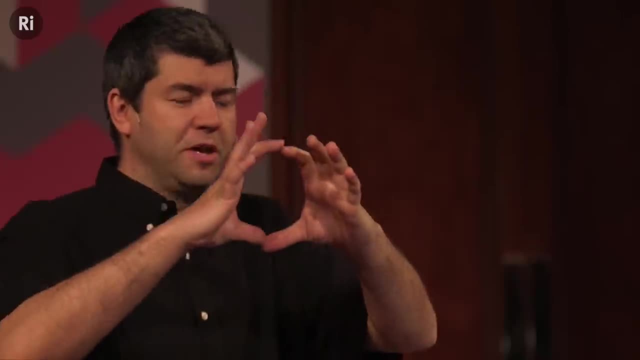 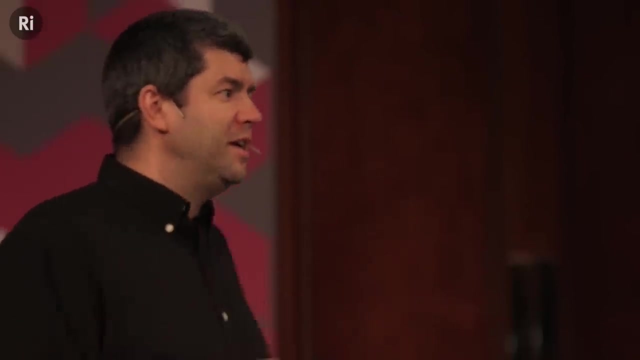 The eyes of Tyrannosaurus are absolutely enormous. They're going to be about this big. That's how big an eyeball you need to fit in the skull. Now, even though this is absolutely huge, it doesn't look very big on the head. 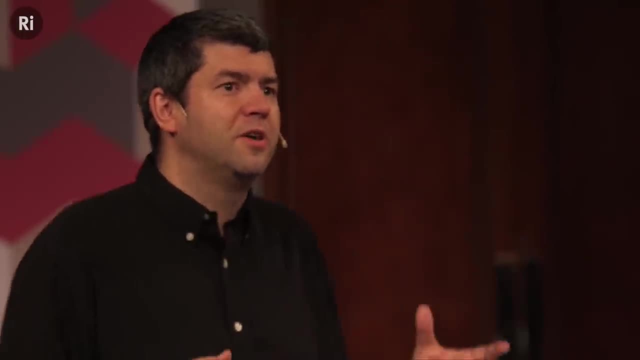 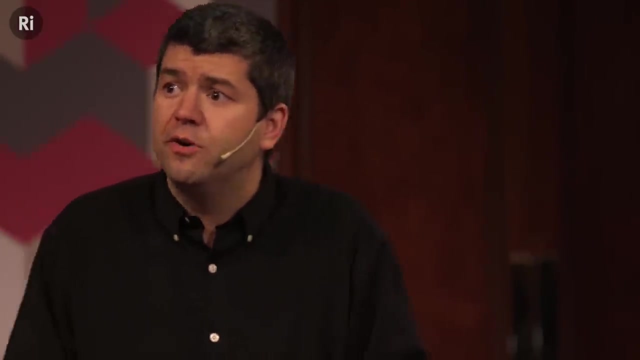 simply because the head is so absolutely, enormously outsized. But if you're looking at eyesight, one of the critical factors as to how good your eyesight is is just how big your eyes are. This is whether or not you want to have a very refined sense of vision. 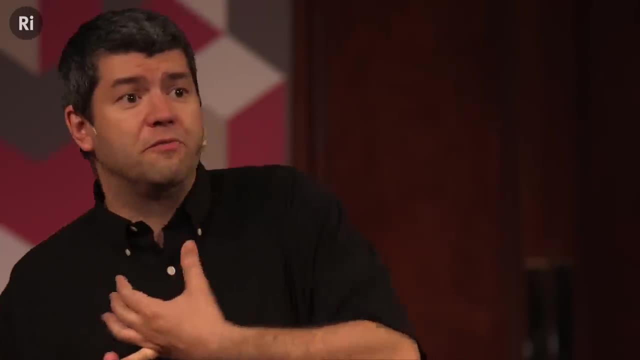 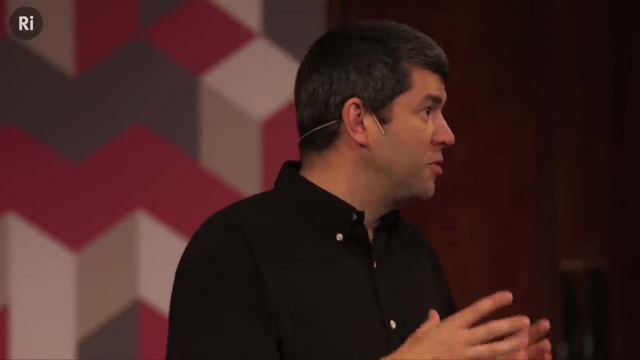 or whether you want to see in the dark, So you can think about things both like vultures and owls. Vultures have extremely good eyesight. Owls see very well in the dark. Either way, you want a big eye. 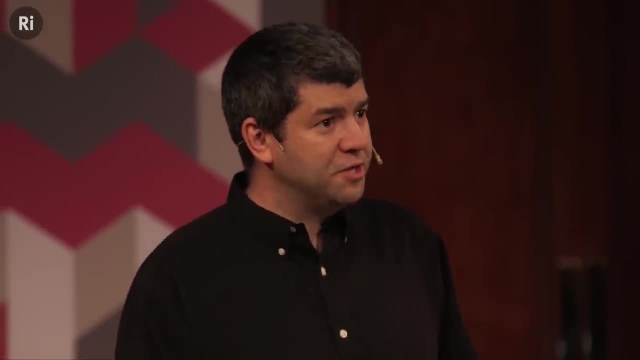 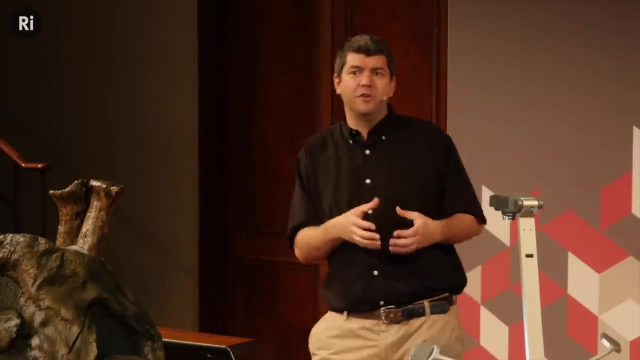 And basically, the bigger the eye you have, the better your vision. And it's all about absolute size, not relative size. So actually Tyrannosaurus, believe it or not, has the largest eye that we know of for any terrestrial animal ever. 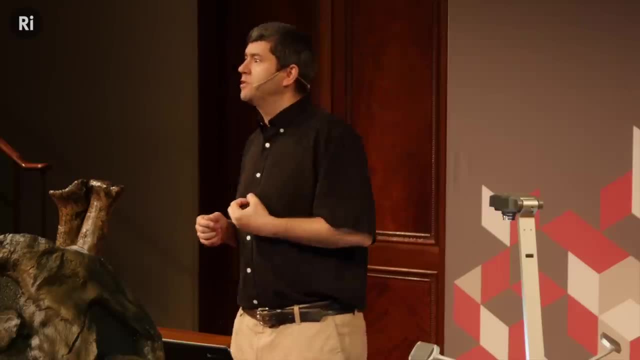 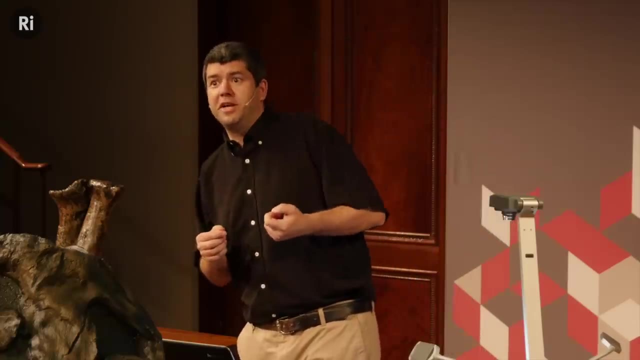 This is an animal with superb eyesight. So just to bust another Jurassic Park-era myth, this is not something that can't see you if you don't move. This has got the greatest eyesight of any animal on land ever that we can know of. 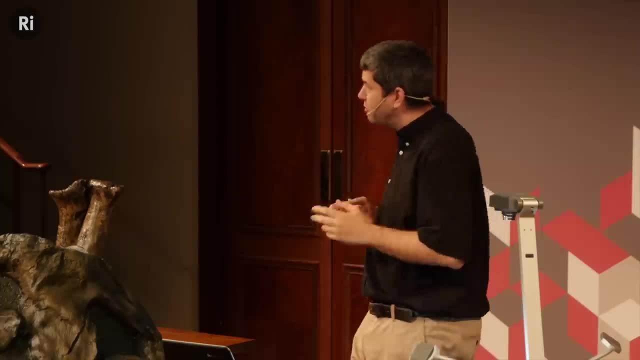 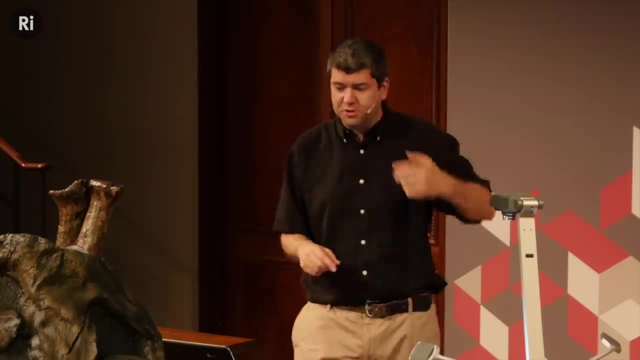 Yes, It does suggest it could see you quite well, and sitting still is probably not a very big defense. But also on top of that, the skull is extremely wide. If we compare Tyrannosaurus to other large carnivores, this is a thing called Carcharodontosaurus. 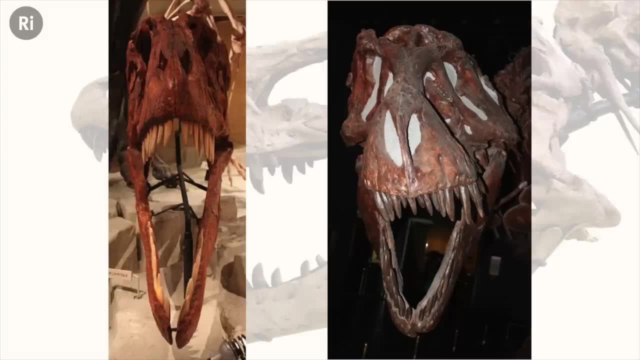 which is actually nearly as big as T rex. This is a very, very large animal indeed And you can see, the skull is extremely narrow. The eyes still point forwards, but the skull as a whole is very narrow. It is a similar-sized skull. 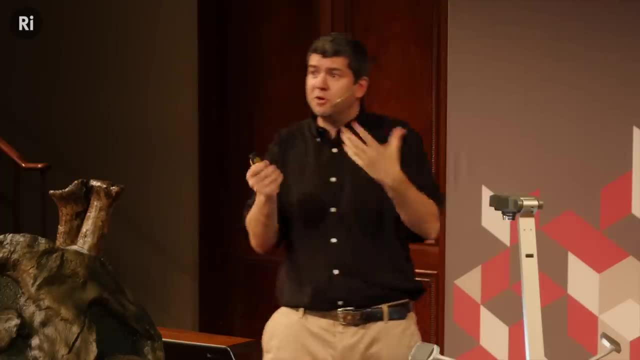 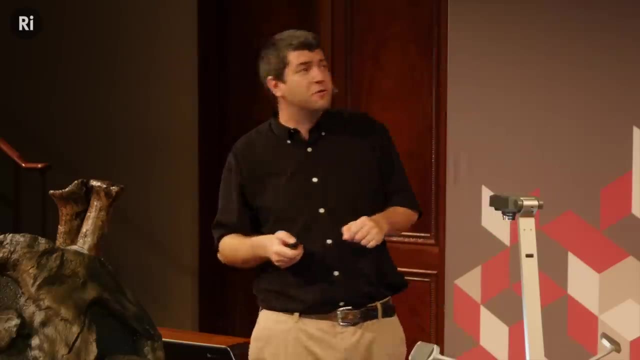 to the one we see on the right which, as you can see, is slightly crushed. This is one of the problems of working in paleontology: Even things like whole Tyrannosaurus skulls tend to get crushed after a few tens of million years. 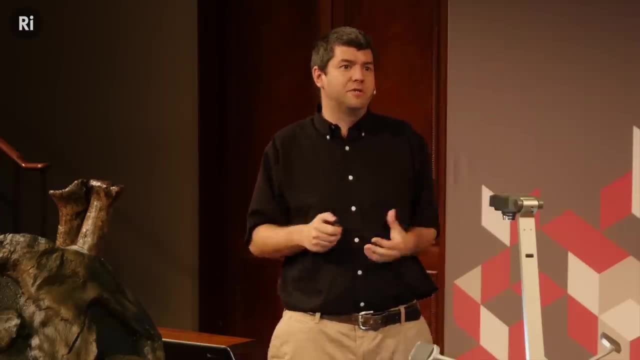 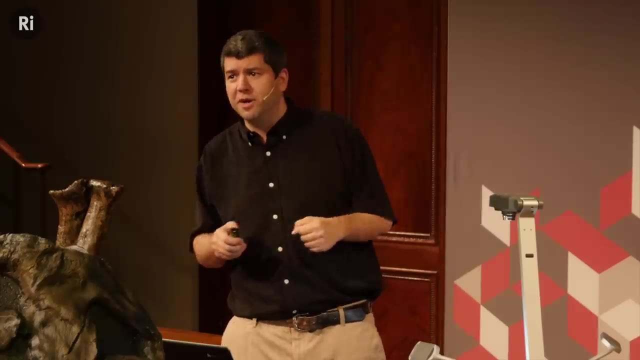 But you can still see the overall width of that skull is very, considerably wider. This is a very, very broad head indeed, And this is one of the other trends that we see. The early Tyrannosaurs not so much, But by the time you start getting to the really big guys, 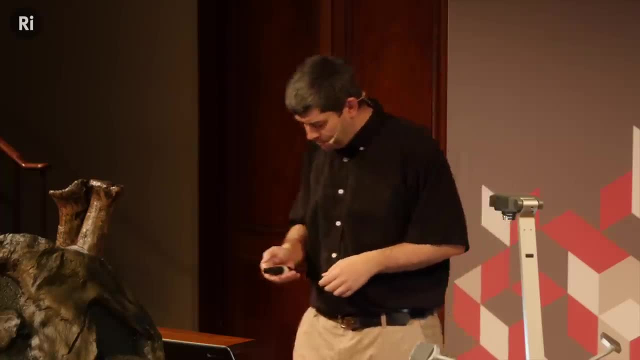 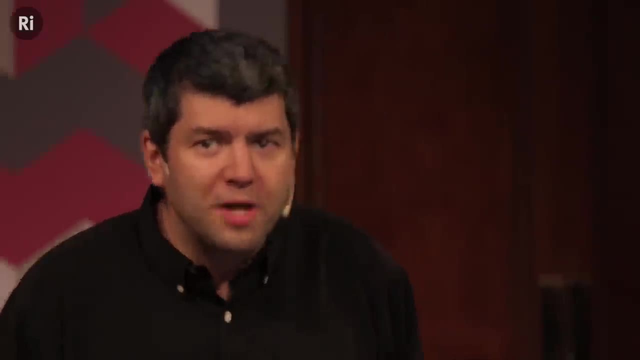 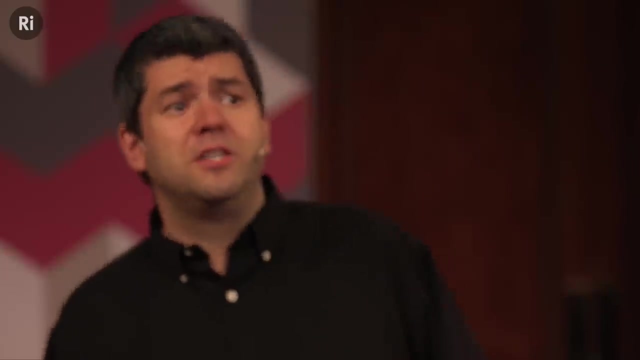 they have this very, very, very broad head. If you're getting very big it can take quite a while. So, Sue, 12-plus metres, seven, eight tonnes maybe, And Tyrannosaurs actually grew very fast. Dinosaurs actually generally grew quite quickly to get to adult size. But even within them, Tyrannosaurus itself actually is a bit of an outlier. If we look at some lovely growth curves here, we can basically see that several nearly Tyrannosaurus-sized animals display here: Spleedosaurus, Gorgosaurus and Albertosaurus- all from North America. 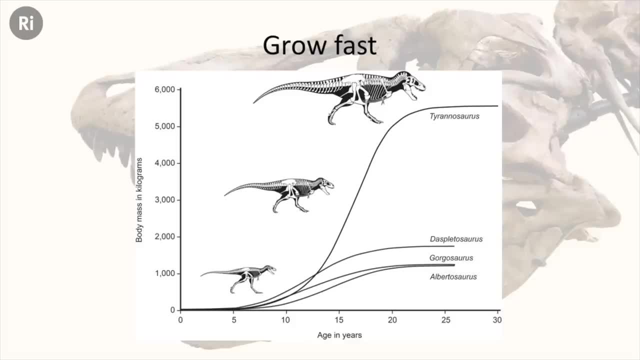 took about 15 years or so, maybe 20 years, to get to full size, And that was two or so tonnes. Some of the bigger ones are probably rather larger. Tyrannosaurus, however, goes through this beautiful growth spurt around 10 to 20 years where it absolutely balloons. 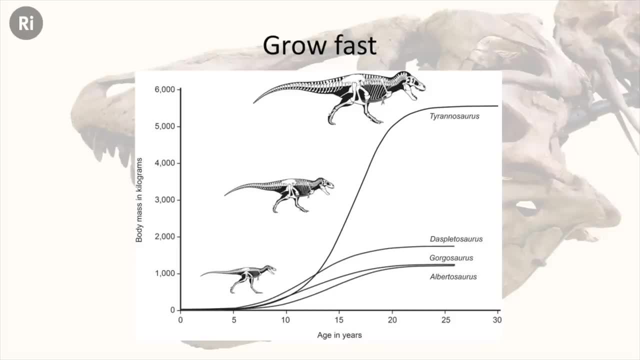 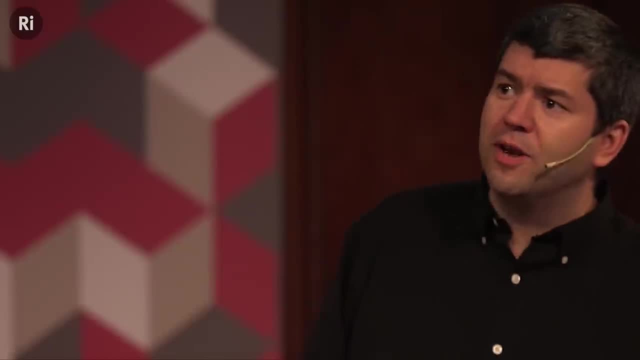 It gets very, very large very, very quickly. So this is an extremely fast-growing animal And that gives you a real sense of you know just what's kind of going on metabolically to grow at that kind of rate. I mean, this is the maximum growth spurt that humans have sustained. 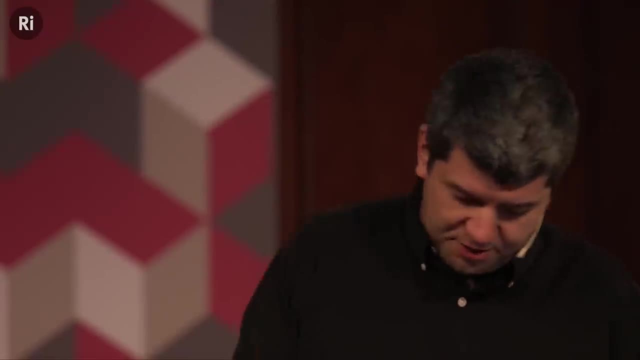 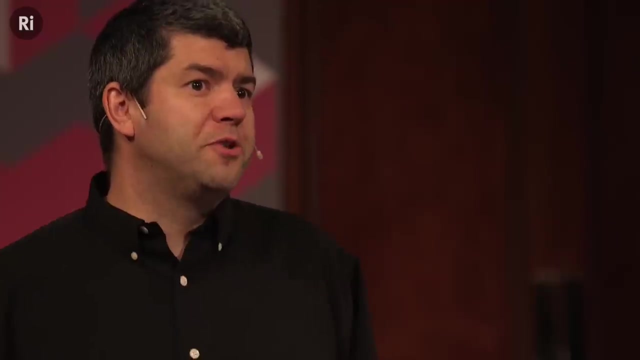 over multiple years and in the range of things that are tonnes in weight. But what's really quite neat is that they don't just grow fast and grow very big, but they actually change shape quite dramatically as they do, so This perhaps isn't so much of a surprise. 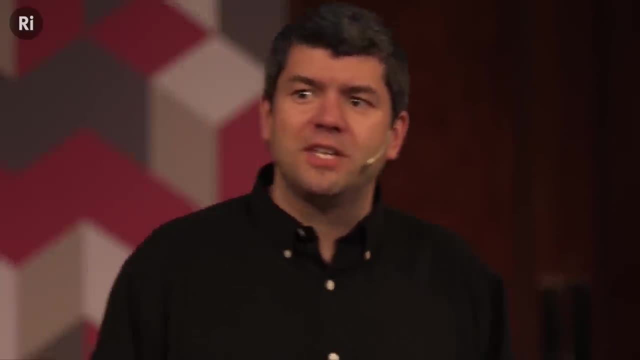 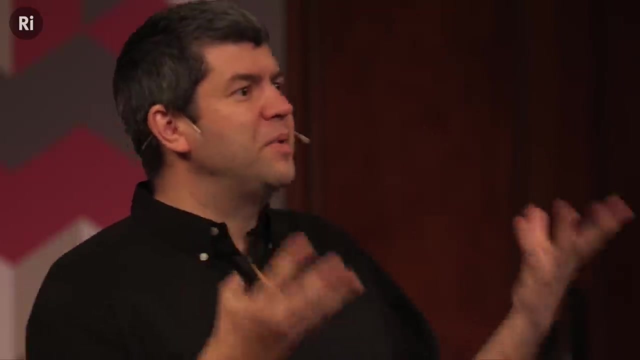 If you think about humans, if you think about any animals, most things actually change shape a bit As they grow. You know, we famously think of puppies and kittens and babies as having big heads and big hands and big feet, And then you kind of grow into them as you grow up. 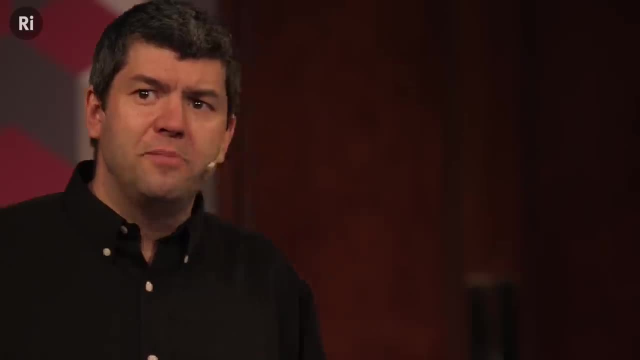 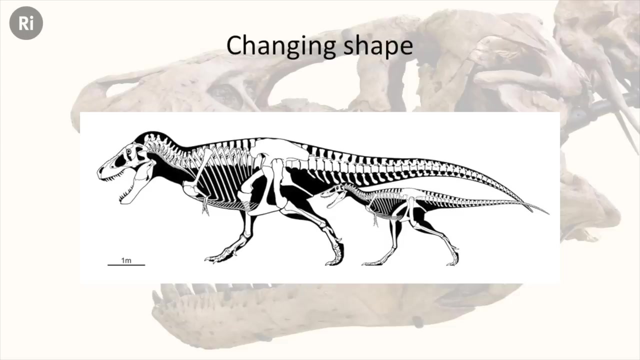 So it shouldn't be a big shock that dinosaurs change shape as well, But it's noticeable just how much they change when it comes to the tyrannosaurs. So this is a skeleton on the right which is known as Jane, And Jane is, as you can see, about half grown. 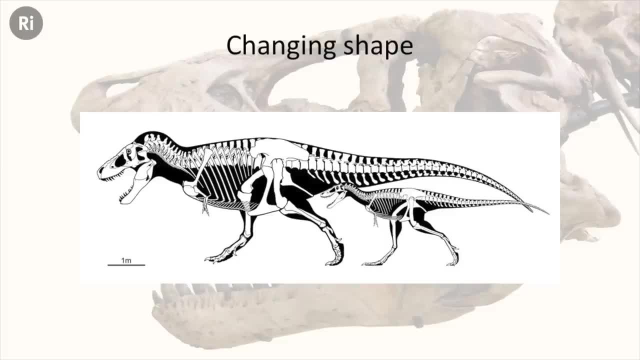 at least in terms of length. so about five, six metres long or so, And yet the head is absolutely tiny compared to that of a full-sized tyrannosaurus. So, whereas we think of babies usually as being big-headed, and then it takes a while for them to you know. 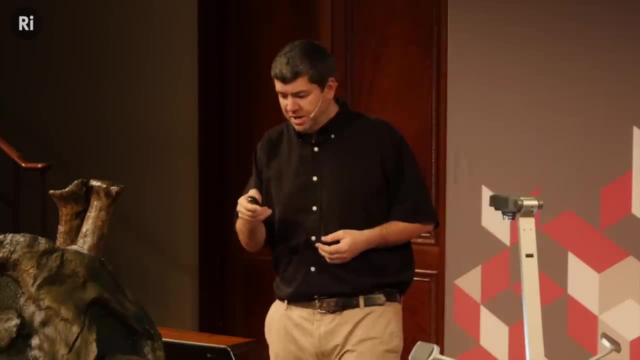 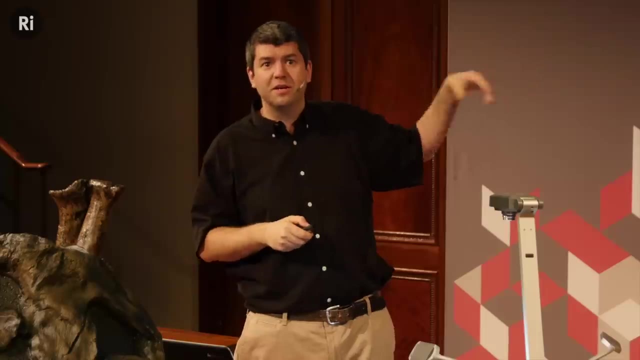 your body kind of grows into your head or vice versa. we see here that actually the young one has a small head And by the time it's got to full size, its head has got proportionally much, much bigger. We also see that, Jane, though tyrannosaurs generally have long legs- 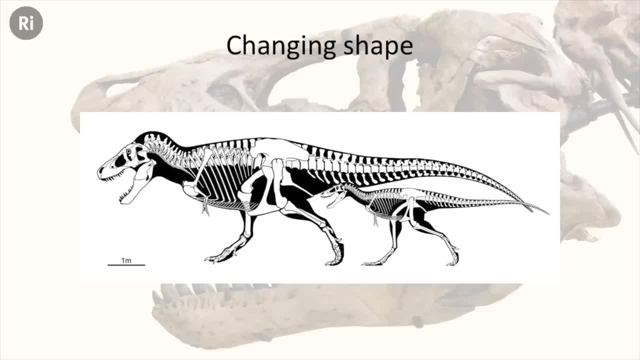 Jane has really quite long legs, a really quite slender body and quite a slender neck, So this points to an animal that's doing something actually quite different. The head is built differently, the legs are built differently. This is an animal which is running in a different way. 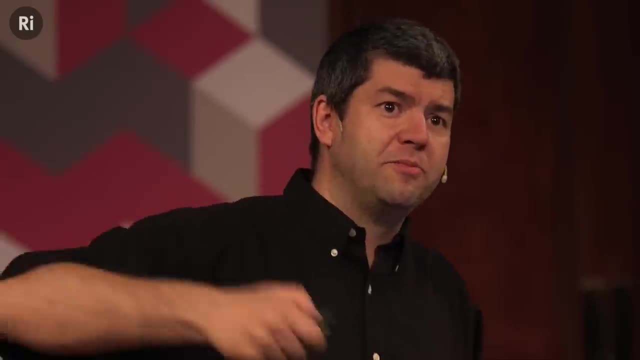 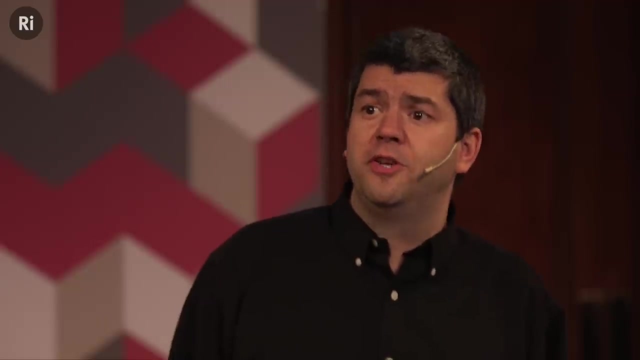 and probably feeding in a different way. So we're not just seeing them growing and we're not just seeing them changing in shape, but the implication for this is that they're also fundamentally changing in their ecology and their behaviour as well, And therefore actually in some ways, 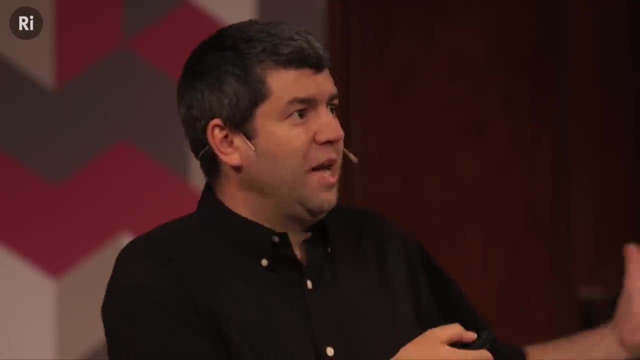 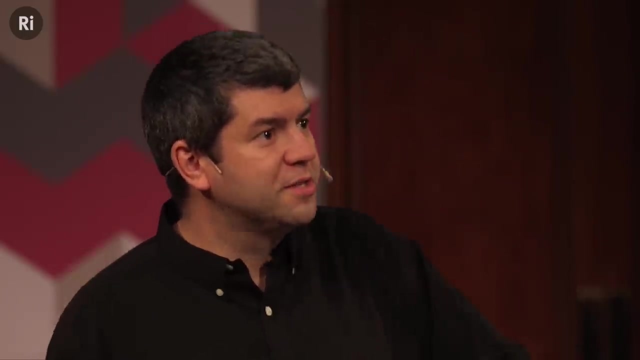 you could treat these as two different species. The big adults are living and hunting and acting in a way that the smaller juveniles aren't, And they're shifting from one to the other as they grow. This is not actually that unusual. We see exactly the same thing in various snakes, lizards, crocodiles. 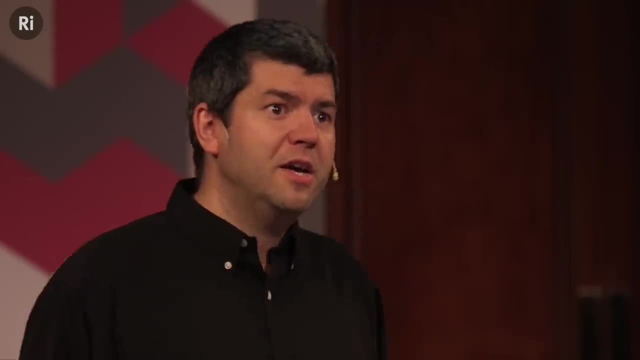 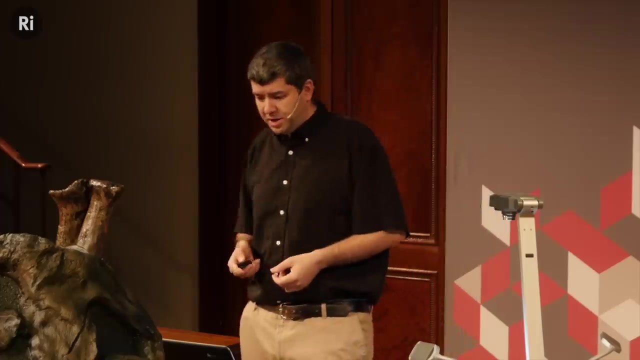 and other relatively slow-growing animals that are around today, But it really shifts the dynamic of how we think of these species interacting with others in an ecosystem when we know that they can have such dramatic changes. One thing that's really important here is these legs. 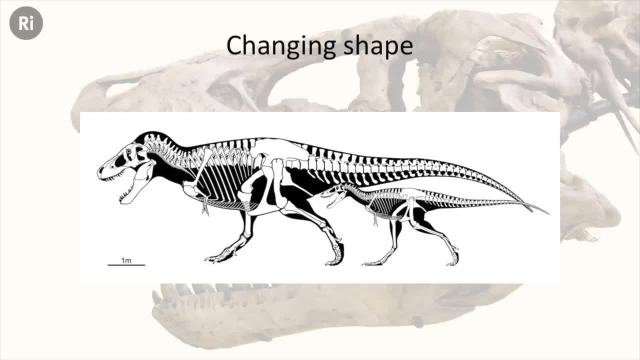 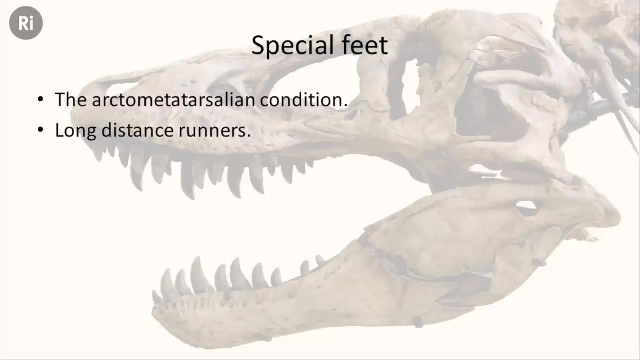 and in particular these feet, because this is another really special adaptation that we see in tyrannosaurs, And this goes by the magnificently tongue-twisting name of the arctometatarsalian condition. I know it's lovely, But actually it's really worth having a word like that. 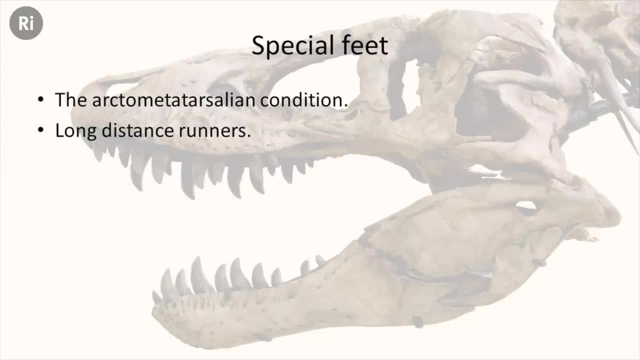 because it's easier to say arctometatarsalian, or at least when it is, when you've said it quite a few times- than it is to say that special condition where the weird metatarsal is kind of shrunk at one end. 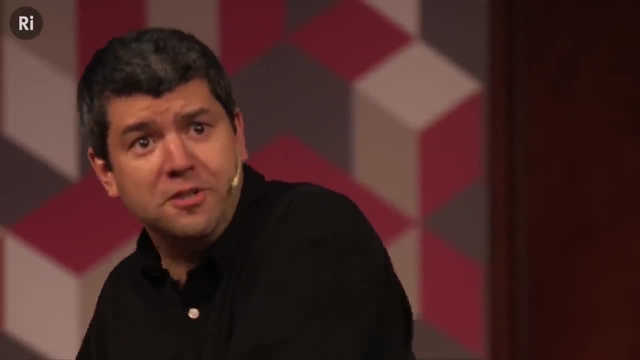 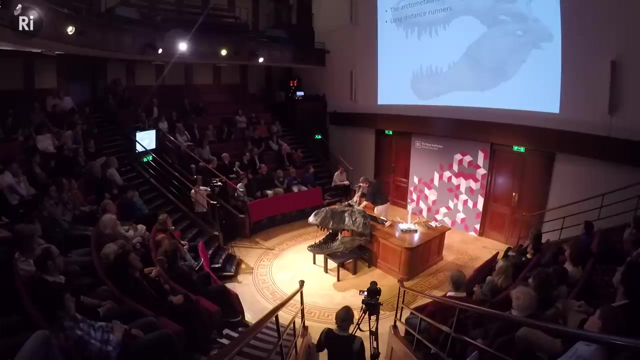 but wide at the bottom and it's kind of pinched between the other two and it changes how the foot functions, Because that's what it means. But arctometatarsalian is actually easier. So if we look at a tyrannosaurus foot, 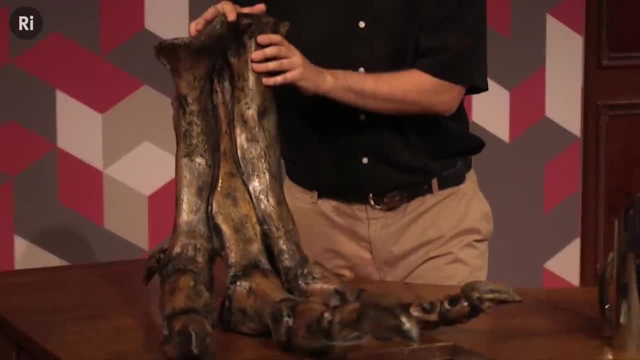 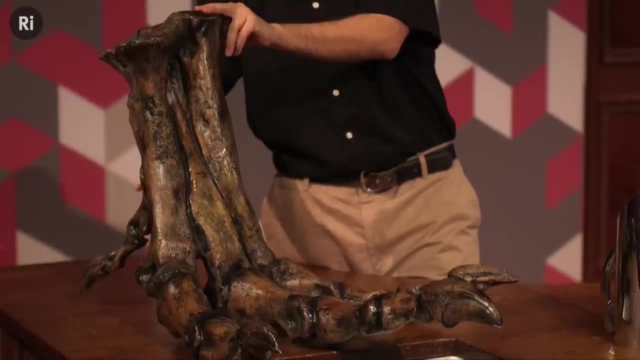 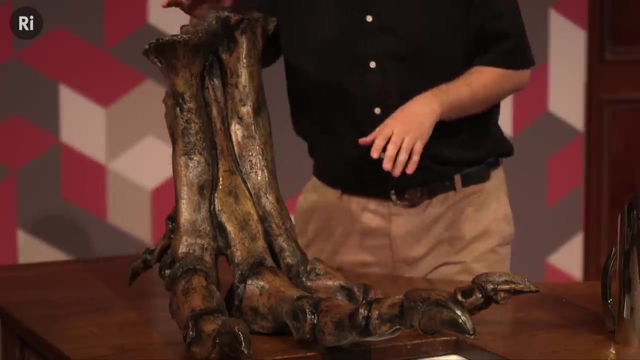 this is the foot from a nearly complete, or nearly full-size tyrannosaurus. It's a right foot, So they have four toes. The first toe, what for us? sorry, it sticks out at the back a little, So it's almost like the dew claw that you get on a cat or a dog. 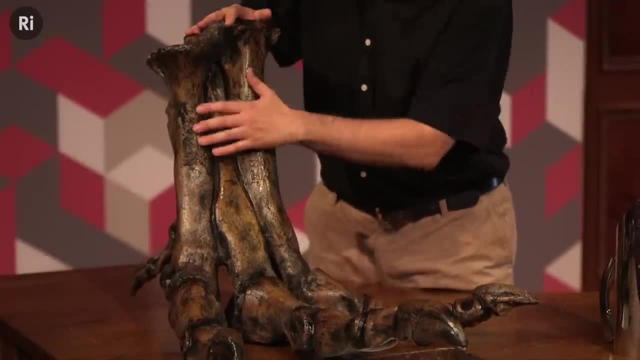 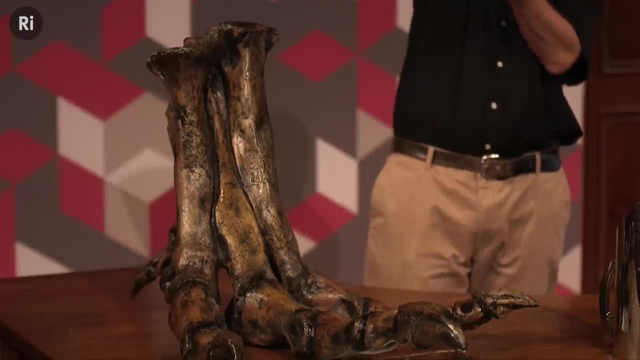 And then three walking toes, And these are the metatarsals, the bane of the footballer. We're forever hearing about broken metatarsals. So we walk on the flats of our feet, We have both our toes on the ground and we have our metatarsals on the ground. 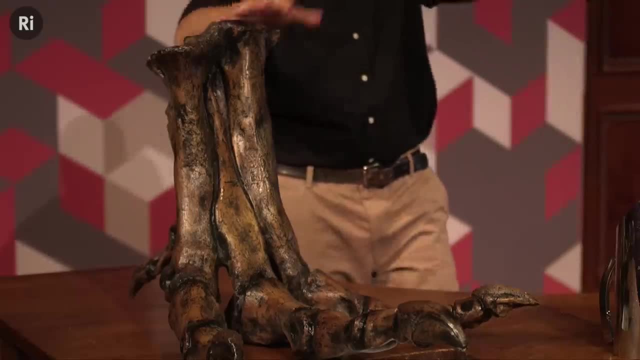 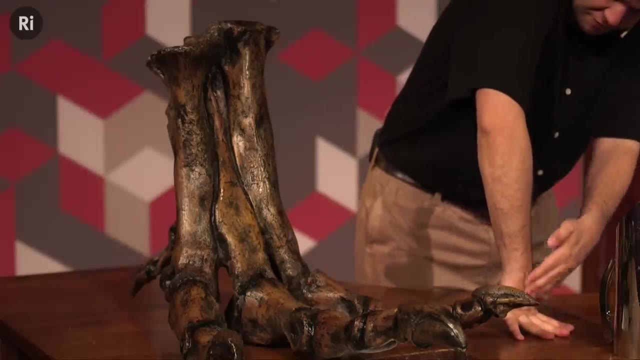 We walk across the whole foot. The dinosaurs and indeed the birds and many other animals just walk on the toes. So they've elevated the foot and they have the metatarsals or, in the case of my hand, metacarpals. 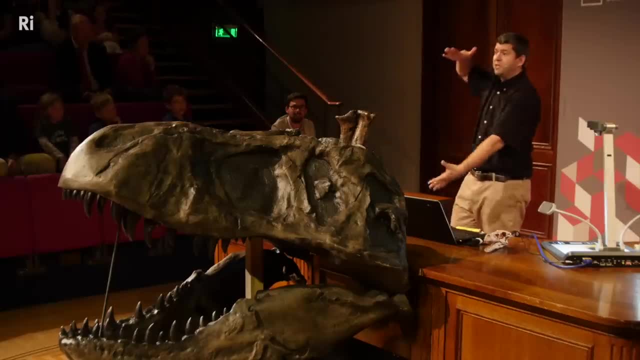 suspended, if you like, upright, And this actually already automatically kind of extends the length of the leg. It gives you a longer leg to run on. So this is actually going to speed you up because it means you're taking longer steps for every pace. 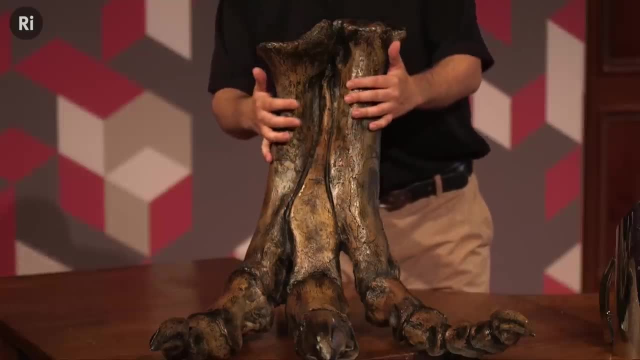 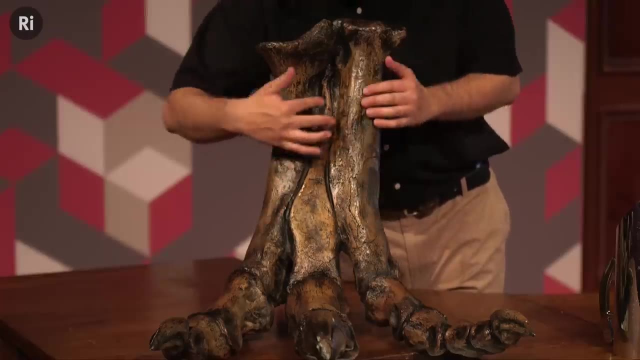 But if we look to the middle, what you'd see on most dinosaurs- in fact the vast majority of them, in particular the carnivores- is the three metatarsals, for the three running toes would all look like this: They'd be lovely long, big blocks, nice vertical strips. 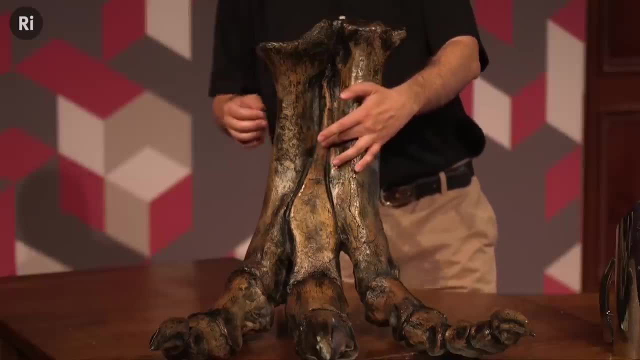 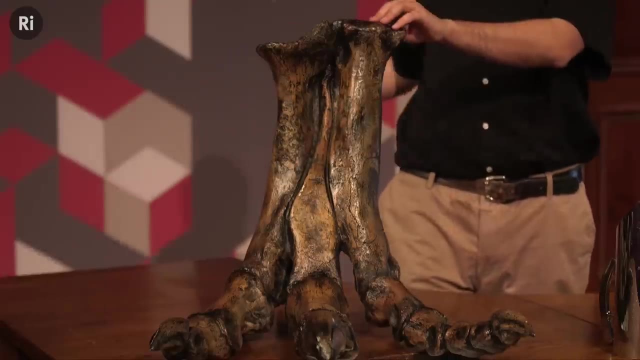 But we see here this middle one kind of vanishes and it's being crushed between the other two and it looks like it's kind of disappeared and like it's going to come out the back. But actually it doesn't. It really is being crushed. 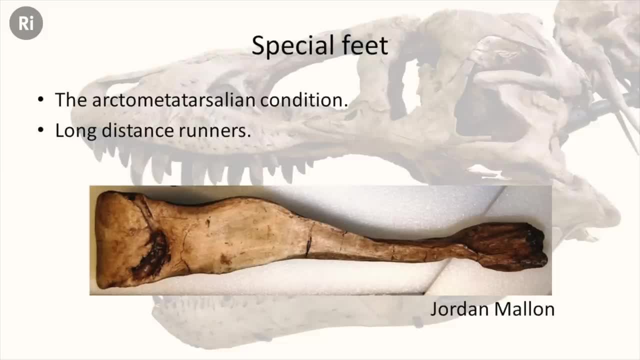 And we can see that If we can switch back up to the slides, There we go. So here it is. This is just the middle one, And you can see the top just kind of vanishes. It just absolutely disappears. I've actually got a real one here. 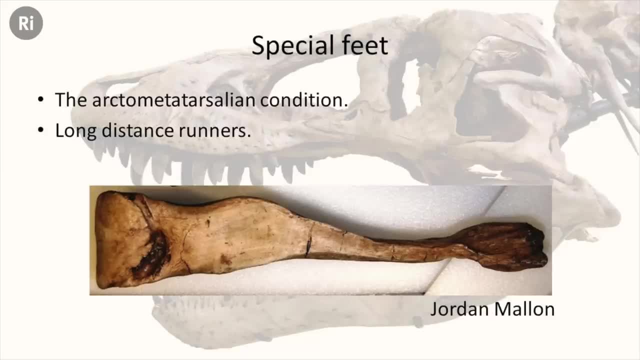 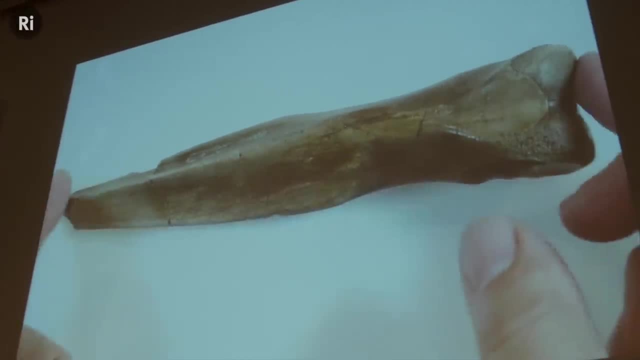 So this is online from the Royal Tyrrell Museum in Alberta. It's actually from another dinosaur. It's not actually a tyrannosaur, but two or three different groups all evolved an arctometatarsal, And you can see here totally crushed in. 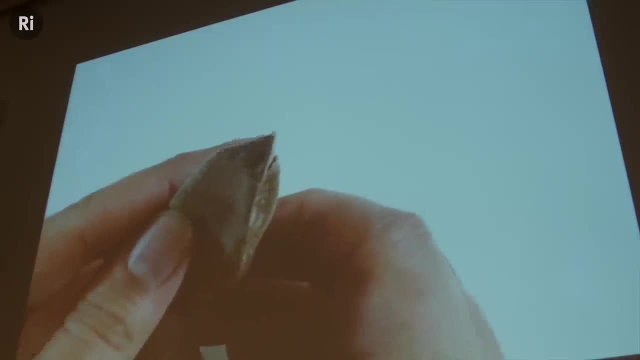 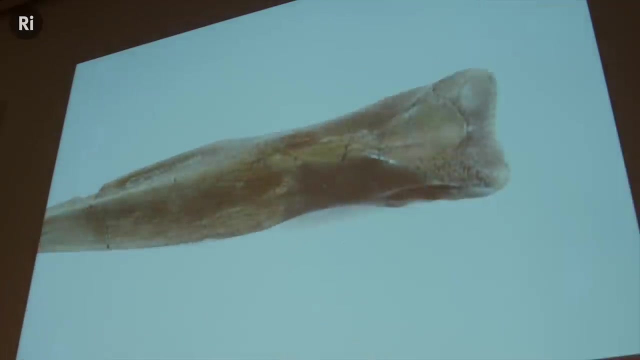 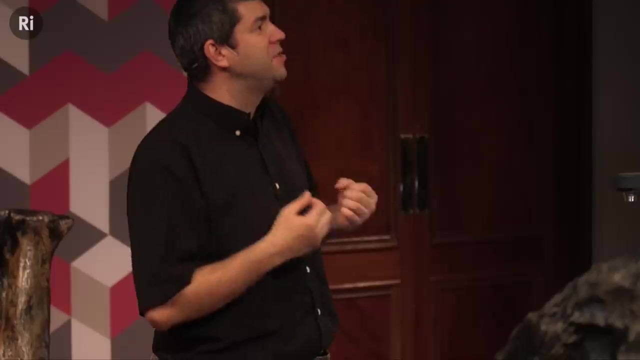 This is where the other two would attach, And if that shows up, you can see the cross section. It's this tiny squished triangle, So it really has completely crushed effectively that middle metatarsal And this is actually a really interesting feature. 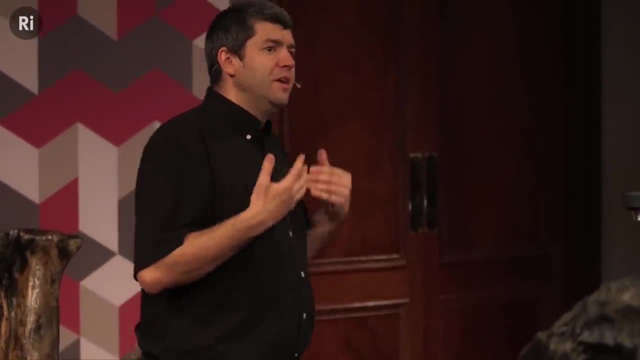 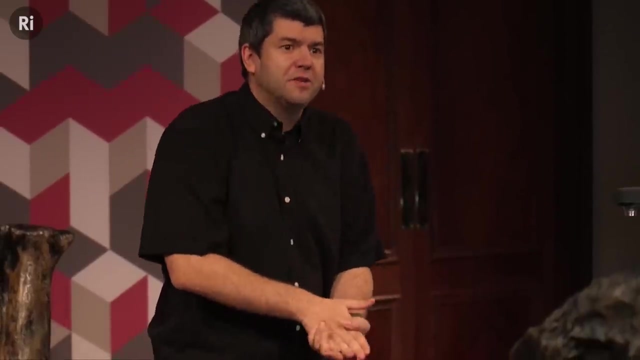 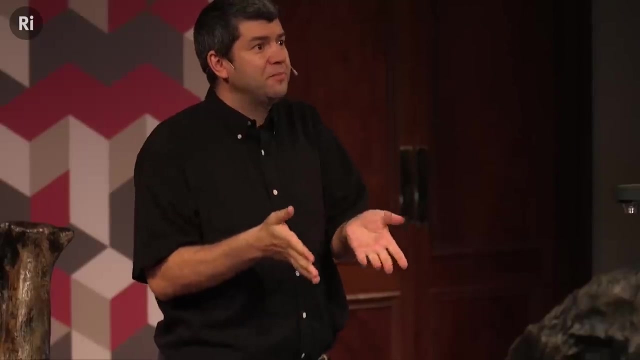 because this totally changes how the foot moves. If you can imagine, you want to be a long-distance runner. every time you hit the ground, every time you take a step, your bones are all slightly moving And that represents lost energy, Because if they don't, what you actually tend to do- 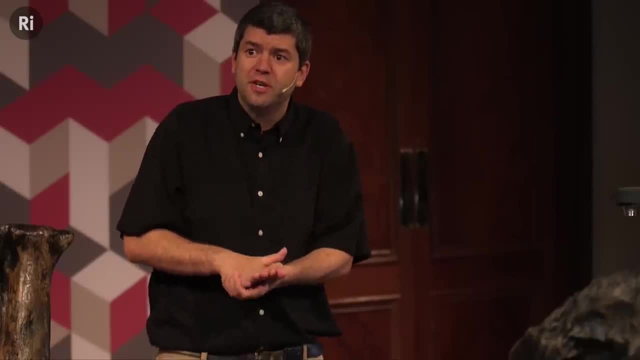 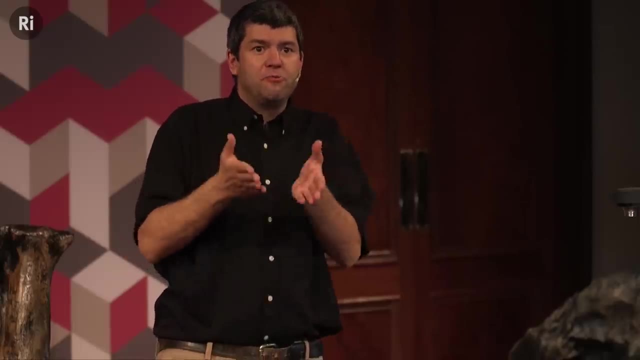 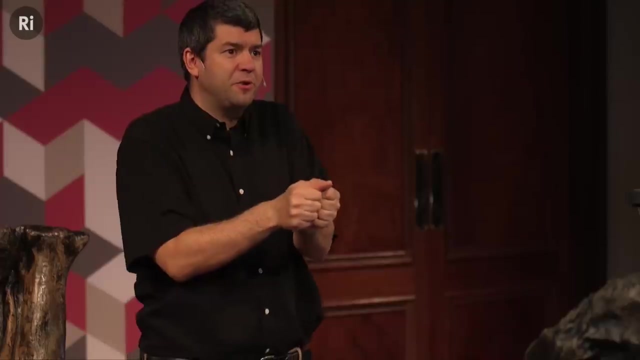 is start compressing some of your ligaments and some of your joints And as you step off again, that springs back and you get a little bit of energy back. So what you really want to do is to minimise all of the movement. You want to have everything as firmly and tightly together as possible. 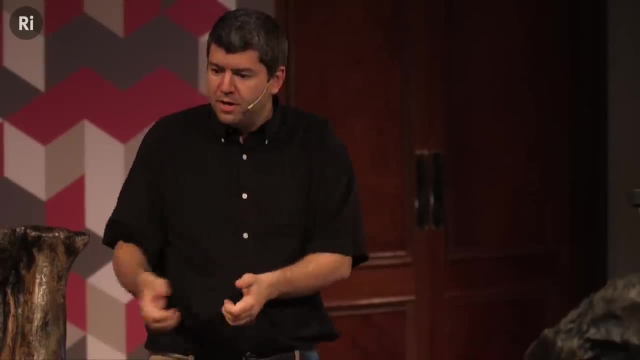 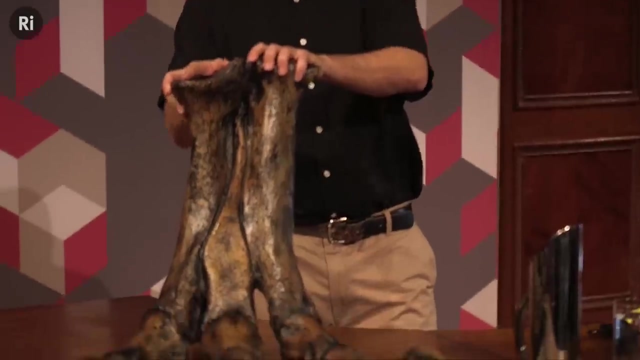 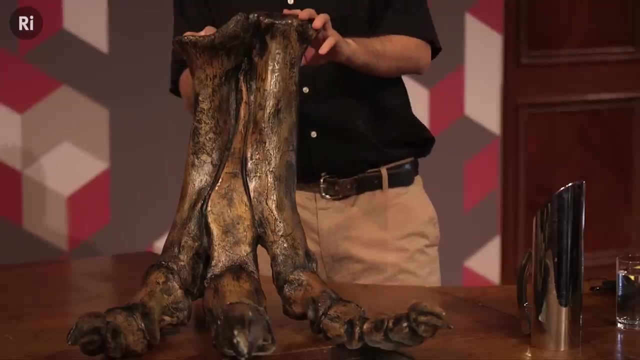 because every little bit of movement is just wasted energy. And if you do this with a lovely, big, wavy bone up the middle with two bones locking it in either side, you're effectively holding the whole foot together. And when we're talking about an animal, that might be six or so tonnes. 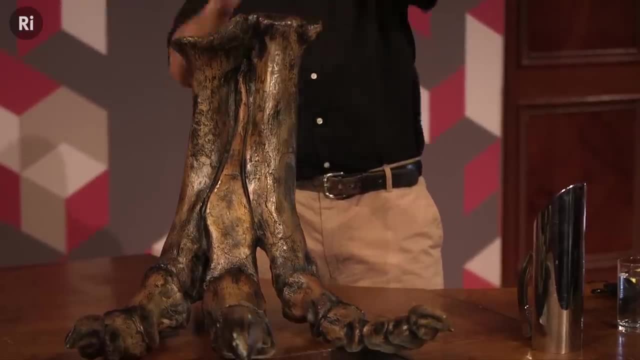 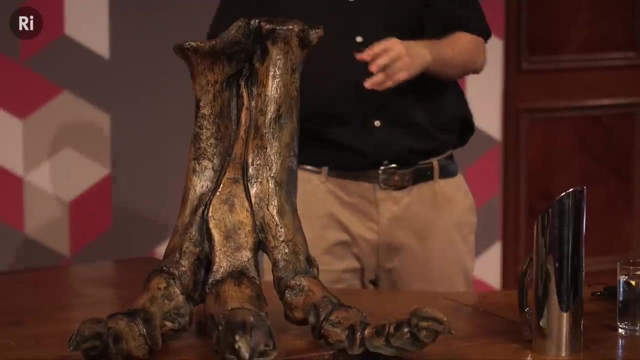 every single footstep can potentially lose a lot of energy, with the bones just see-sawing either side of each other and you're having to hold them together. If you lock them up into a single block, that doesn't happen. Some of that energy will then go into your joints. 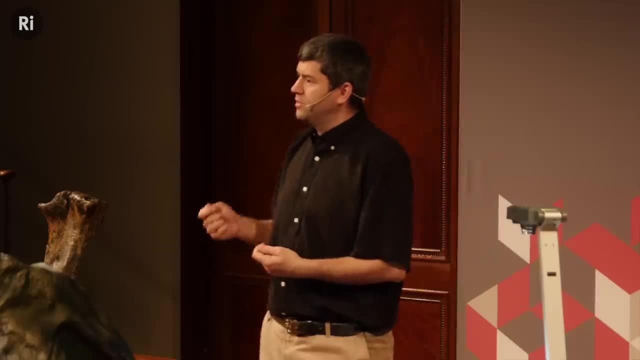 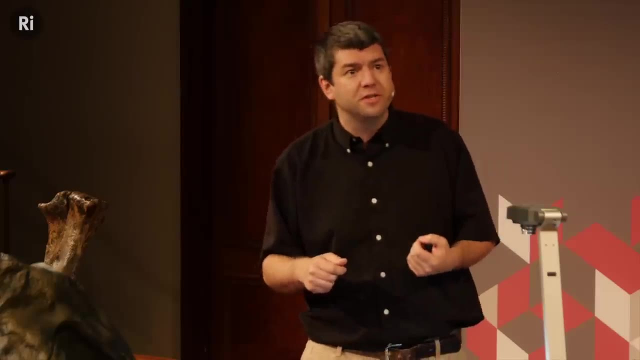 and you'll get it back on the next step. And so this is an adaptation that we see in three or four groups of joints of dinosaurs, and they're all long-distance runners. They're all very efficient over long distances. They usually have very long legs, a light build. 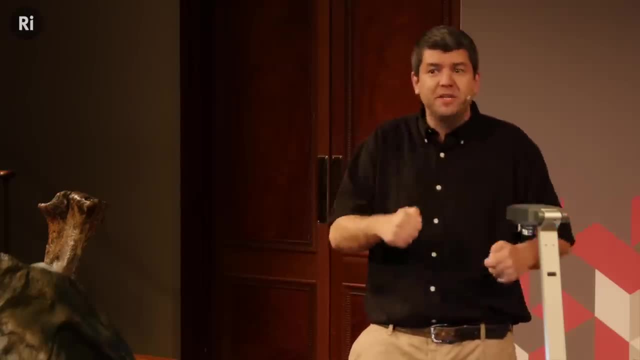 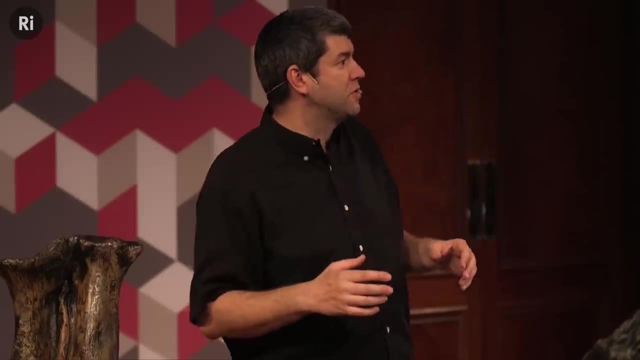 they have a relatively short thigh bone, which allows them to move the legs repeatedly, and that makes them both quick and efficient over long distances. So, despite the fact that a full-sized Tyrannosaurus was clearly a very bulky animal, they were also pretty fast. The speed estimates are really difficult for an animal that's been dead for 65 million years, for which we have no muscles, But bearing all of that in mind, something like a full-sized Tyrannosaurus was probably reaching speeds comparable to an Olympic sprinter. 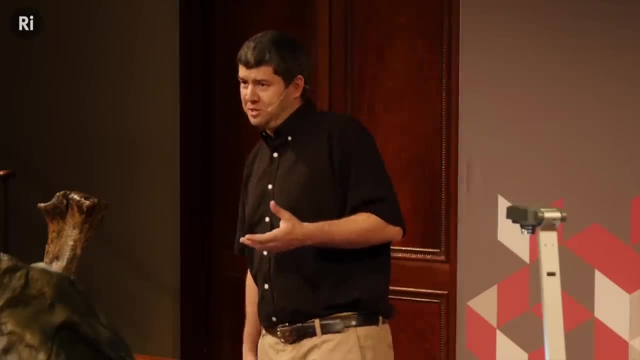 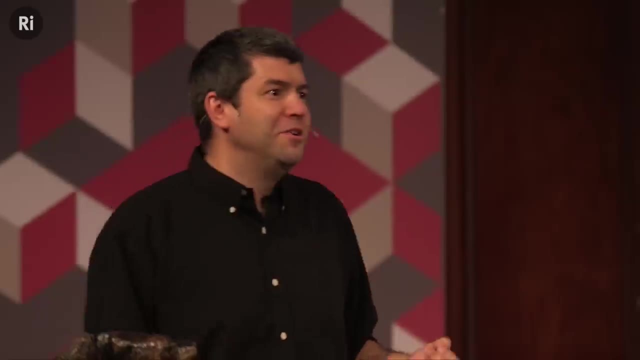 Only the difference is this is an animal which isn't specialised for sprinting, it's specialised for long-distance running, So it's holding that speed probably for quite a considerable period of time. You could not outrun this animal. No chance, Not even beginning to. 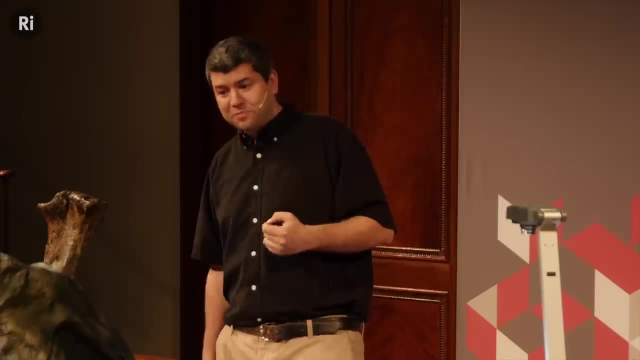 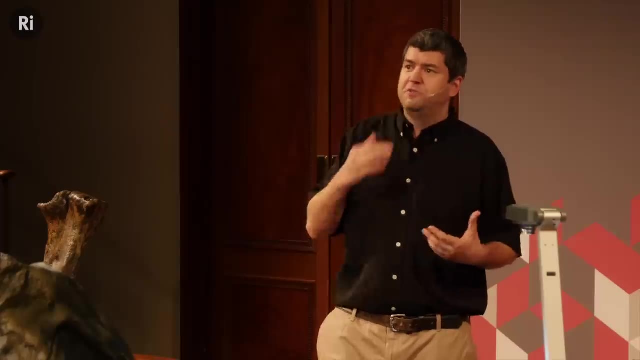 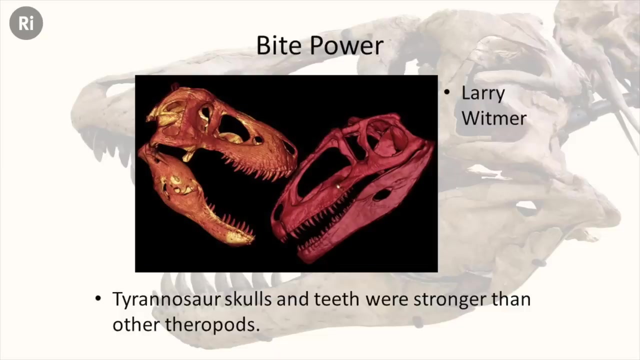 And you also couldn't hide, because it could see you very well as well. This is a really really effective animal, And more so than that: it's really really effective because of the way its skull is built. So here we have some beautiful CT scans of a pair of skulls. 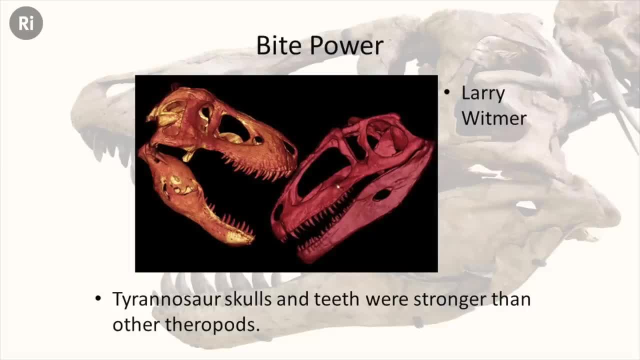 of very, very large dinosaurs. Indeed on the left, once again, we have a Tyrannosaurus and on the right we have this huge carnivore from South America called Giganotosaurus. As you can see, they're scaled to the same size. 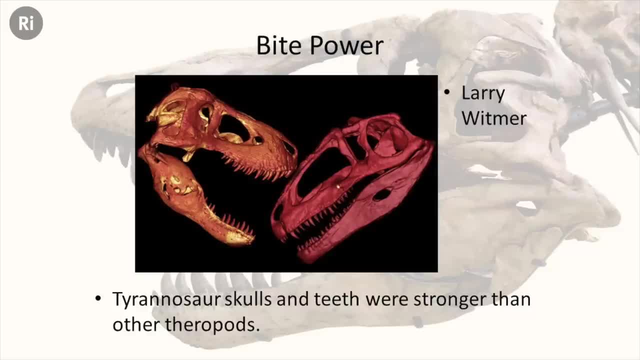 In fact, they're not scaled to the same size. they are the same size. Giganotosaurus has a skull about the same size as Tyrannosaurus, But look at the difference in the amount of bone which is present in each of them. 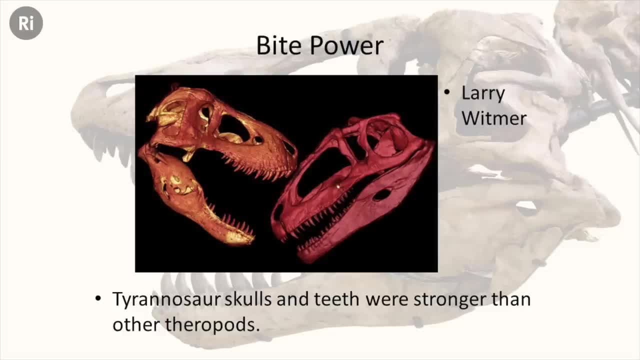 Tyrannosaurus is basically this solid block. Yes, it's got some holes in it, but there's a huge amount of bone here and the lower jaw is almost entirely solid. Compare that to Giganotosaurus, with this really thin lower jaw. 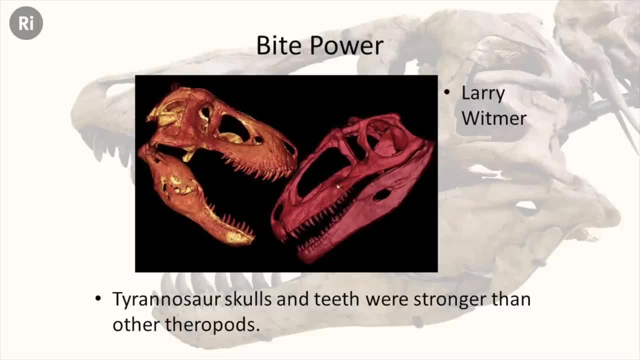 with a large hole in it, This huge anterior hole in the skull, and a very large one at the back as well. There's not a lot of bone there. it's really quite thin in places, Despite the fact that this is a huge and powerful animal. 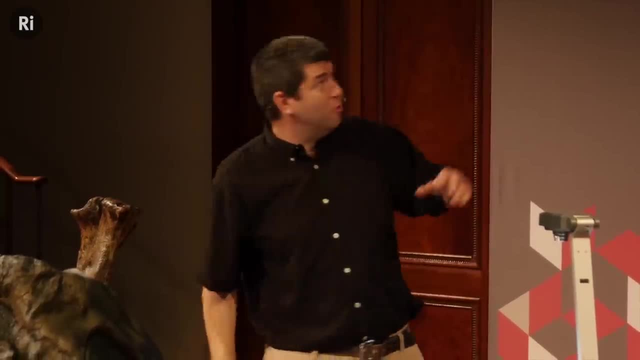 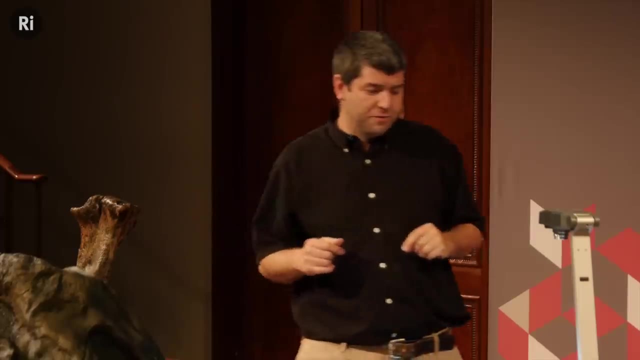 it has nothing like the build of a Tyrannosaurus. It also doesn't have the fused nasals which help make the skull even stronger, and it also doesn't have the teeth. If we can switch back to the viewer again, I've shown you the little teeth at the front. 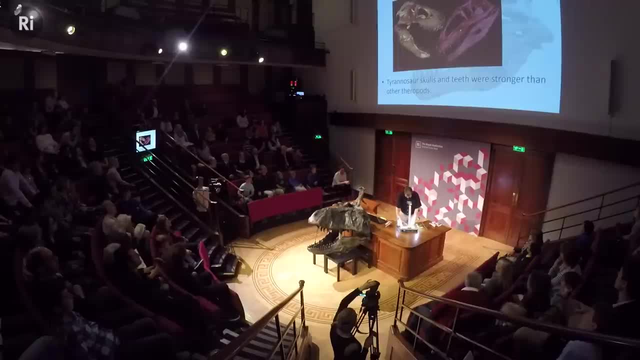 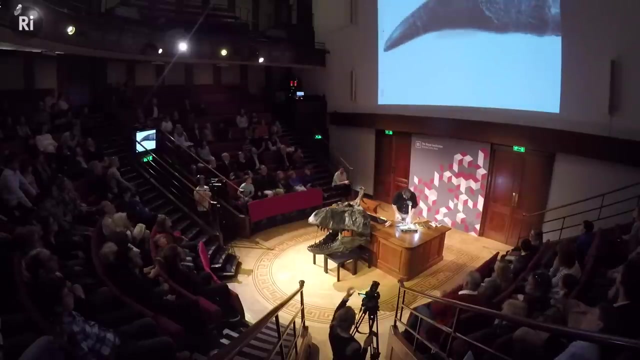 but now let's have a look at the big killing teeth down the side. So this is a maxillary tooth, so one of the big teeth down the side. Oh sorry, can we flick up? Lovely, thank you. So here is one of the big teeth, so this would be down the side of the jaw. 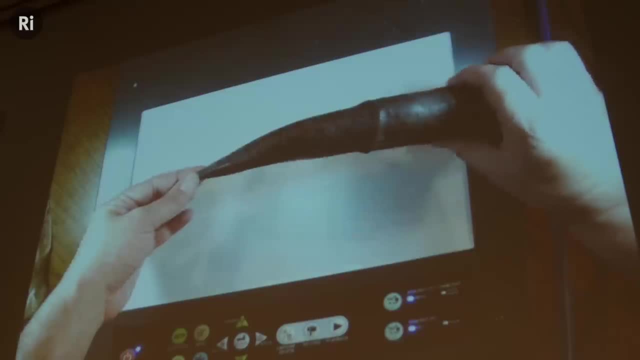 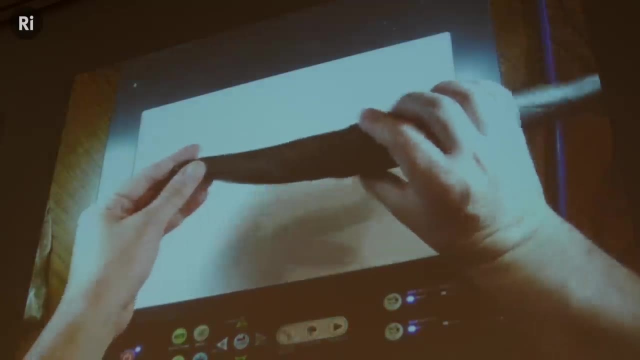 and look at this thing. It's absolutely solid. This is the crown, here again with a very large root. It's absolutely solid. It's almost circular in cross-section, It's nearly as wide as it is long And again, if we compare this, this is a Carcharodontosaur. 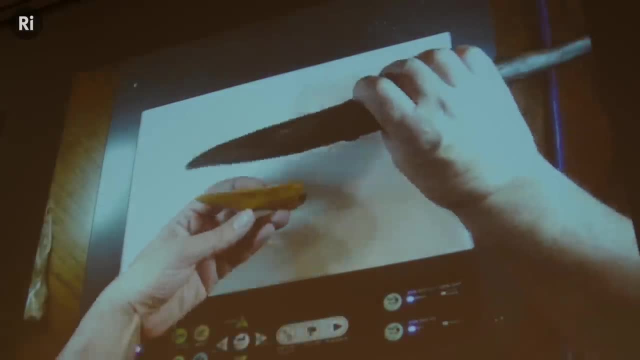 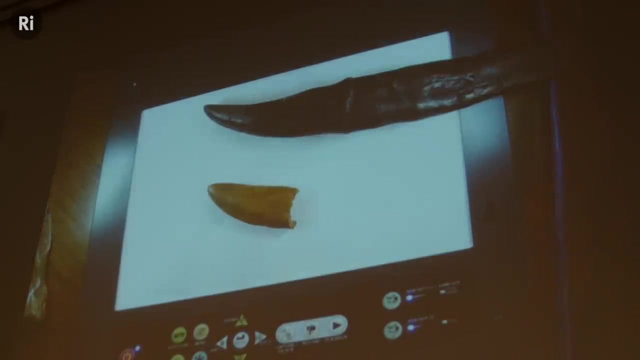 It is from a slightly smaller dinosaur, but there's the comparative width. It is a fraction of the width And, of course, if you make something much, much thicker, you're going to make it much, much stronger. So this is a tooth which is extremely powerful. 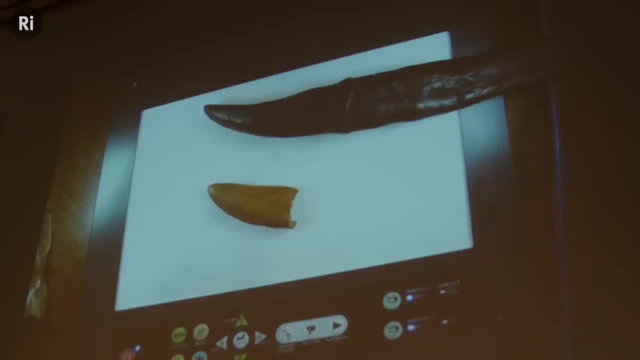 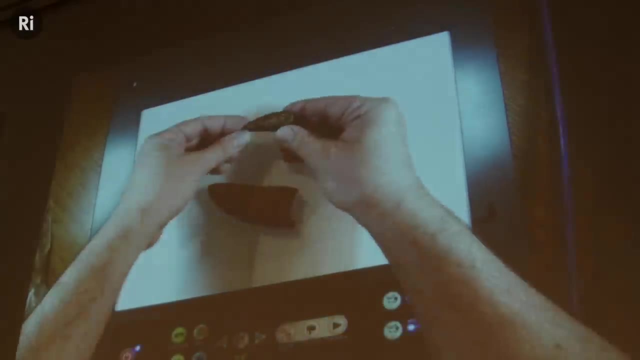 perfectly capable of biting Very deep and very hard into things, even very, very hard things I actually have. sadly, it's only the tip, but I actually have a real Tyrannosaur tooth here. Again, this is on loan from the Tyrrell Museum. 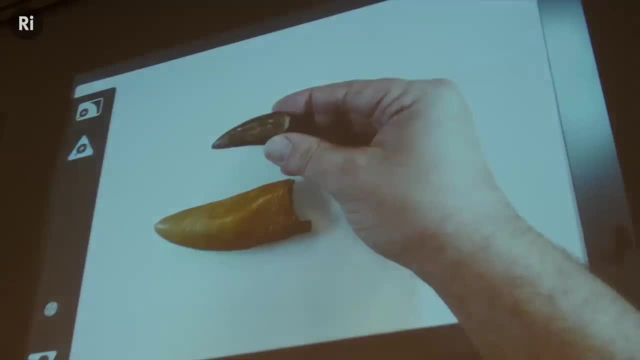 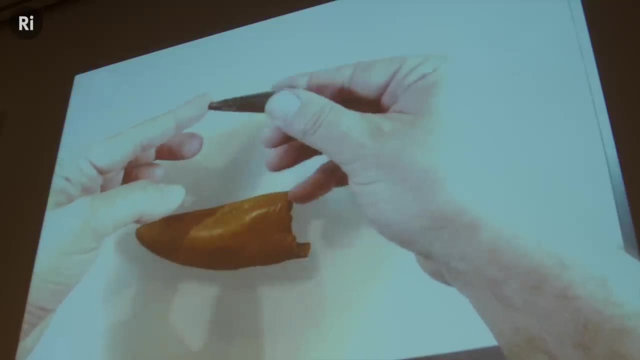 If we can just zoom in a bit, There we go, lovely. So it's just the tip. This is probably from a Gorgosaurus from Alberta. This was found by one of my students last year when we were out in Canada. 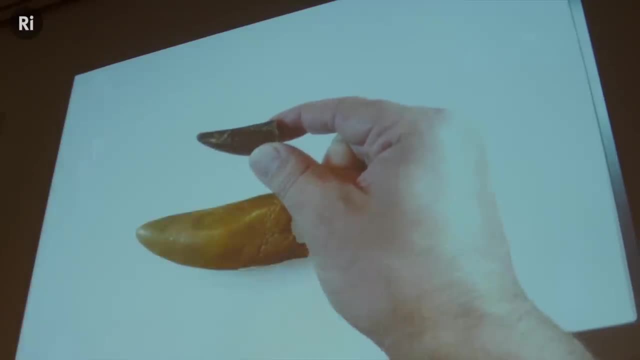 And you can still see there's actually a little line of serrations along the back. So even though this is a Carcharodontosaur, it's not a Carcharodontosaur Even though they have this enormous kind of puncturing tooth. 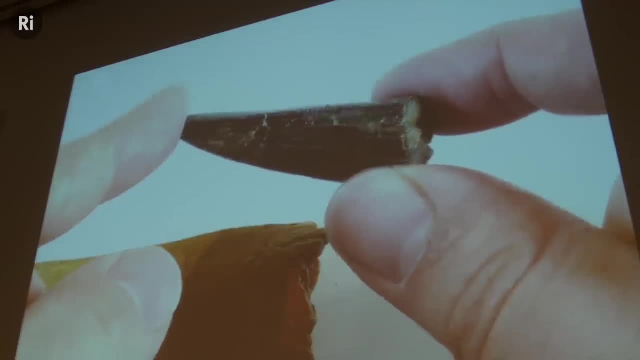 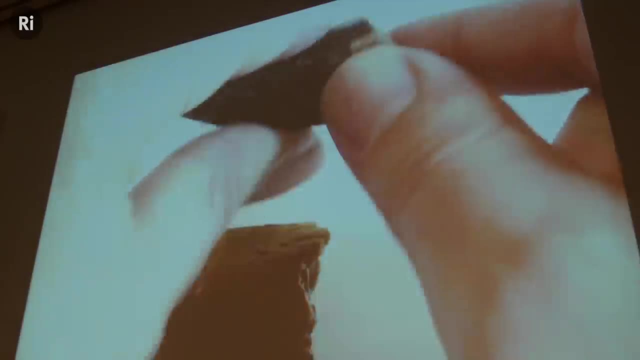 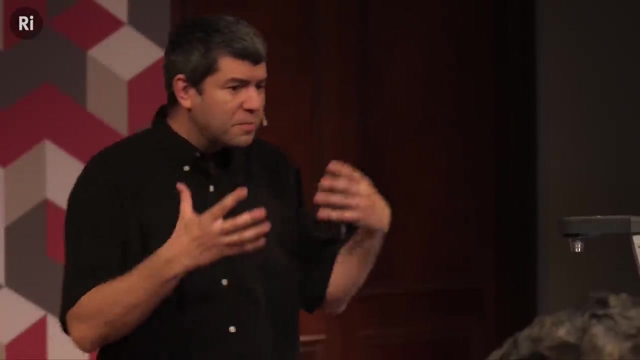 they do still have a lovely little train of serrations along the back. So there is still a cutting edge front and rear. And again, look at the cross section Very, very round. This is an extremely solid and powerful tooth. So we have a super large skull in the big animals. They have super large teeth And they're well built, with lots of bone and various fused parts to give them enormous strength, And when you add that together, you get an animal with colossal bite power, more so than any other dinosaur that we know of. 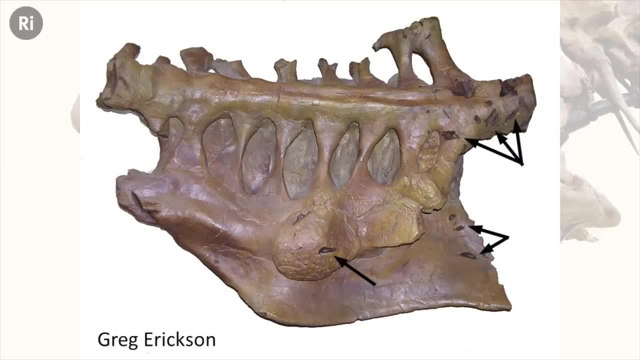 And then you start seeing things like this. This may not look like very much, In fact, it all looks like a bit of a mess, But this is most of a Triceratops pelvis. We're looking at it from underneath as if the animal was lying on its back. 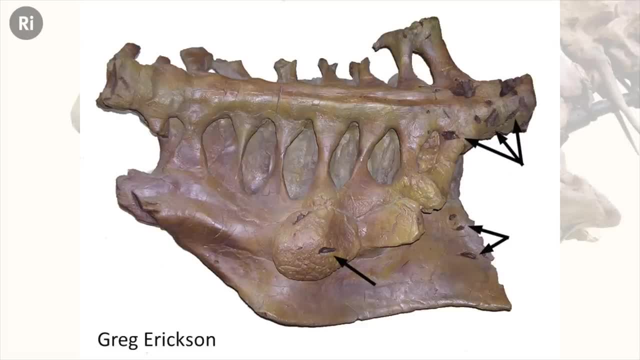 We've only got about half of it, So here would be the backbone, Here are various extensions, And then the major part of the pelvis is here, And then the major part of the pelvis is here. For a start, a fairly large part of this is missing. 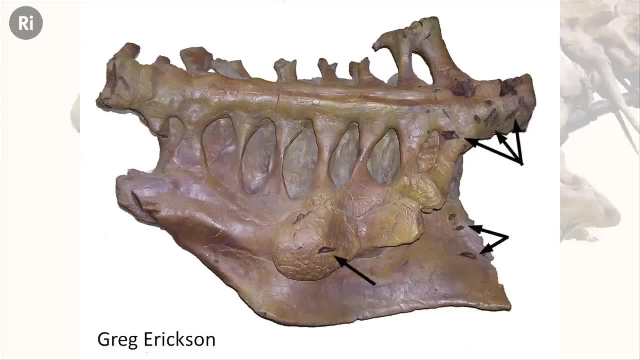 And it's missing in a rather suspicious way because it's got a kind of little serrated edge to it, Almost as if five or six big, very strong, powerful bitey things had knocked a hole in it and broken the end off. 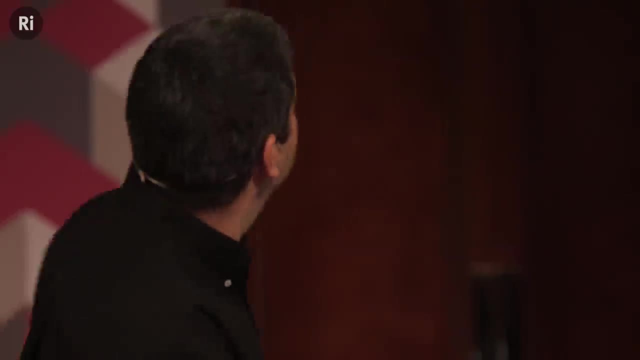 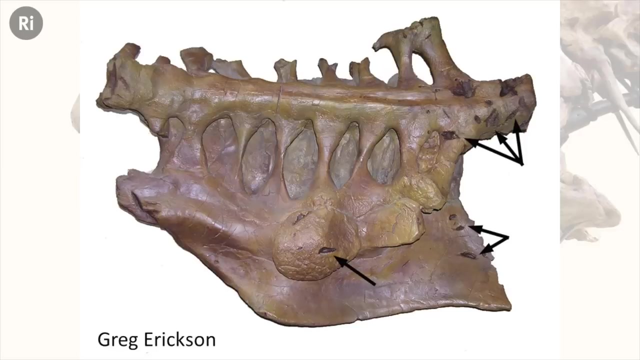 You can guess what that might have been. More so it's got a whole load of holes and gouges and grooves in it, All of which are suspiciously very, very broad compared to their length. In other words, they look an awful lot like the cross-sectional shape of a Tyrannosaurus. 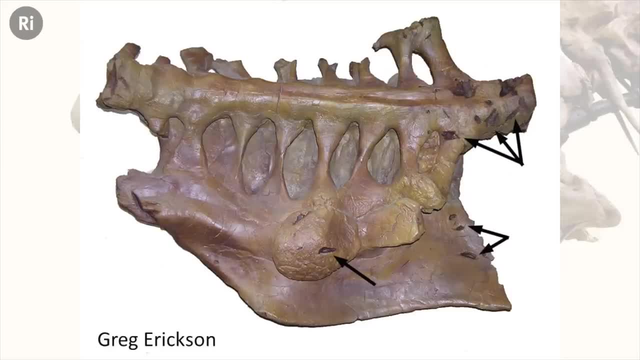 And, in fact, the researchers. this is a photo from Greg Erickson in Florida. they actually took some lovely liquid rubber cement- the kind that the dentist used to take a mould of your teeth- and they poured it into those holes And when you pull it out it's almost a perfect copy of a Tyrannosaur tooth. 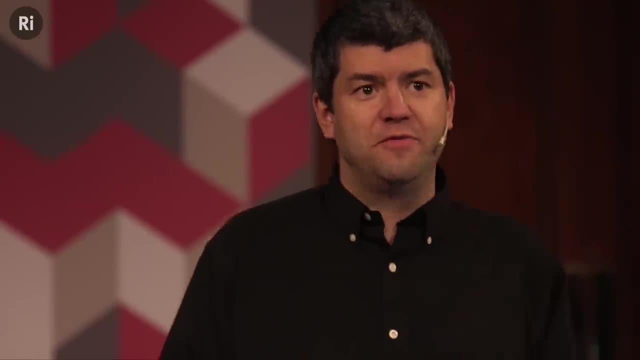 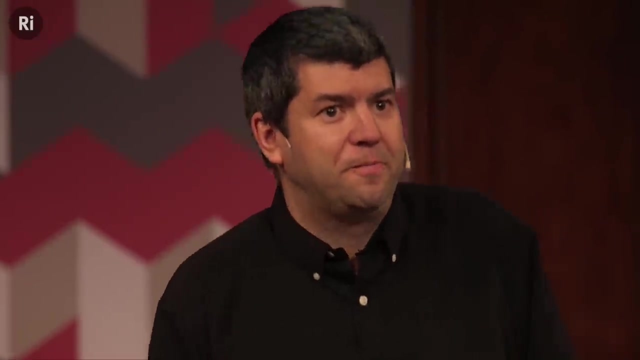 Their teeth are not just capable of biting deep into bones and leaving huge holes in them. They're so good at it. they actually leave a mould of their tooth behind in a lump of solid bone. This is an extraordinarily powerful animal in terms of its bite power. 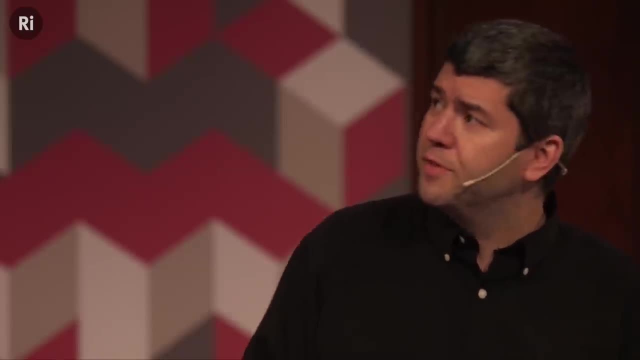 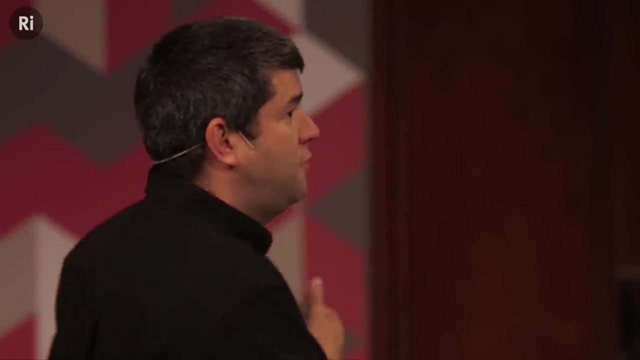 And this is an adaptation that we do not see in any other animal, which is really quite nice. Now there's a really interesting aside to this study, which is trying to infer what the animal was doing. There was a famous debate, which I really wish we had. 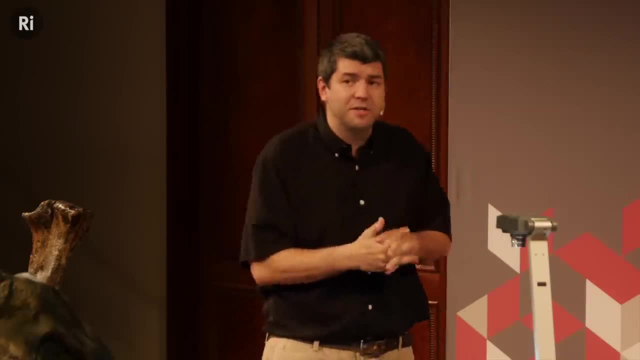 which I really wish we had, which I really wish we had, which I really wish would be over, but if it isn't over already, I hope to demonstrate it- as to whether or not Tyrannosaurus and the Tyrannosaurs generally were predators or scavengers. 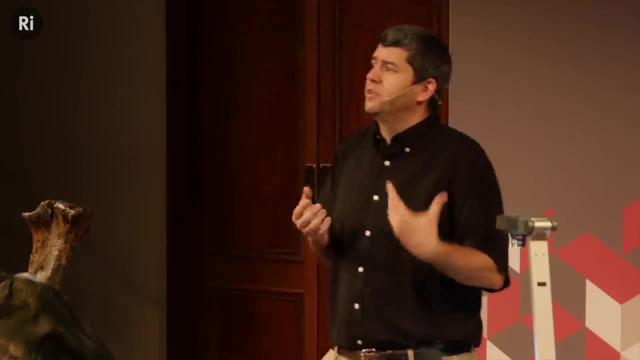 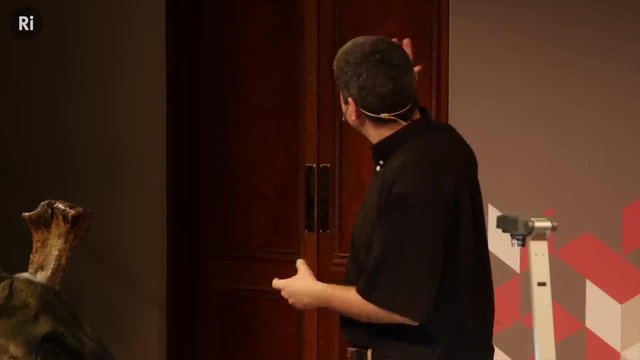 Now this is very actually hard to show because obviously seeing and identifying those kinds of behaviours in the fossil record is very, very difficult. It's very hard to come up with any evidence which will show it either way, And Greg and his colleagues suggested that this may have been a scavenging event. 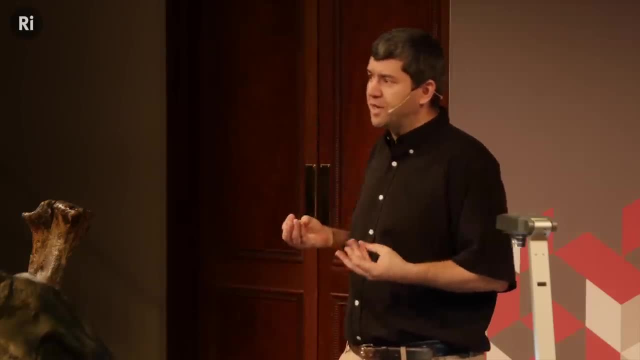 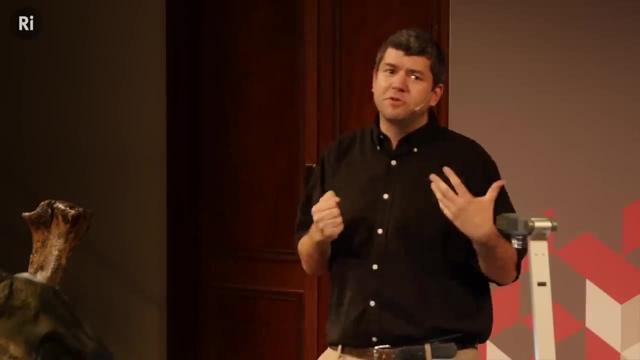 Animals don't usually chew apart a very old pelvis unless there's not a lot of food going and that kind of implies that it was perhaps scavenging. But it's very difficult to demonstrate that this might actually be the case. It certainly could have been and I think it's quite likely. but it's also true that things like leopards, if they manage to kill a large antelope, they'll spend several days eating on it and by the end they will be chewing on the last little leftover bits. And that's not scavenging. it's just taken them a long time to get through it. 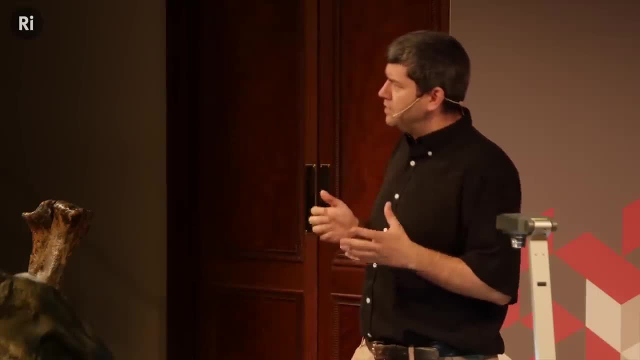 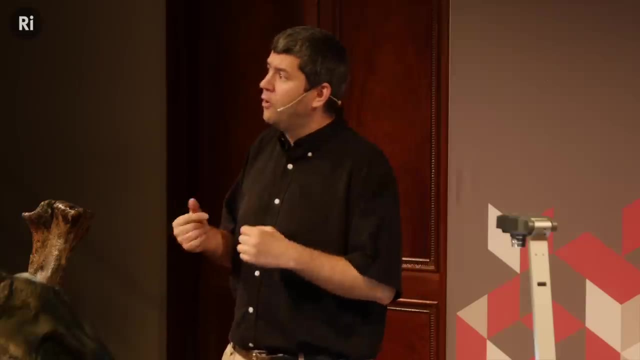 What you'd really need to try and demonstrate. that is, in fact, some kind of very special specimen where you could tell what the history of the dinosaur was before the tyrannosaur got to it, And I was lucky enough to be given the opportunity to work on one such specimen. 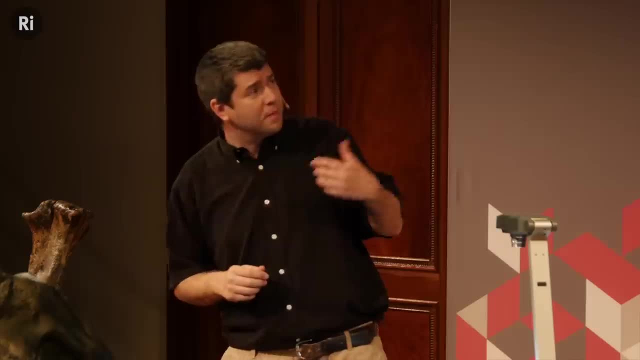 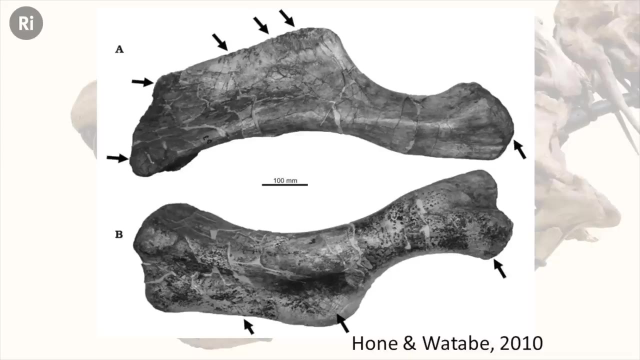 back in 2010 with my colleague, Mahito Watabe in Japan. This specimen is actually from Mongolia, though it's held in Japan, and it's the humerus or the upper arm bone of a hadrosaur, one of the duck-billed dinosaurs. 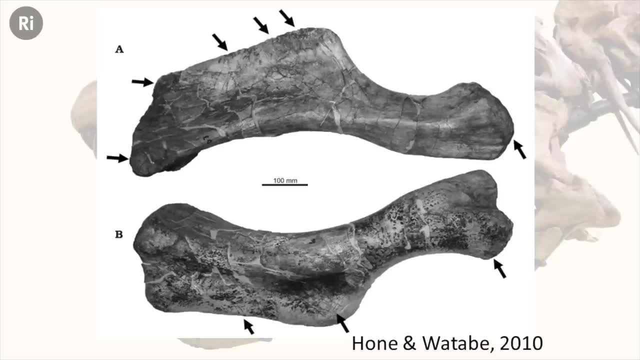 And what all these black arrows point to is various different bite marks along it. In fact, this thing has been extremely well bitten by a large tyrannosaur, and this would be a thing called Tarbosaurus, which lived in the late Cretaceous of Mongolia and North China. 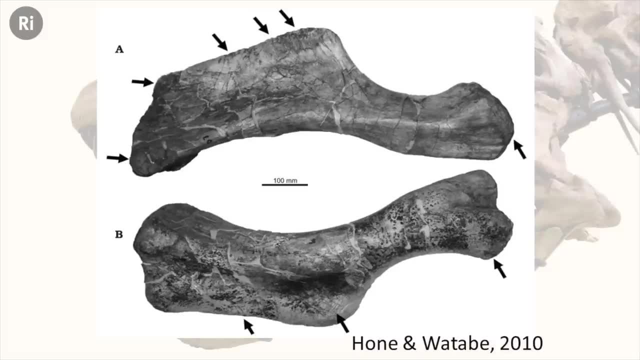 So there are big deep bites at each end, and then this big flange of bone along the front here has groove after groove after groove after groove stored in it. You can't see it too clearly there, but if we go to this close-up. 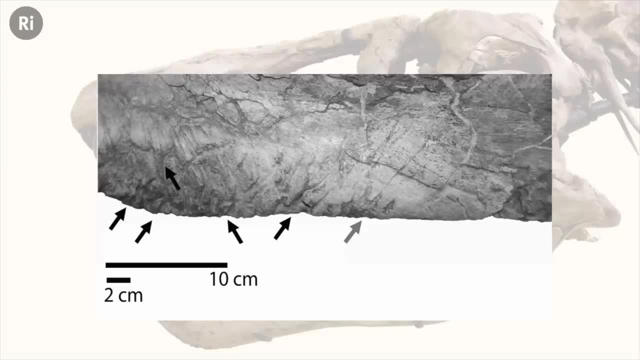 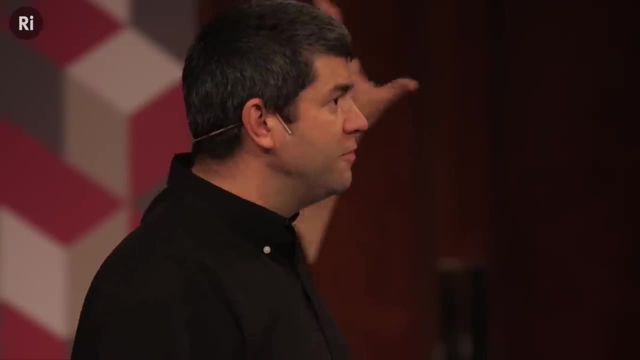 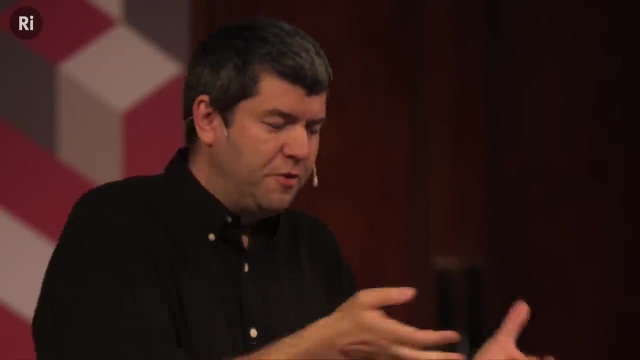 But they're also quite distinctive because, although this is clearly a very large animal, we're lucky with some of the big tyrannosaurs that often they're the only large carnivore in their environment. If you find a bone in Africa with a whole bunch of big bites on it, from a large carnivore. it's often hard to say: was that a lion or a leopard or a cheetah, or was it a hunting dog or one of the various species of hyena? With tyrannosaurs, you've often only got tyrannosaurs around. 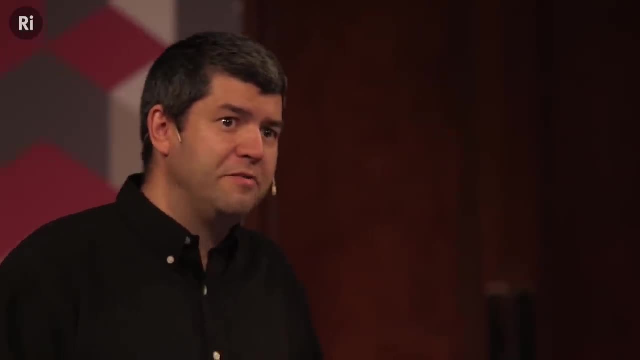 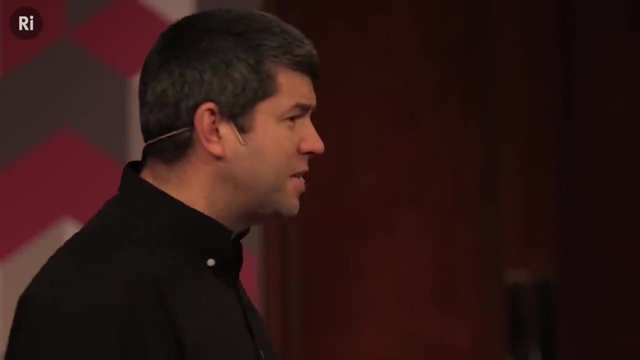 so you kind of know what did the bite, even if you have no direct evidence. And yet, even though these are very strong and powerful bites that have gone into the bone, the teeth don't appear to be that big and they're also really really close together. 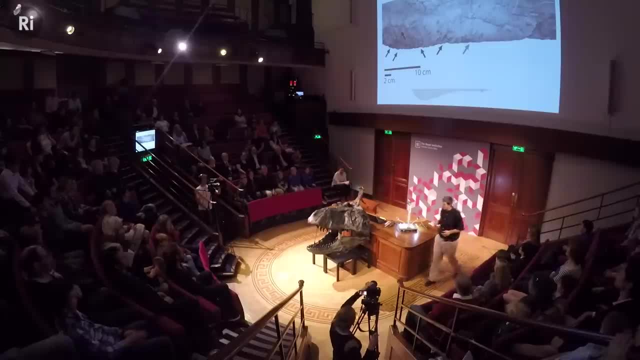 And this takes us all the way back to our defining characteristic of tyrannosaurs. They have this little cluster of teeth at the front. They're all the same length, They're all very close to each other and they're all really quite strong and solid. 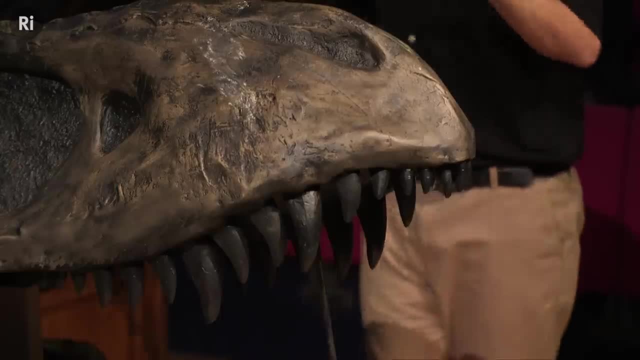 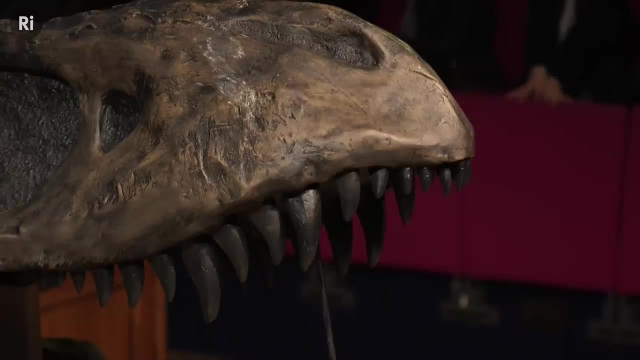 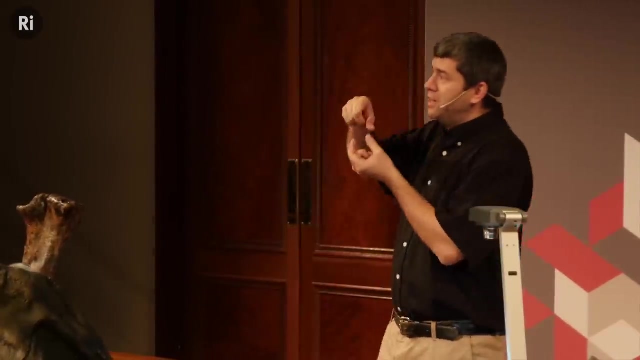 and with these little flat backs, And this is going to be perfect for grinding across the surface of a bone. I suspect that everyone in this audience has at some time taken a custard cream or a bourbon biscuit and you take the top one off. 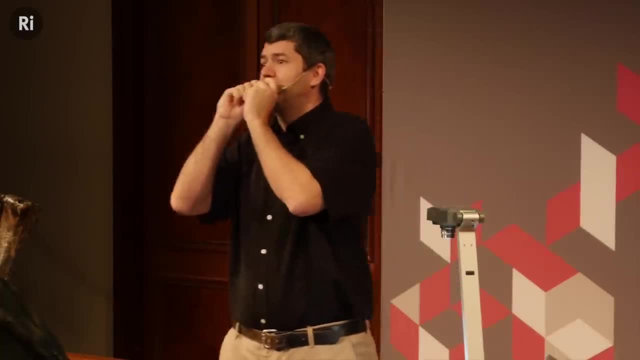 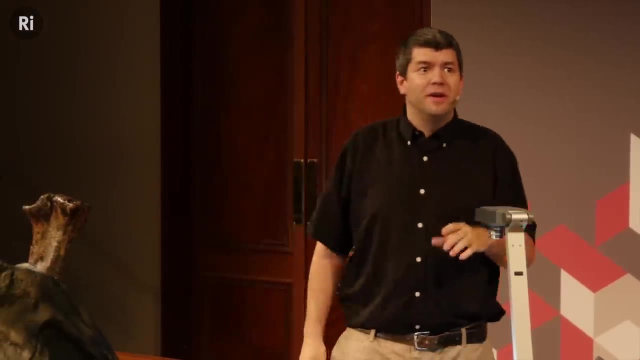 Yes, we all know this is going. And you put it in your mouth and then you scrape the cream off. Yep, That's what tyrannosaurs are doing, And I know that's what they're doing, because the interesting thing is: 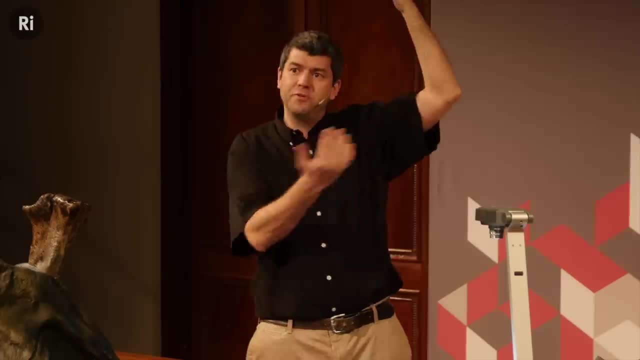 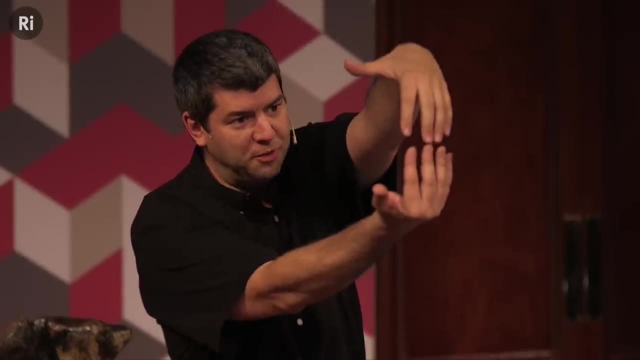 if you flip this bone over, the bites on the underside aren't in the same direction as the ones on the top. So it is not biting top and bottom together and pulling, because if it was, all of the marks would line up. 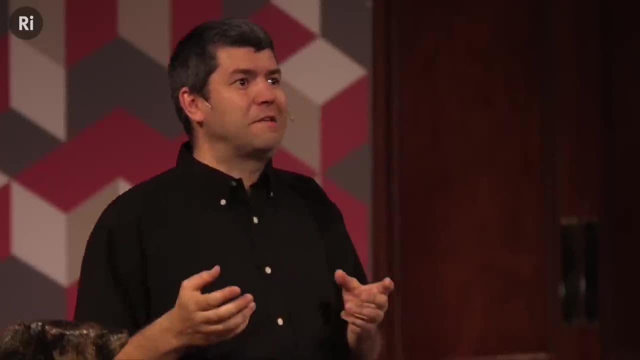 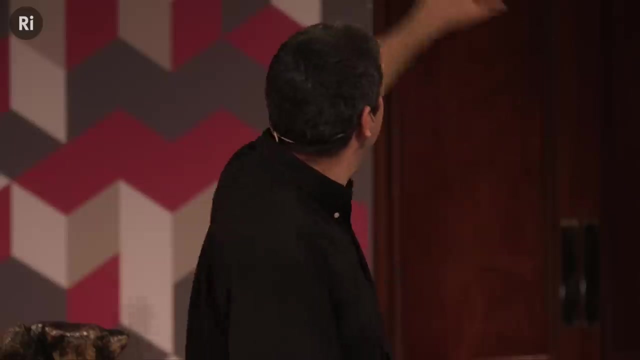 They go in different directions, And tyrannosaurs are not like us. They can't move their jaws like this. They can only go up and down, So they're just using the upper teeth, And that's why you get this very distinctive set of marks that are large. 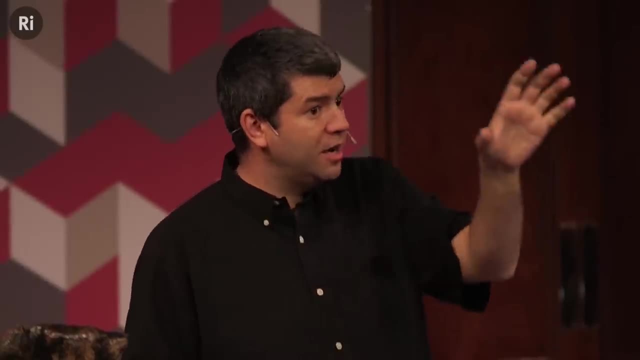 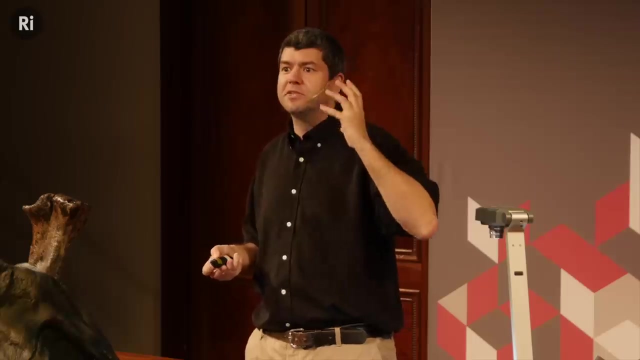 showing the teeth are large, but they're very close together And they're all the same depth, Whereas if you look along the side of the jaw, all the teeth are different lengths. If they were doing this with the big teeth in the side of the mouth, 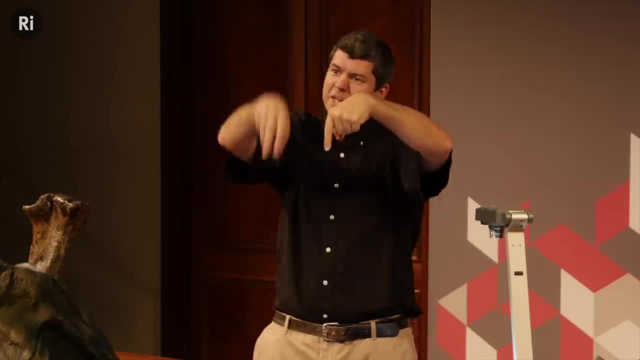 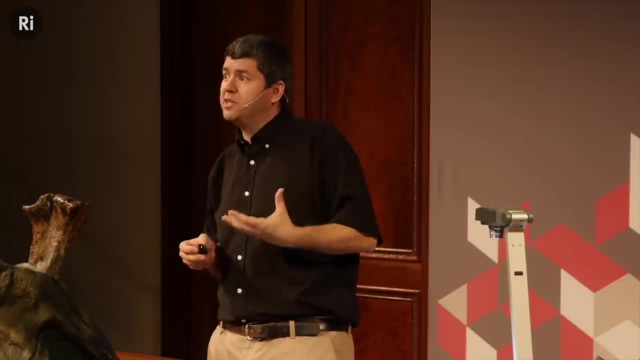 there'd be big spaces between them and one tooth would contact, but then the next one's shorter, so it doesn't do anything. It's only if they're using their upper teeth and drawing it along the surface will you actually get this effect. 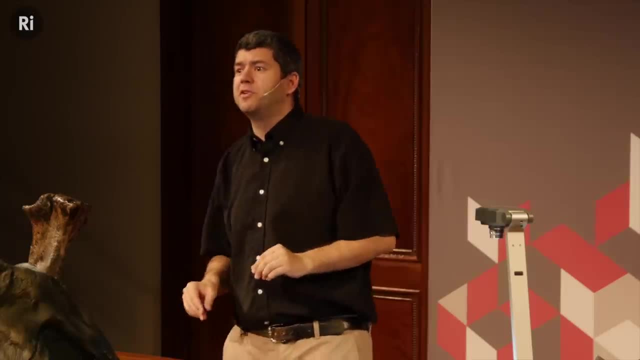 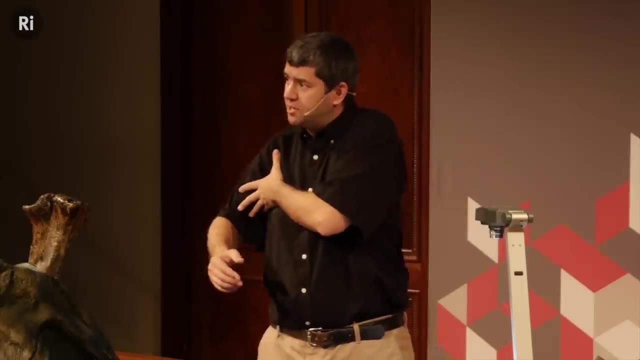 It's also interesting that the only place they do this on the bone, at least on the duckbill, is this part here, which is where all of the big chest muscles attach to the upper arm, And they don't appear on other parts of the bone. 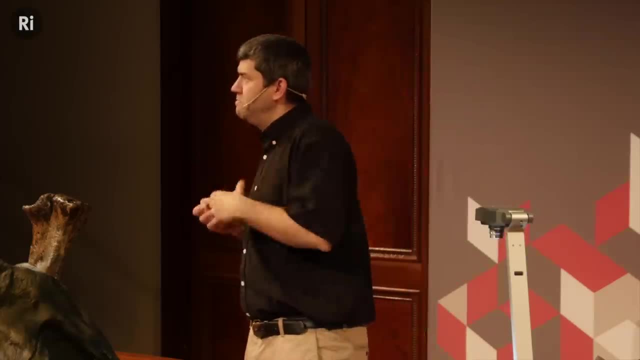 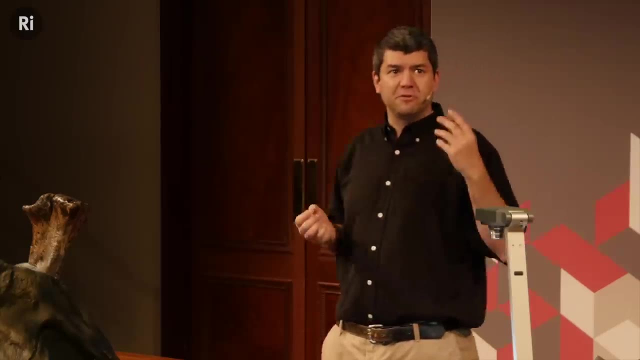 This animal was feeding selectively. It's not some mindless big bone cruncher. It's not like you see crocodiles feeding, where they just tear off big chunks of everything and bash it about and swallow it. This animal only bit in a certain way, on a certain part of the bone. 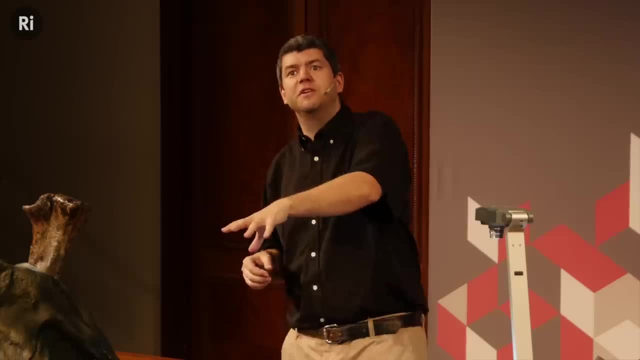 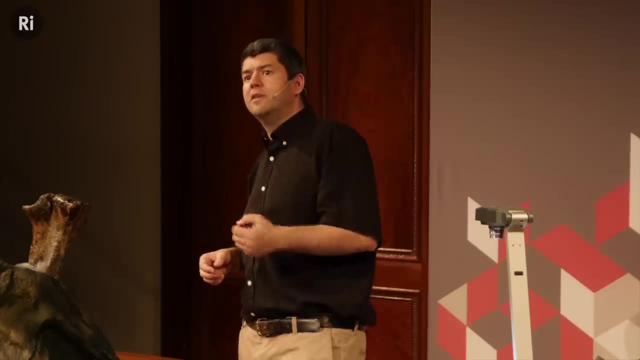 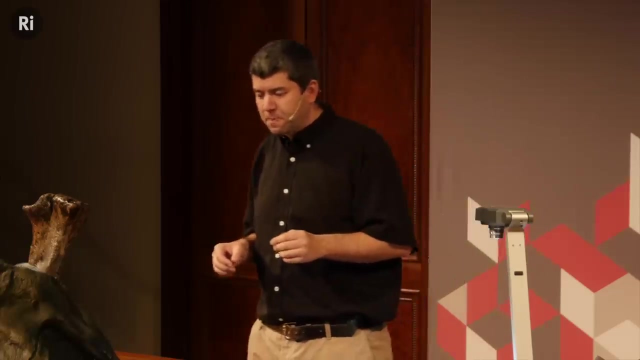 where it could get muscle. This is a very careful feeder. These animals can selectively choose how they bite and where they bite in order to feed, And they have a suite of adaptations in the skull to allow them to do that. They're really quite a specialist animal in lots of ways. 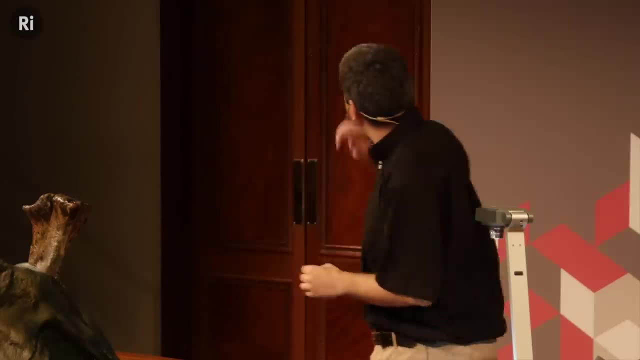 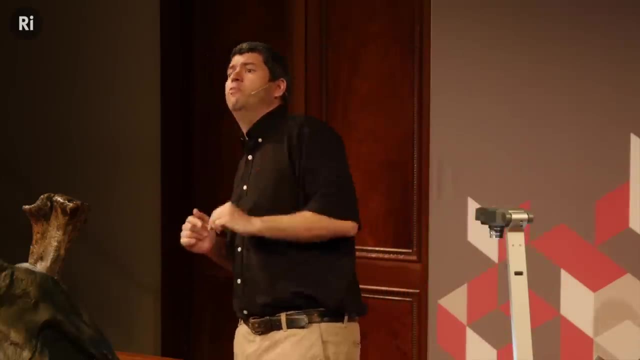 So this really tells us something about their behaviour. But there's another factor to this skeleton as well. I've only shown you this one falling bone, but in fact that hadrosaur is known from an almost complete skeleton. We have the skull, the neck, the ribs, the legs, the tail. 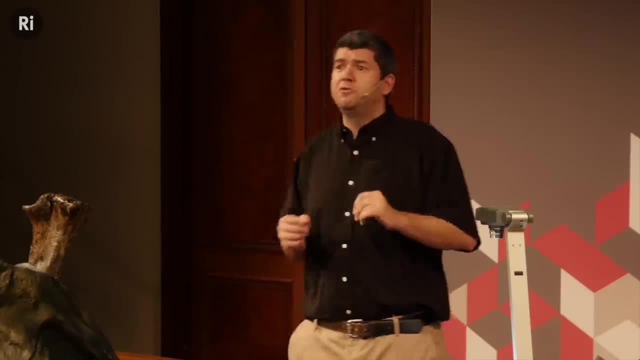 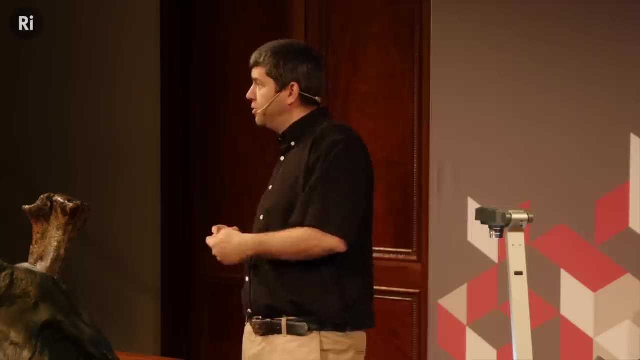 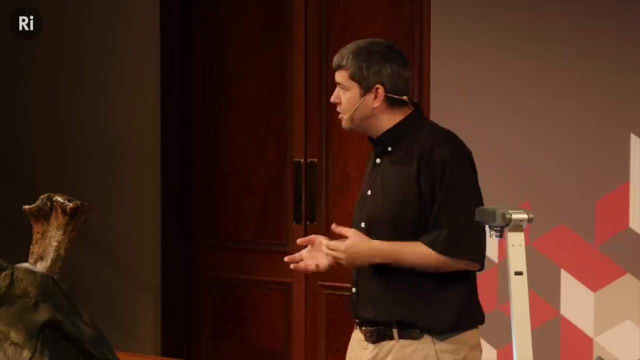 We've even got patches of the original skin preserved. It is in beautiful condition But interestingly, several bits of it show evidence of having been damaged by the skeleton. This is an animal that actually lived most in the desert, but it was found in what we know was a fossil water channel. 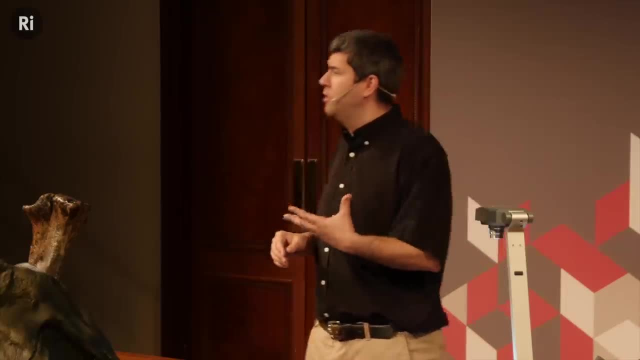 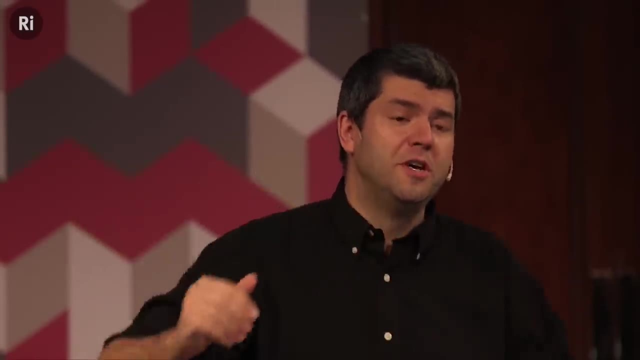 and that had been partially buried, And only one bone of this incomplete skeleton shows the damage, And it's the humerus, but it's also the bone that was sitting uppermost. So this animal was keeled over on its side and only one bone was sat out. 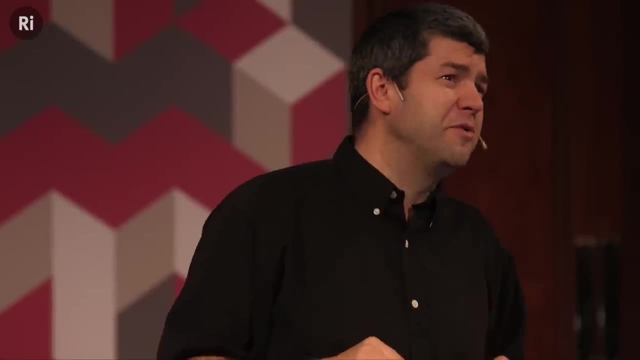 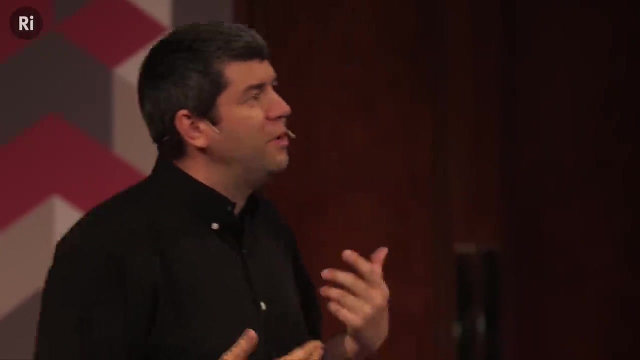 And that bone didn't show much evidence of water damage, but it did show evidence of having kind of been beaten up by wind. They do leave very distinctive traces on the bone. When you combine this information it becomes fairly clear what must have happened. 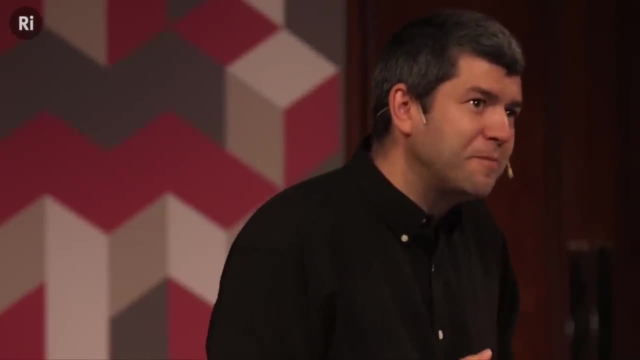 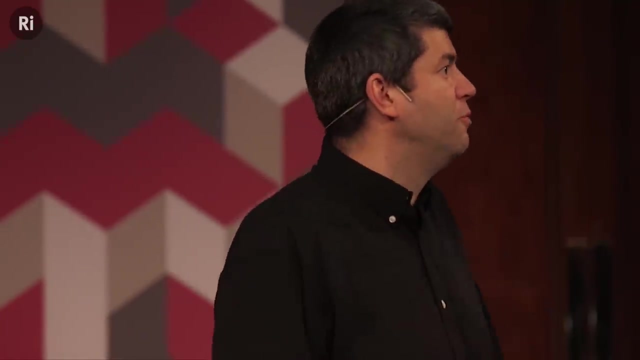 We've seen what a Tyrannosaurus will do to a pelvis if it gets hold of it. So why has it left this entire skeleton, which even has skin left on it? so must have had all the muscles and other tissues attached. 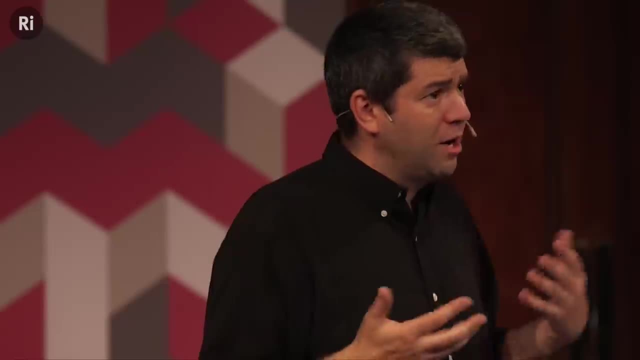 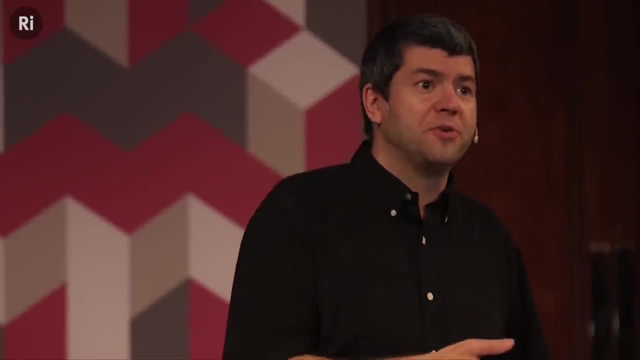 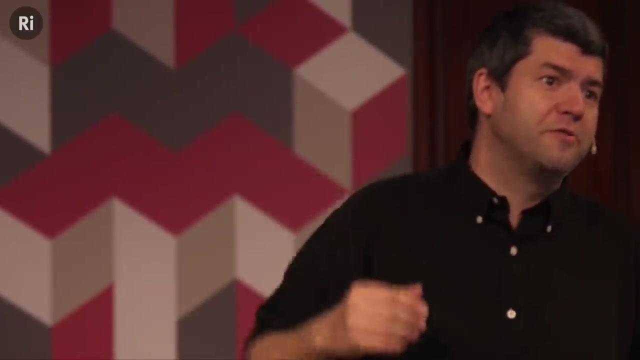 not a bite one bone: 53 bites on it. What happened was this hadrosaur had died somewhere else, perhaps in the water, and drowned, washed downstream onto a sandbank, showing evidence of water transport and damage, then been buried, and only one arm was left on the surface. 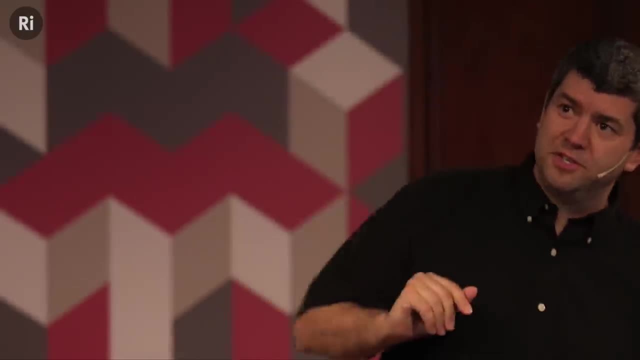 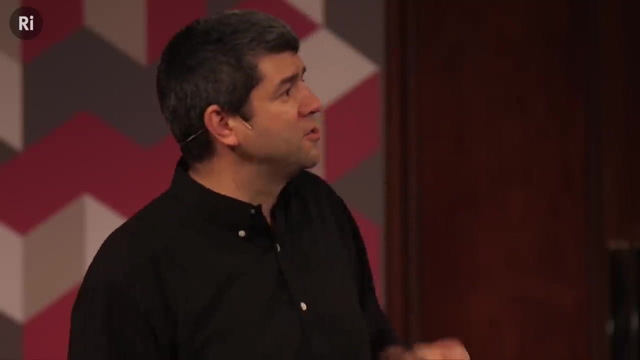 Then a Tyrannosaur fed upon it. So now we know this is scavenging. This animal was scavenged because it was dead before it was bitten, So we can put one thing to bed: Did Tyrannosaurus scavenge things? 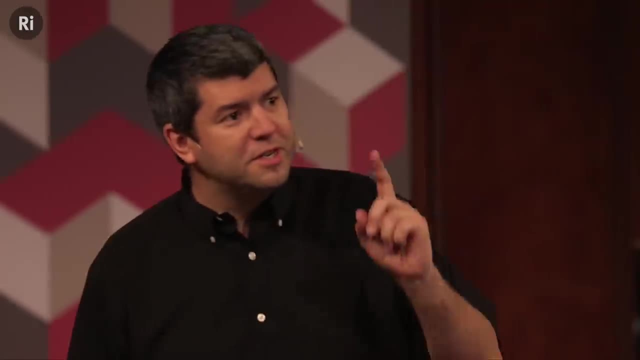 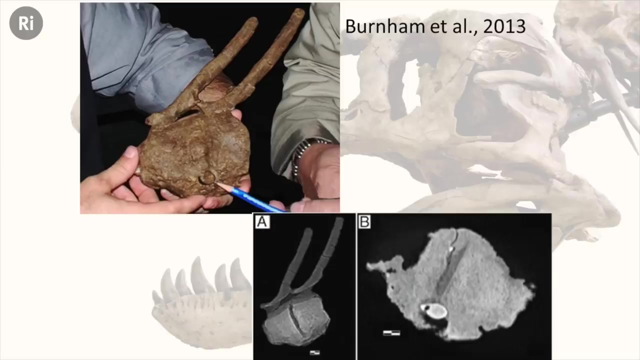 Yes, Excellent. Now the other half. Did they predate on things? Well, here we have yet more hadrosaurs. This time we have a pair of tail vertebrae, so two bones from about halfway down the tail and they fuse together. 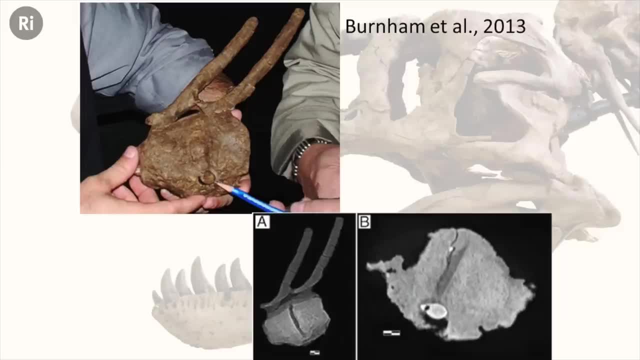 There's a major injury or illness here which has caused the bones to fuse. They're actually really quite common in various dinosaurs. They have lots of little bones in the tail and if you bash them up a bit they tend to form a big lump. 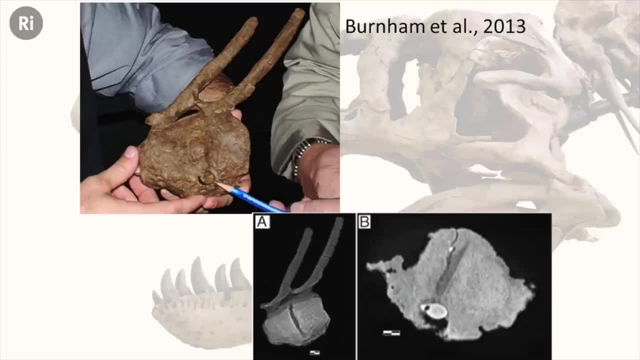 But in this case, as you can see, hopefully, what the pencil is pointing to is a weird nodule in the middle. that's a bit of a funny shape, And so they x-rayed this, And when you x-ray it, first of all, you can see the original join. 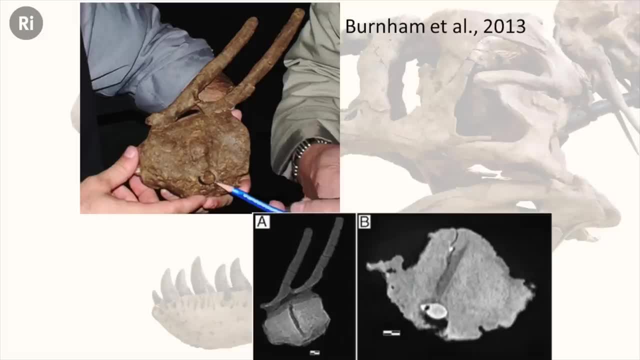 which is now sealed up between the two bones. But then you can also see something which is a very different density to the rest of the bone, because it's a different colour and also has a fairly distinctive shape. It's a shape we've all seen. 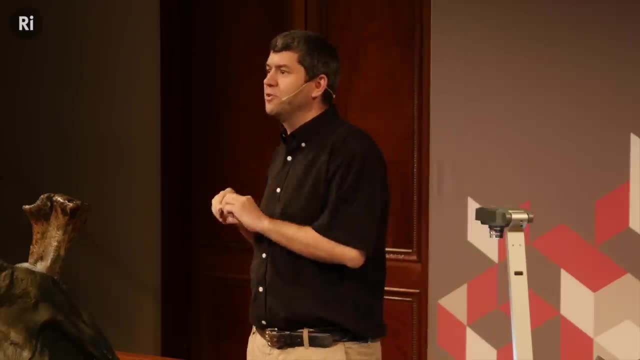 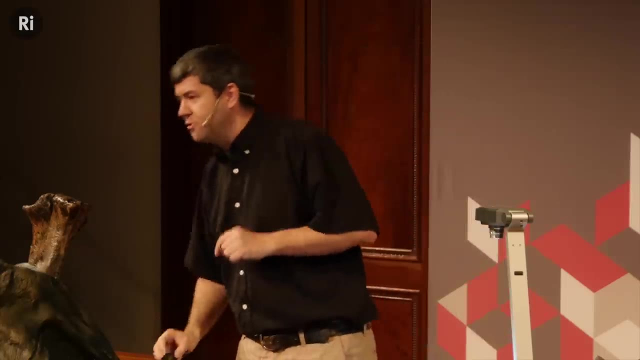 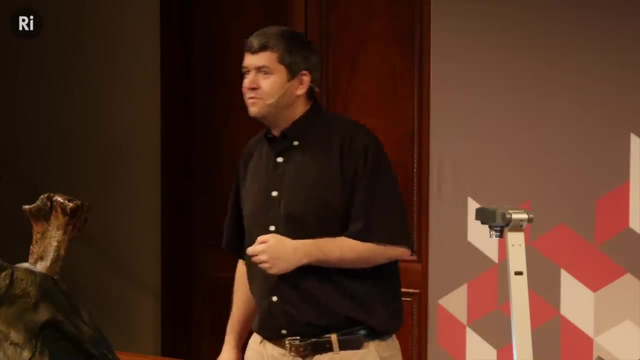 before it's the cross-sectional shape of a Tyrannosaurus tooth, which is nearly as thick as it is long and slightly tapering at the back. That's a Tyrannosaurus tooth which is inside the bone and the bone has grown over it. 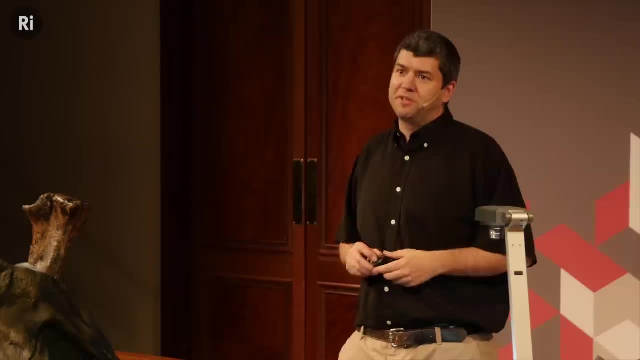 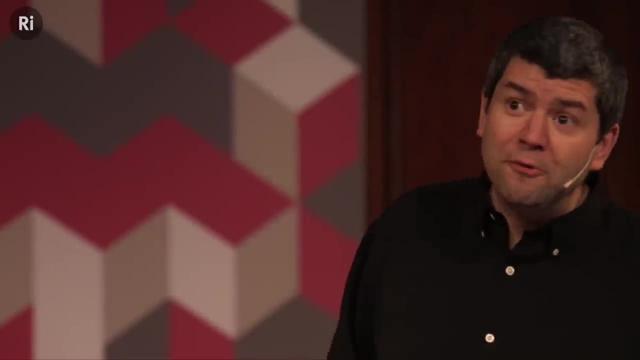 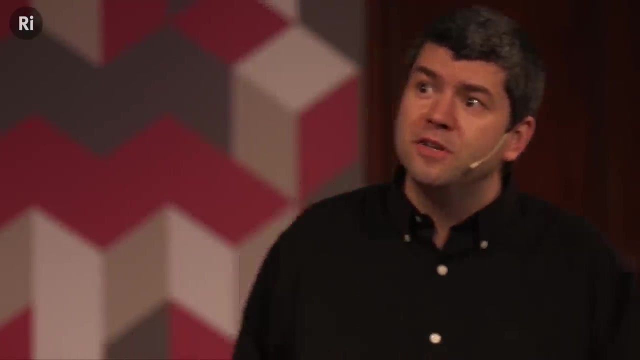 That takes days, maybe weeks, possibly months to happen. This was a hadrosaur that a Tyrannosaur bit into it, pulled a tooth out and left it, presumably because it got away And over time it healed. it was a nasty wound. 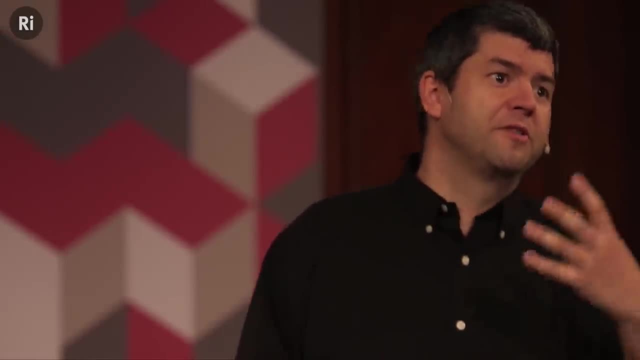 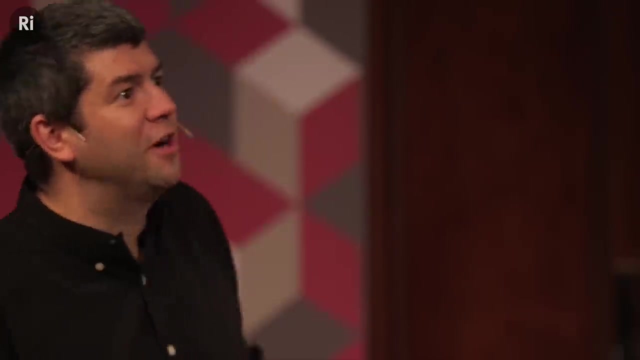 lots of new bone form to try and heal up that wound, and one of the things that it did was cover the tooth. Now, technically that's not a predation event, because clearly it survived, but I think you'd be hard-pushed to come up with many other explanations. 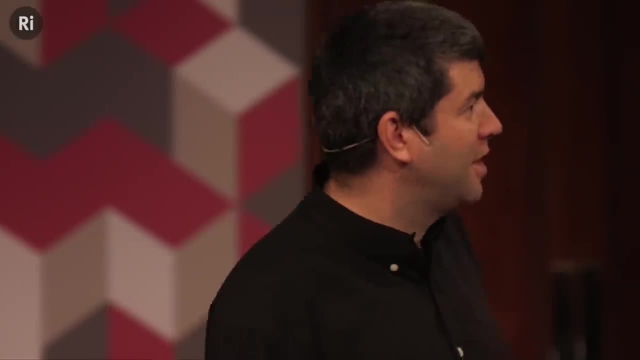 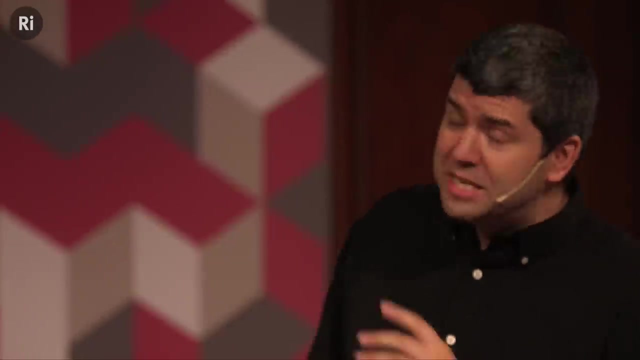 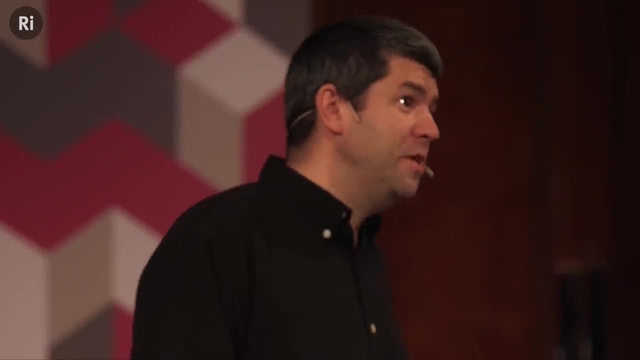 for why a herbivorous dinosaur had the tooth of a Tyrannosaur jammed into its tail. This also isn't the only specimen we have like this. There's actually another specimen which has a Tyrannosaur tooth embedded in the lower leg. 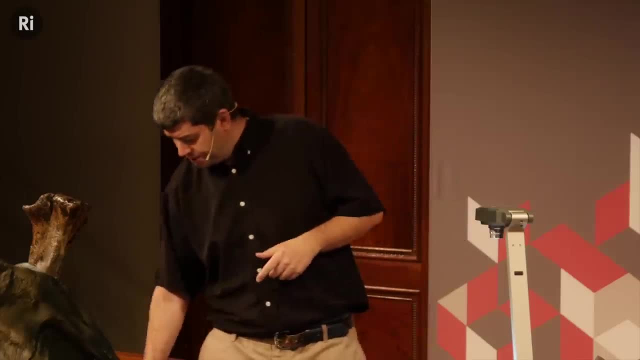 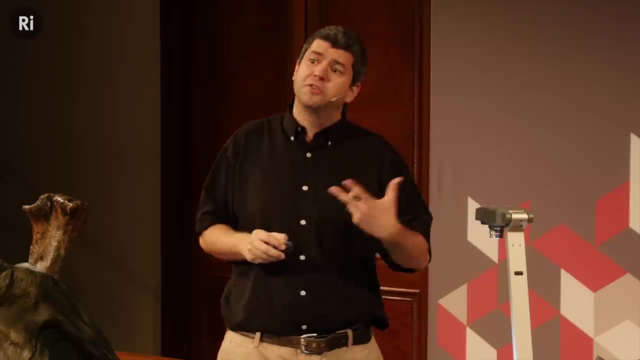 and there's yet another hadrosaur, which has one of its tail vertebrae, has the top broken off in a pattern which is very suspiciously similar to the shape that we saw in the Triceratops pelvis. So, in other words, it looks like it's been bitten through. So we have three different instances here where it looks like a Tyrannosaur has bitten a herbivore and that herbivore has escaped. But I really think we can fairly convincingly call this predation. So were Tyrannosaurs scavengers? Yes. 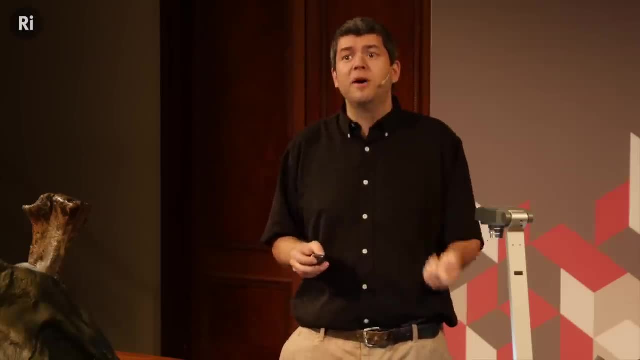 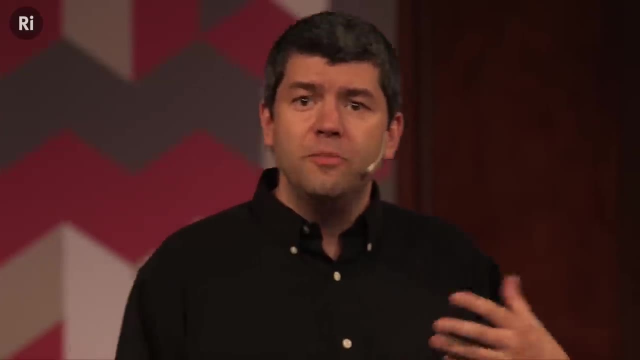 Were Tyrannosaurs predators? Yes, They were both. This is not a big surprise. The vast majority of carnivores alive today are quite happy to hunt food down when they can, but also to pick up a free meal when it's available. 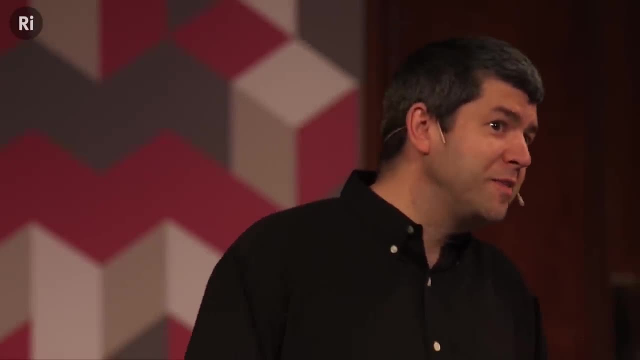 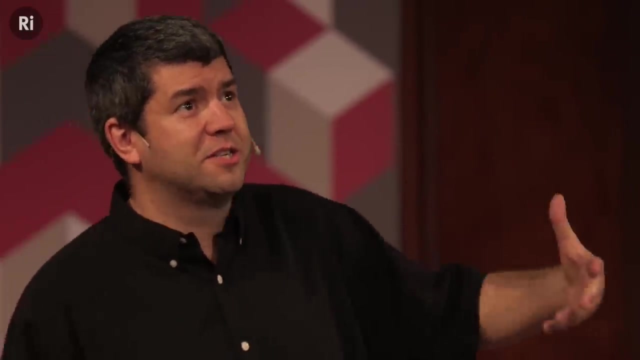 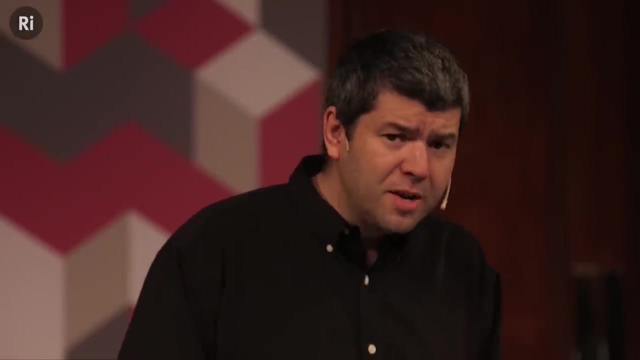 We can begin to put the two together. We're on the spectrum. These things sit. That becomes harder to say, particularly when we've got the situations we've seen where they're actually changing size and shape over time. Maybe some were better adapted for some jobs than perhaps others. 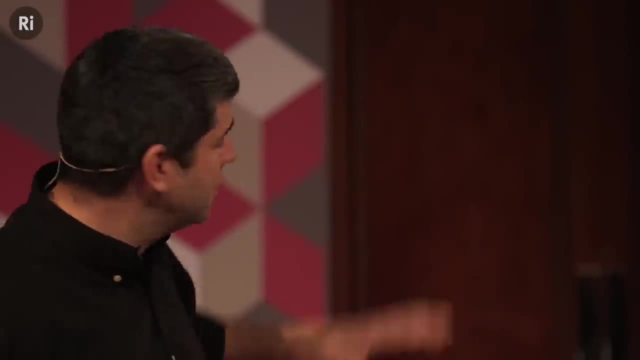 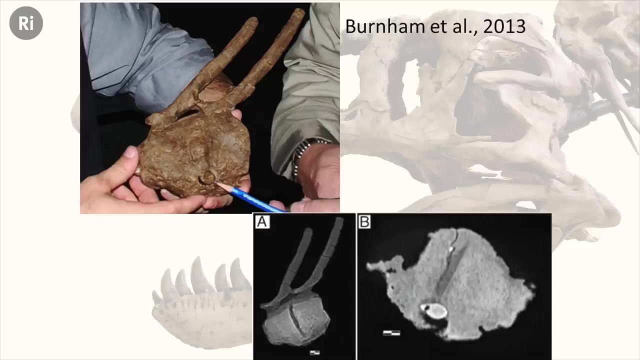 There's also another pattern that's feeding in here. So these three specimens- the one I've mentioned here and the other two, another with a tooth inside it and the other one with a snapped vertebrae- they're all quite young animals, maybe only about half size for hadrosaurs. And in fact there are several evidence of Tyrannosaurs with stomach contents where we actually have the fossilised remains of their last meal. Those are also of juvenile dinosaurs And indeed we also have a Tyrannosaurus coprolite. 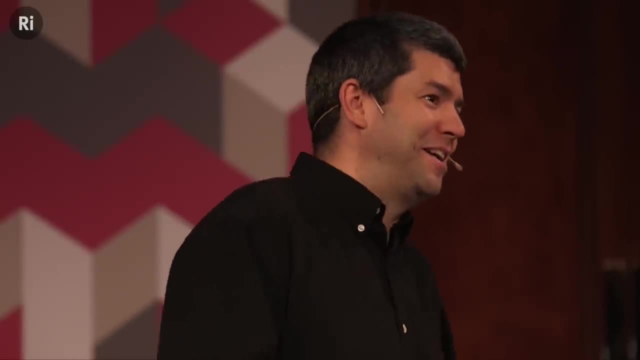 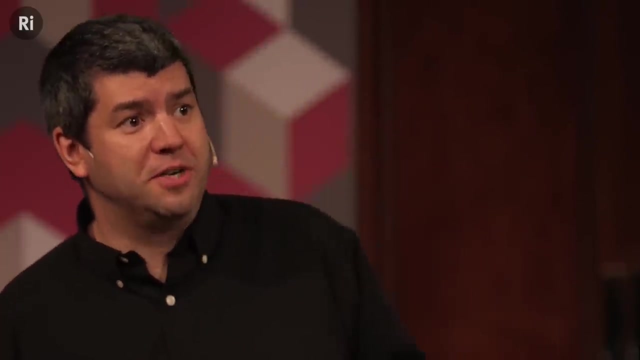 Does everyone know what a coprolite is? Is everyone going to? let me admit it: This is fossilised poo. We have fossil poo for a Tyrannosaurus, and it has bits of bone from baby dinosaurs in it. Now, that's rather interesting that we have five or six of these records. 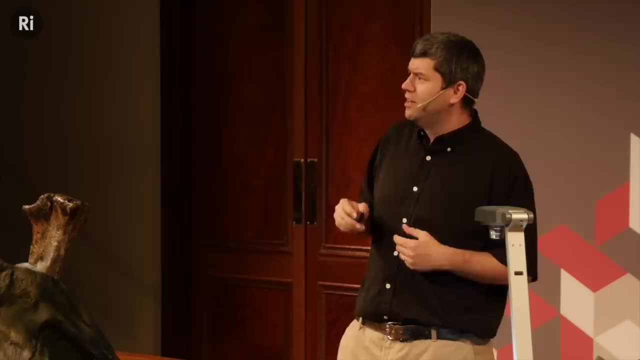 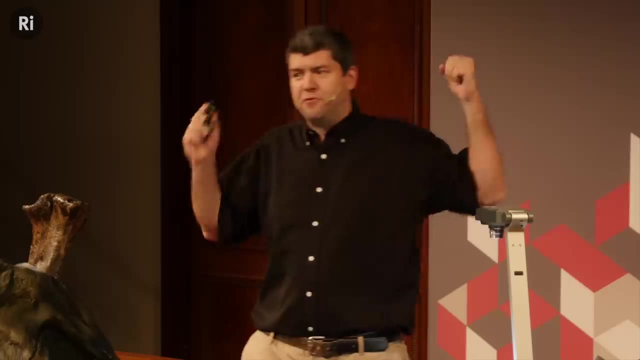 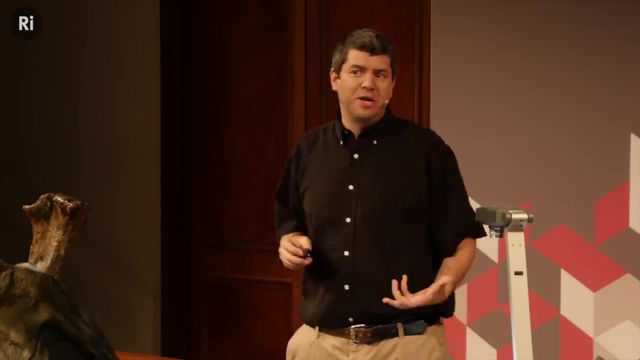 and every single one is a juvenile, because what you always see in documentaries and films is you have to have a full-size adult Tyrannosaurus fighting a big, full-size adult Triceratops, And that's a really bad idea, because a big Triceratops is ways about the same as T rex. 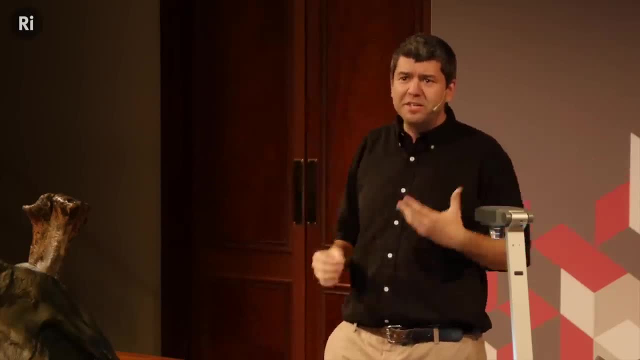 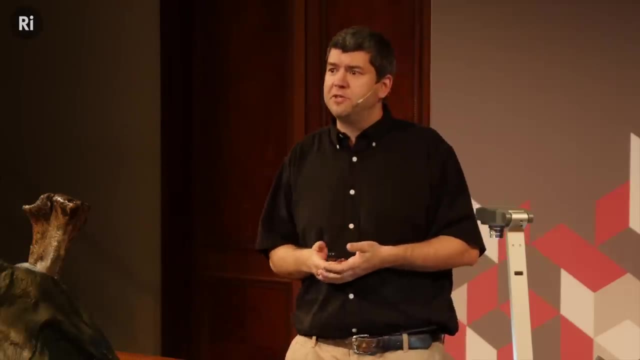 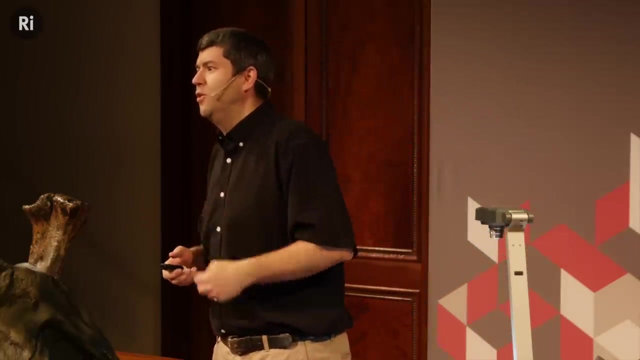 and their horns are about this long. It is an extraordinarily dangerous animal, And anyone who's seen any of the great natural history documentaries, what's the one thing you hear on the voiceover? time over time, The lions target the ill, the old and the young. They don't go after big, healthy, strong adults because any major injury to a carnivore is generally fatal. They will not be able to hunt and they're going to die. So what do they target? Things they can get hold of easily that may not fight back. 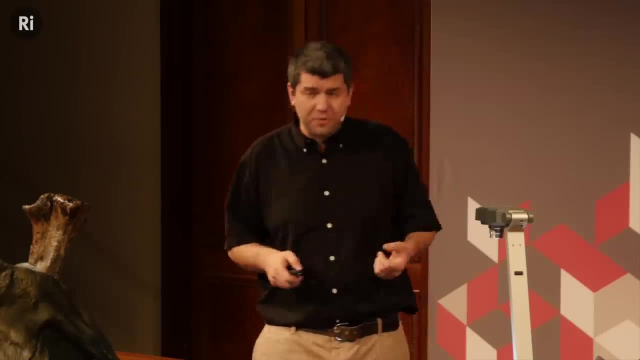 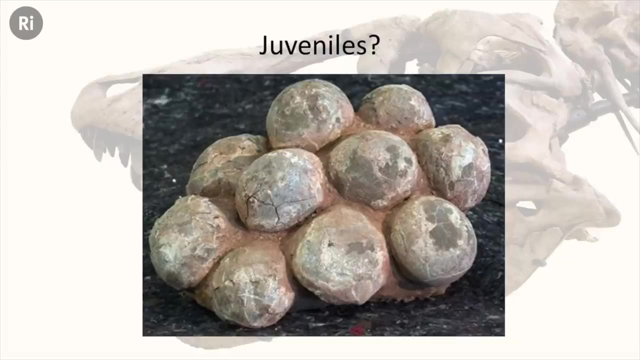 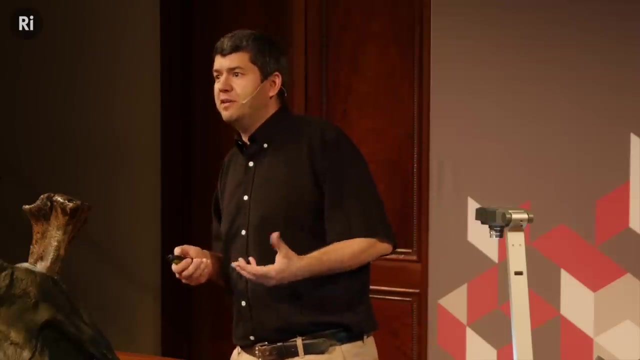 And that leads us to juveniles. What's another big feature we know of dinosaurs? Here is a cluster of dinosaur eggs from central China. They laid lots of eggs. We have very large numbers of juveniles out there. Some of the bigger dinosaurs may have been laying 50-plus eggs at a time. and may have laid multiple nests in a year. Compare that to elephants that have one baby every four to five years, And an even larger dinosaur like a large hadrosaur may have had 100 eggs a year for multiple years in a row. There are an awful lot of small dinosaurs out there to be eaten And it's certainly a better option to try and tackle those than a lovely big adult which is also covered in giant horns or armour. It's much more dangerous. This also fits with what we see in terms of general patterns. 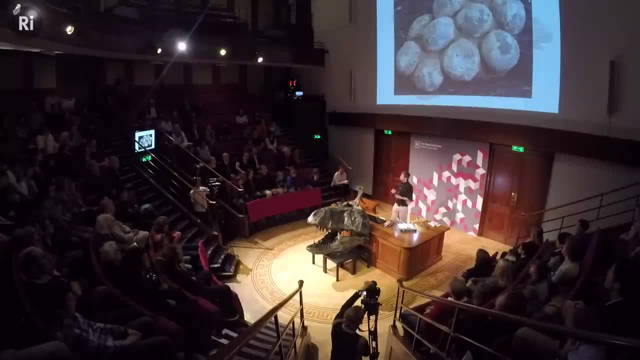 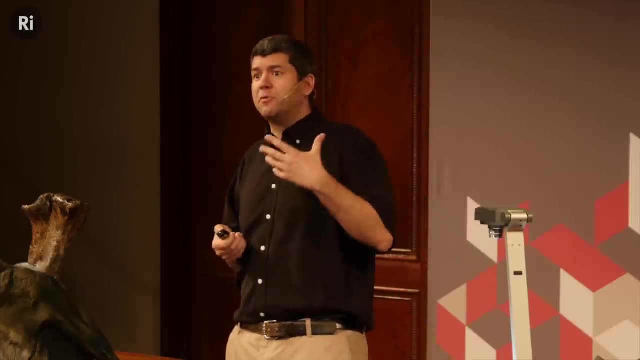 One of the great defences for animals of all sizes and shapes against predators is hanging around together in a cage, so that when they hang around together in groups you're more likely to see some danger coming. And it's very noticeable that we now have dozens of specimens of Triceratops. All the adults are found on their own. We've only ever found juveniles twice, and both times they're in groups, So the adults appear to be solitary. They probably don't have too much to worry about, in the same that a buffalo or rhino generally doesn't worry too much about lions. 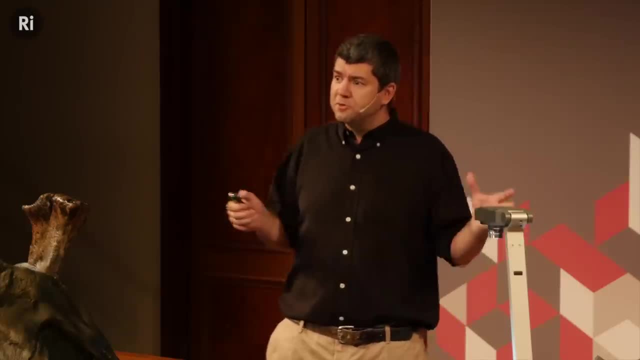 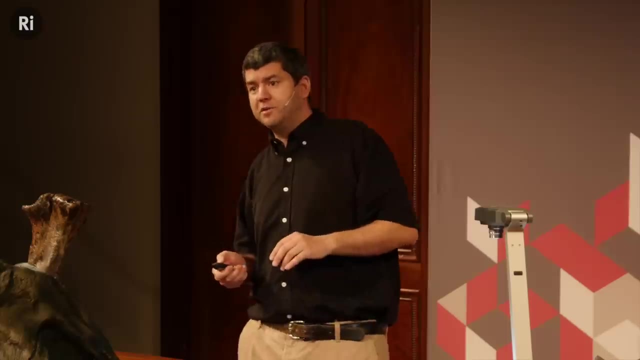 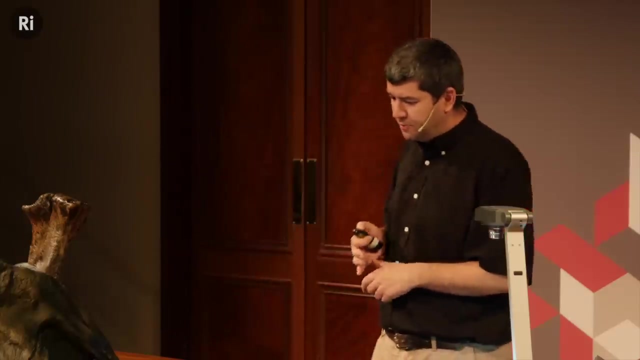 But the juveniles are vulnerable and they're hanging around together. So we see a fundamental shift in the ecology of herbivores as a result of the threat of carnivores. A couple of last things just to bring up about tyrannosaurs before we finish up. 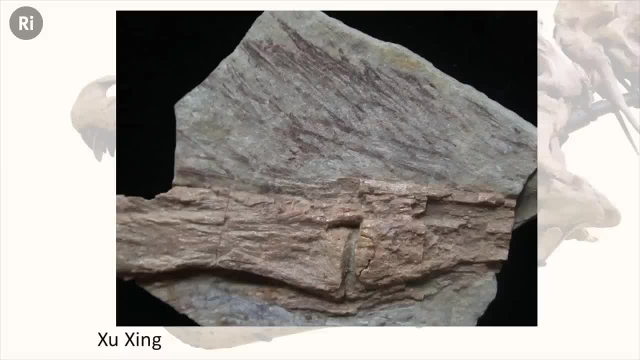 This is part of the tale of DeLong. If you remember, back to the start, DeLong is one of the early tyrannosaurs from China. It's around 150 or so million years old, So from the early part of the tyrannosaurs. it's just a bit of the tale. 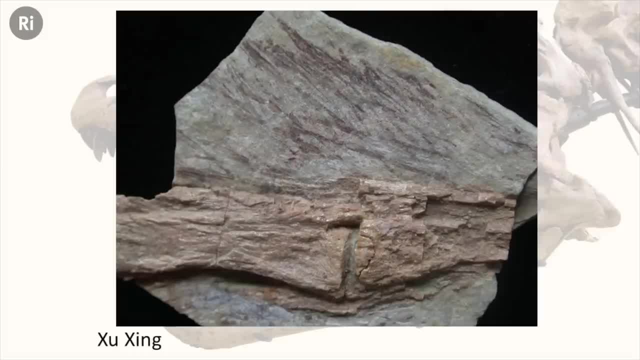 So here's one tailbone, here's the second tailbone, and there's all these lovely little stripey bits on top. Those stripey bits are feathers. Tyrannosaurs had feathers. DeLong has feathers- In fact the nearest relatives of the tyrannosaurs. 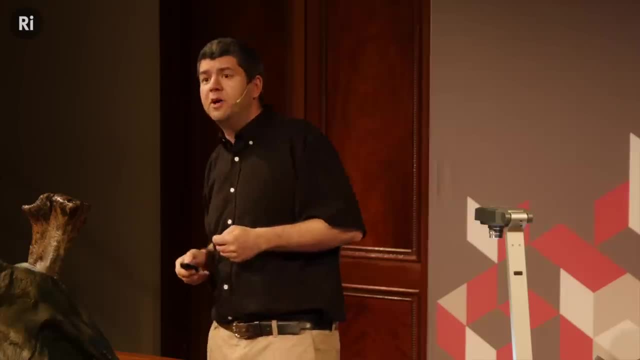 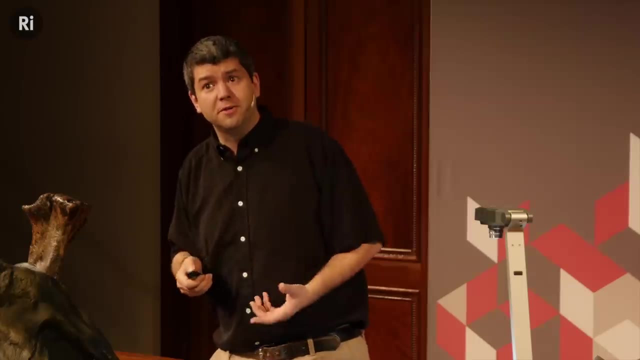 one group called the consignathids and another called the ornithomimosaurs. we know both had feathers and indeed all of their more recent relatives had feathers, up to and including the birds. There's a whole swathe of dinosaurs. 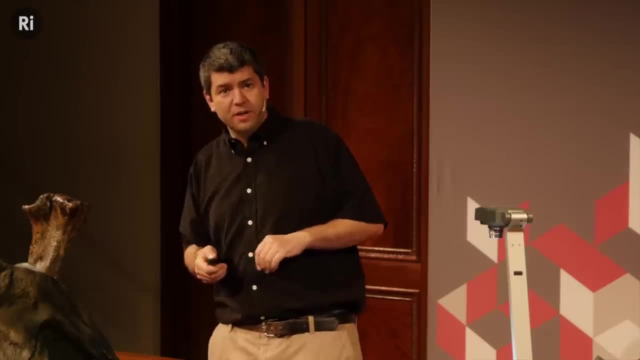 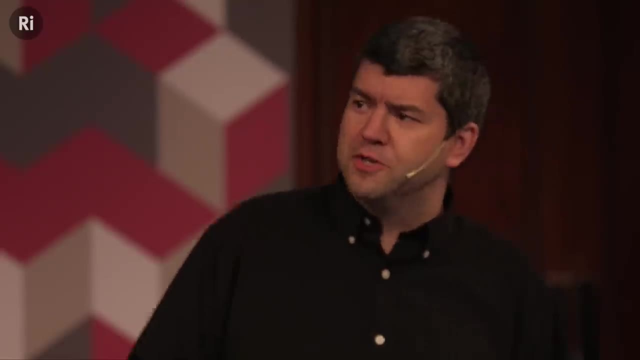 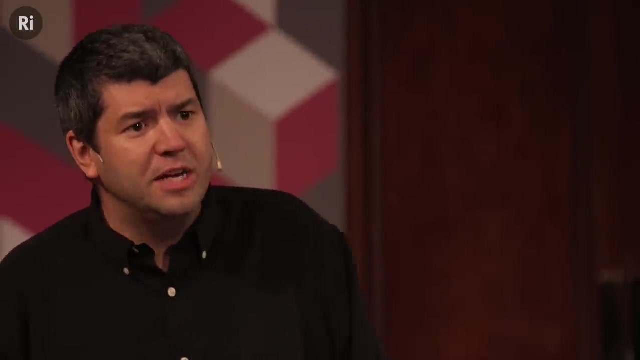 with feathers. One of them is the tyrannosaurs. Now, when this was first found, people were fascinated: Wow, tyrannosaurs may have had feathers And the immediate criticism was okay, but DeLong's like tiny, Like DeLong's two meters or so, It's a really small, little light animal. It lived in quite a cold environment. It needed feathers to keep warm, but T rex wouldn't have feathers. Once you get big, you're going to need to have scales. You're going to need to get rid of those feathers, or you're just going to overheat. 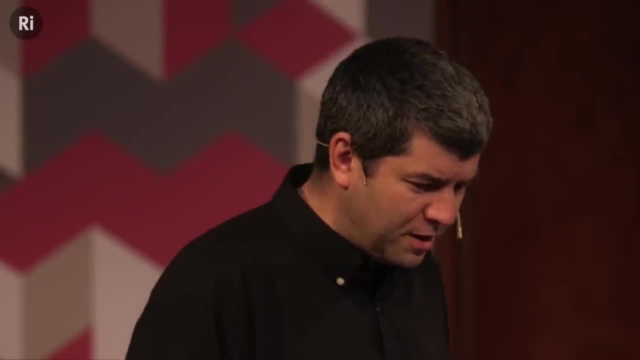 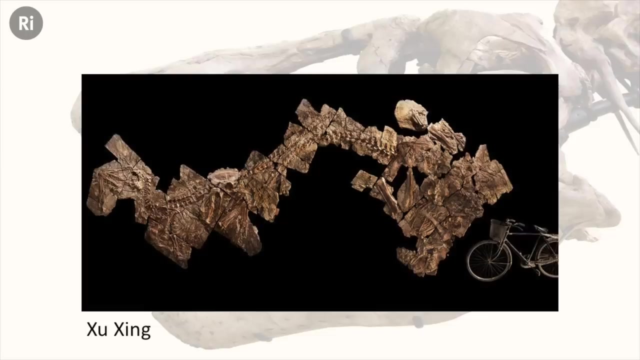 So, okay, maybe DeLong's got feathers, but the other tyrannosaurs don't. Then, a couple of years ago, this turned up. This is Eutyrannus, And it may not be this clear, but Eutyrannus is now known from three specimens. 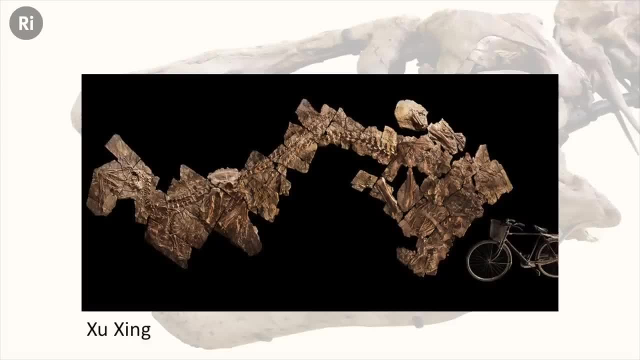 and two of them were found together. So hopefully you can see here is a head and a neck, a back pelvis and a leg and one tail, and then a second tail, pelvis, leg, second leg, body arm and a squashed head, So two lying together. 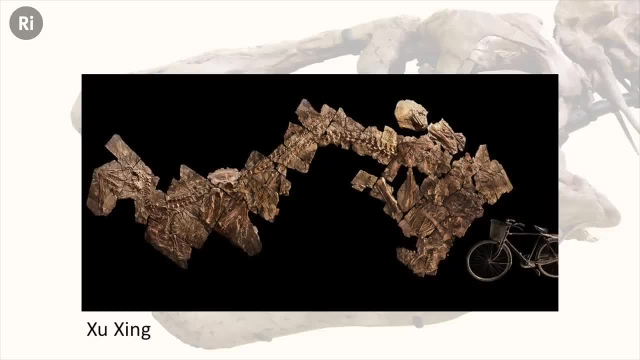 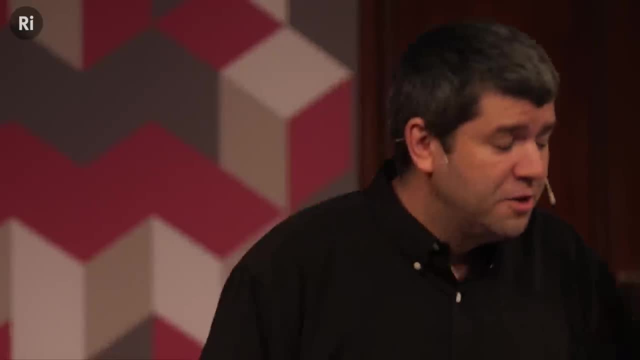 There's a bicycle for scale. You can see how big these are. Eutyrannus is perhaps seven, eight meters from snout to the tip of the tail, maybe a ton. ton and a half. Eutyrannus is covered in feathers from the tip of the snout. 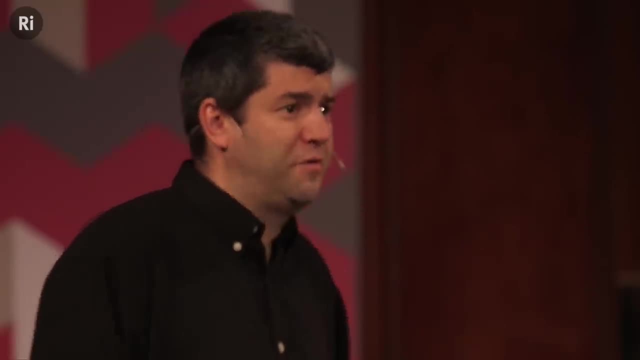 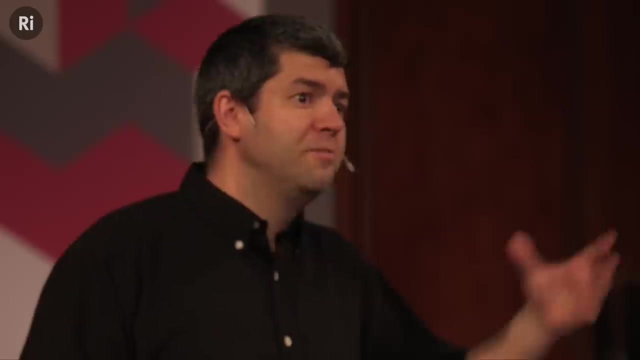 to the tip of the tail to the toes. This is a completely feathered animal. It's also much closer to tyrannosaurus than is DeLong. So we have two different tyrannosaurs with feathers, both a small one and a large one, and separated in a great deal of evolutionary history. 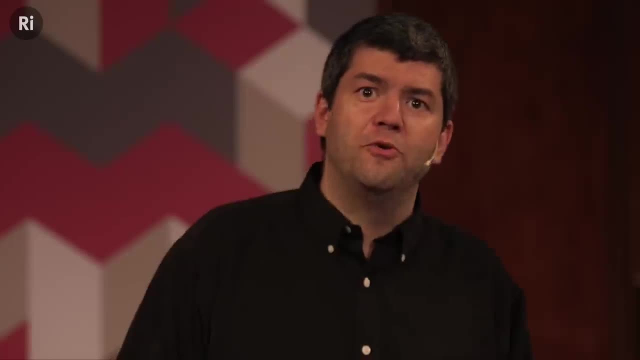 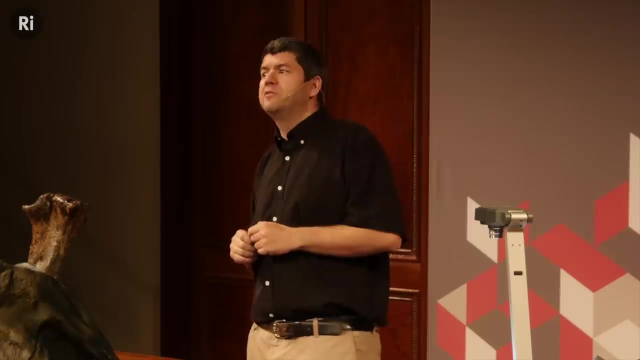 This really strongly suggests that feathers are uniform and present across the tyrannosaurs. We may not have found a feathered tyrannosaurus yet, but it may only be a matter of time, and certainly I'm confident that tyrannosaurus had at least some feathers on it. 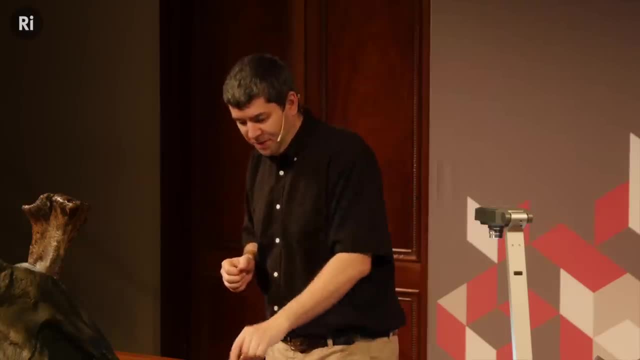 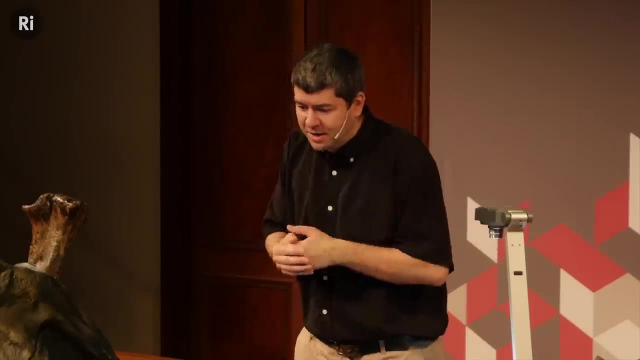 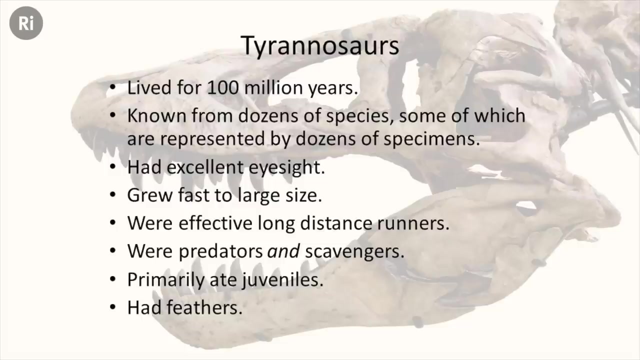 Perhaps not quite a giant chicken, but certainly fluffy. So let's try and summarize all of this up to the best that we can. Tyrannosaurs were around for 100 million years. These were around for a long time. They were on at least three different continents, perhaps as many as five. 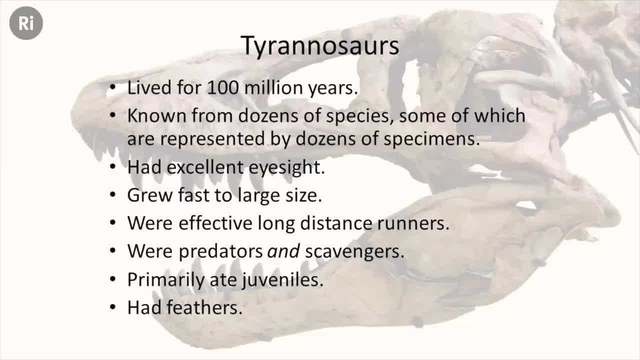 and therefore it wouldn't surprise me if they eventually turned up in Africa as well, and we've got all of the major continents represented. for tyrannosaurs, There's around 30 species known. There are still more coming. There's a new tyrannosaur named only about four weeks ago. 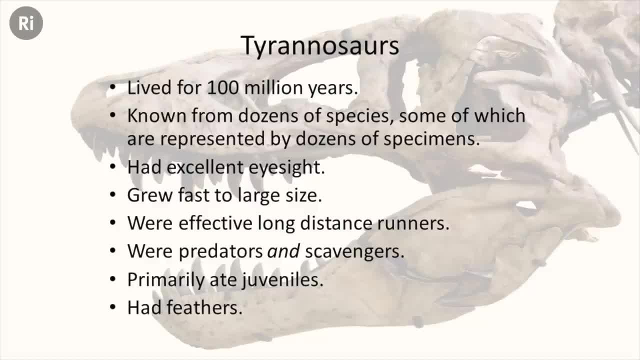 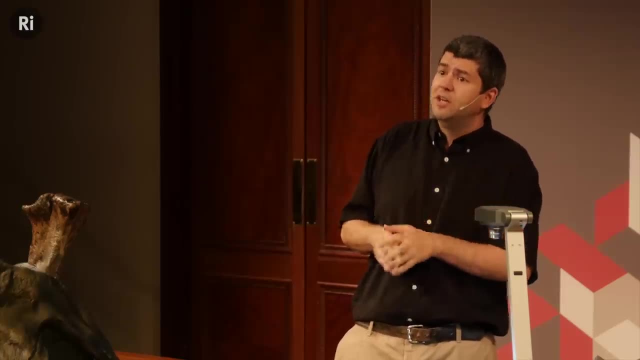 So we're still finding new species, we're still identifying new animals and we're still describing them. But the ones we do have, some are represented by dozens of specimens: T rex around 20.. There's also around 20 of Tarbosaurus in Asia, and about the same for Albertosaurus. 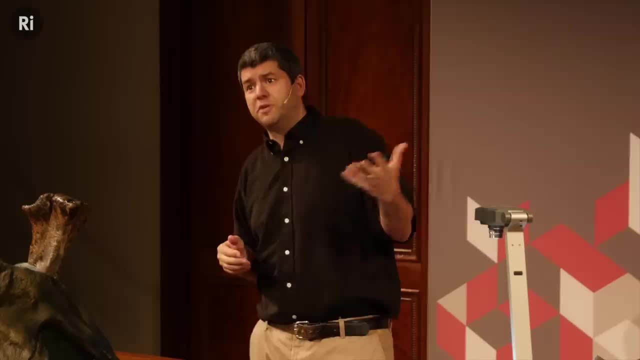 Some of the others are rather less known, but even Guanlong is already known from three complete specimens, including a juvenile. So we actually have a really great knowledge and understanding of these things, their variation, how they grew and how they changed, and indeed they did grow fast to large size. 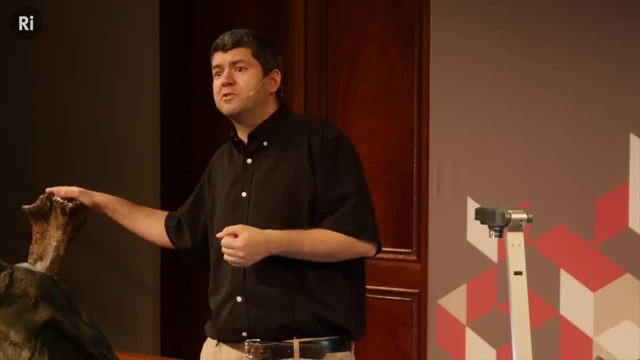 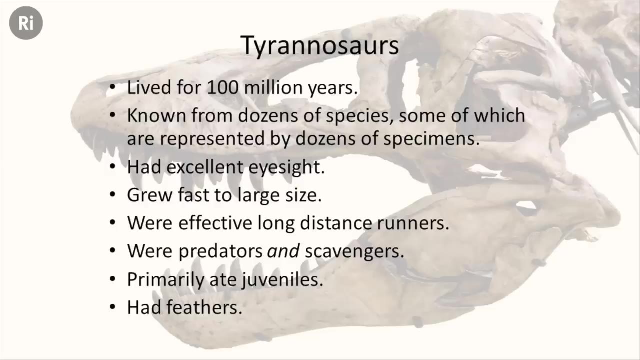 We've seen adaptations in the feet, which means they were probably effective long-distance runners, on top of the fact that they had big, long legs with a long stride length, which would make them quick. We've seen evidence for both predation and scavenging. 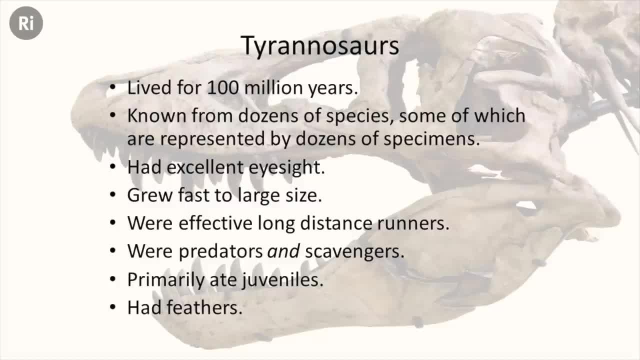 So let's have no more of predator or scavenger. They were predators and scavengers. They had great eyesight. They would have made effective predators. They were probably primarily hunting Jesus. They were probably hunting juveniles when they were, and they were feathered animals.